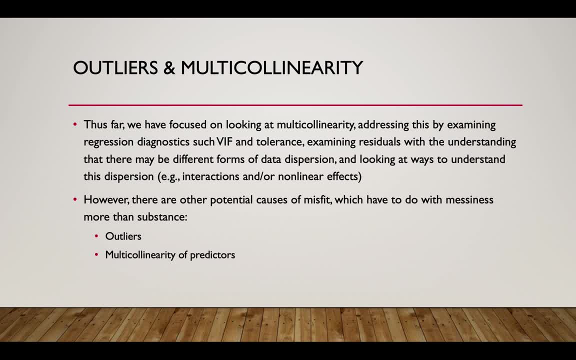 Examining residuals, with the understanding that there might be different forms of data dispersion within those residuals. They may not show homoscedasticity, which is what we're looking for, right, We might see what's called heteroscedasticity, And then we looked at ways to understand this. 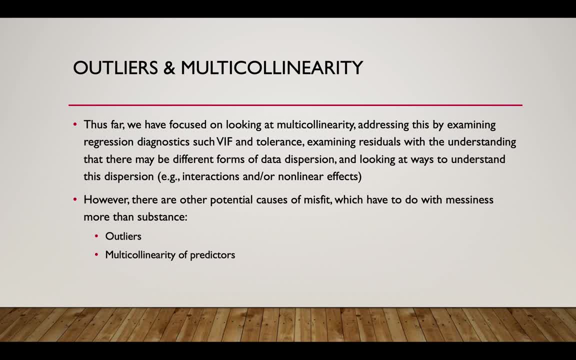 dispersion, either by examining potential interactions, when we see heteroscedasticity, when we see spreads of our residuals or a non-normal distribution of residuals, or trying to fit nonlinear effects with the basic assumption that the effects that we have in our model are almost always nonlinear. 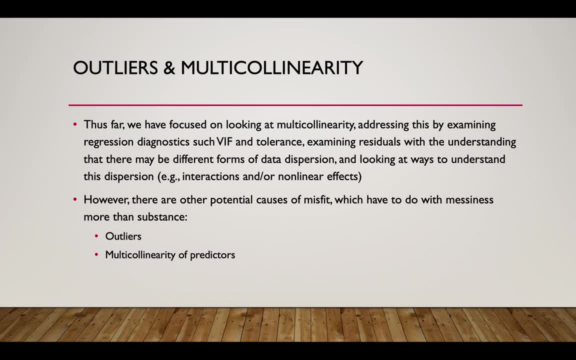 because nothing in nature is truly linear. However, there are other potential causes of model misfit or misspecification which have more to do with- I say messiness, than substance. You know, those first issues having different distributions, or different linear associations or nonlinear effects, that are part of the 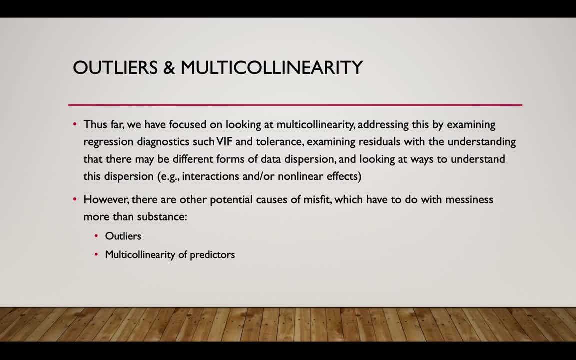 substance of your research question are different than just having problems. We're going to talk about how some of these problems come out. Now, of course, we've talked about multicollinearity and having multicollinear predictors, and this being one of the primary reasons why we center our variables and how we can go about handling 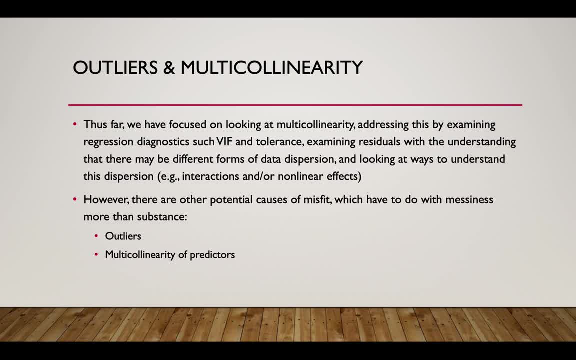 multicollinearity and the different types of multicollinearity. We have not talked very much about outliers. We talked a little bit about graphical descriptions of outliers and how we look at outliers, but we haven't really talked about how we go into testing for outliers. 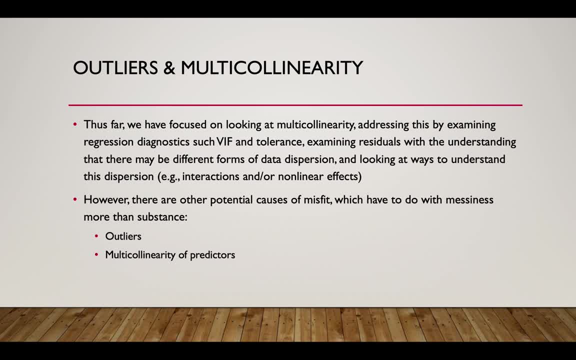 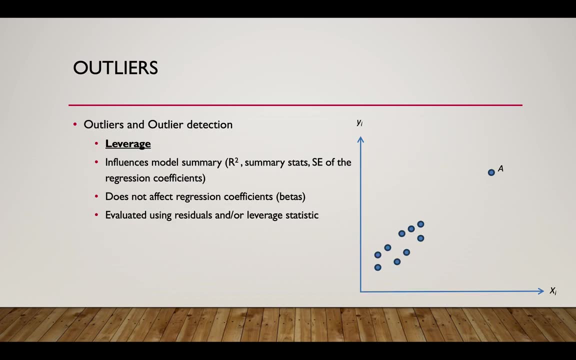 and the ways that we examine our data and come to conclusions about what to do with problematic, um problematic observations or multiple problematic observations. Let's start by talking about leverage. So there are two kind of basic forms of outliers and the first one is leverage. Leverage outliers tend to be something like this: where you 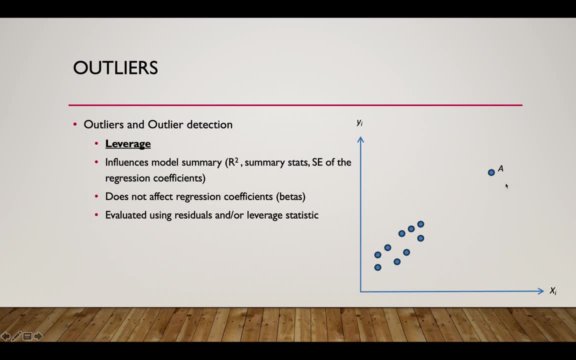 have your nice kind of cluster of linear data and then you have this person way out here. Now, this tends to fall in our linear model and we're going to- you know, we're going to do something here in a little bit- um to to kind of make an example of this. but 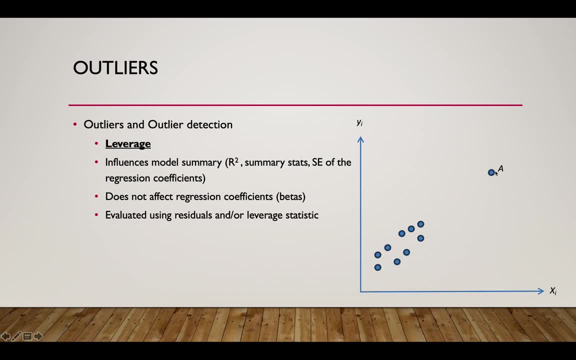 you can see that a observation a, or person a uh, falls in this line, but they're way out here. This actually doesn't change our regression coefficient at all. right, Our regression coefficient would stay roughly the same. What it does do, however, is it inflates. 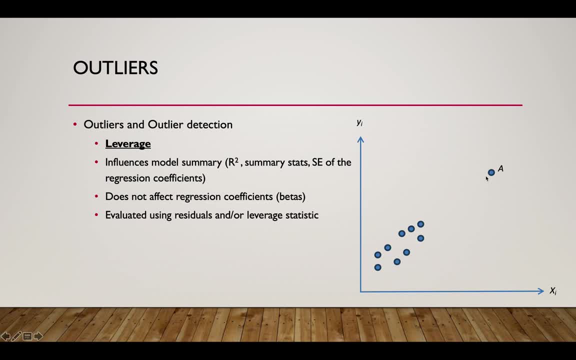 are R-squared for this right. It makes a more perfect, fitting model. It can influence the summary statistics or the standard error of our basic regression coefficients, And we evaluate this using residuals and or the leverage statistic. So we're going to 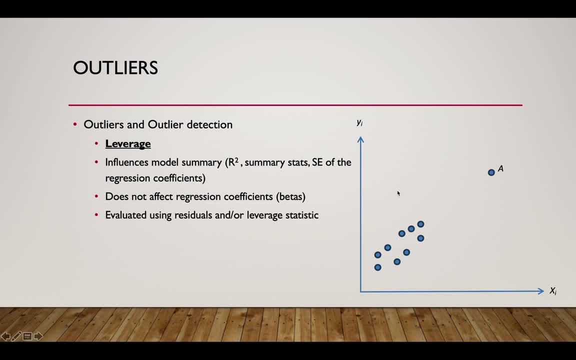 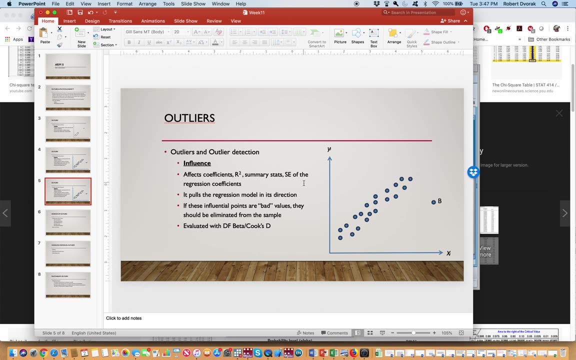 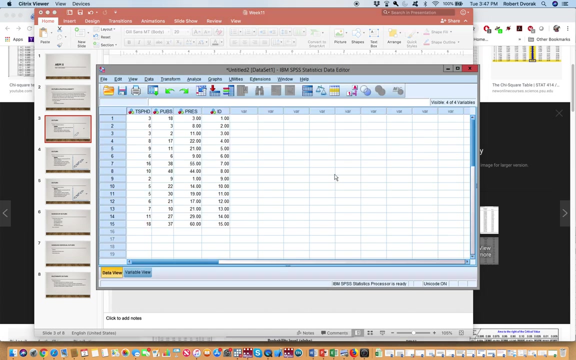 we are going to hop away here for a second And let me do this. Oh yeah, I think I can do that. There we go. All right, we're going to come back. Whoops, let's stay here. We're going to talk about leverage, But let's have a look at some data here. 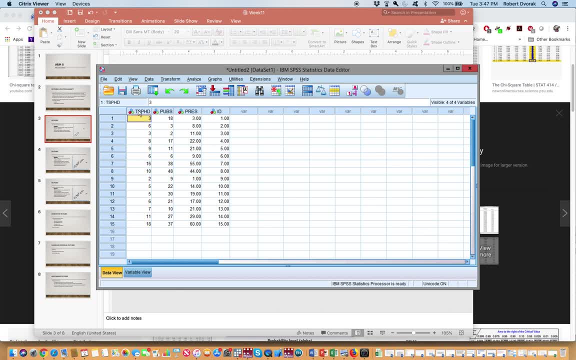 So here we have time. since pH And publications And our this is presentations, We're going to throw another variable in the mix here, And this is just the person's ID. Notice that they correspond to these very this row right here: 1, 2,, 3,, 4,, 5,, 6,, 7,, 8,, 9,, 10,, 11,, 12,, 13,, 14,, 15.. And 1,, 2,, 3,, 4,, 5,, blah, blah, blah, blah, blah, blah. 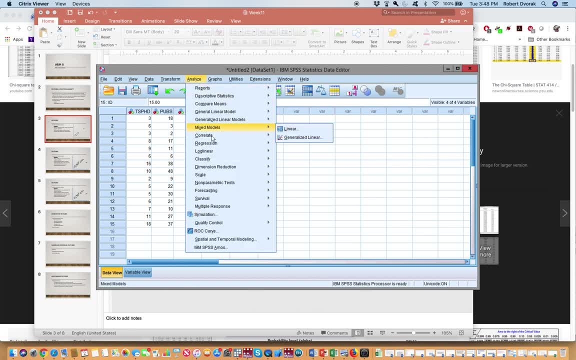 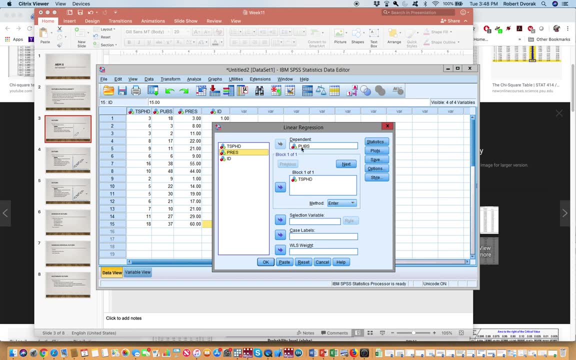 Okay, so let's do something. Let's go analyze regression linear. Let's remove presentations. We're going to look at the, the time since pH, the, as a predictor of publications Statistics. we want model fit R squared descriptives, part and partials, collinearity. 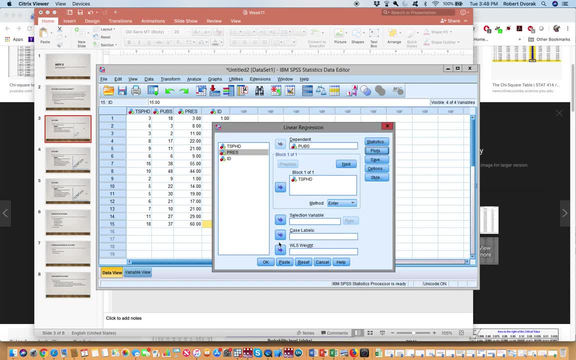 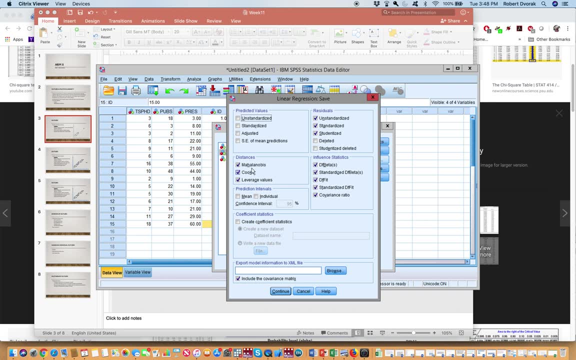 All of the things that we normally request- Plots. we're not going to worry about Save For right now. let's save a whole bunch of stuff. We'll save Mahalanobis distance Cooks. We're going to get leverage values. 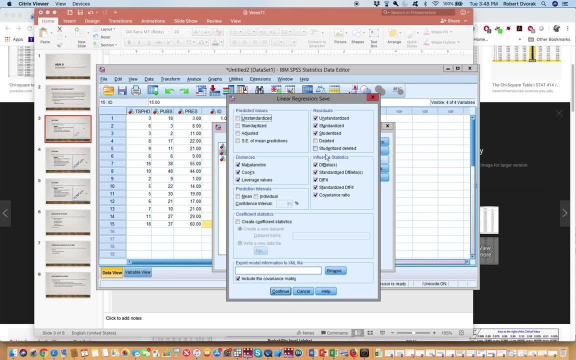 That's what we're talking about right now is leverage. We'll grab some residuals And then we're going to get influenced statistics. We're not going to use these right now, but we're going to come back and compare these after we've run a couple of models. 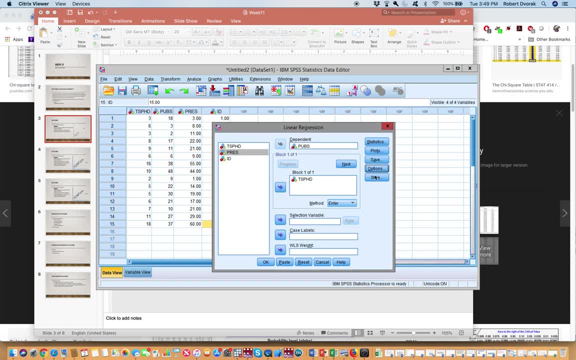 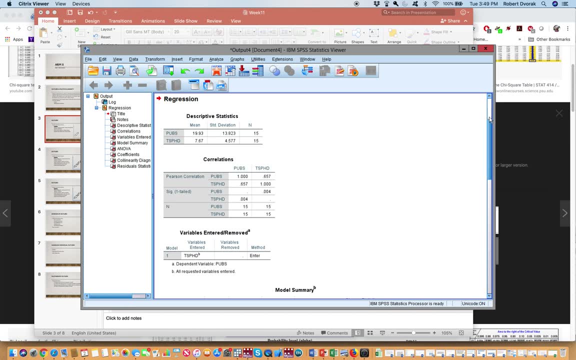 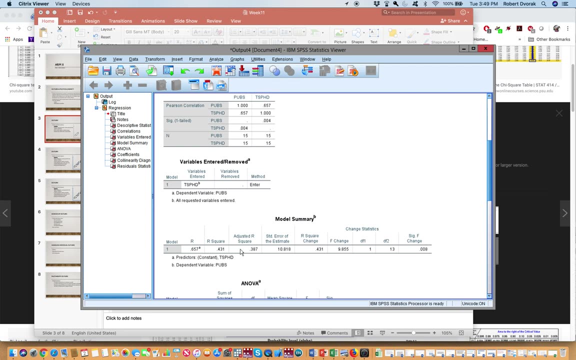 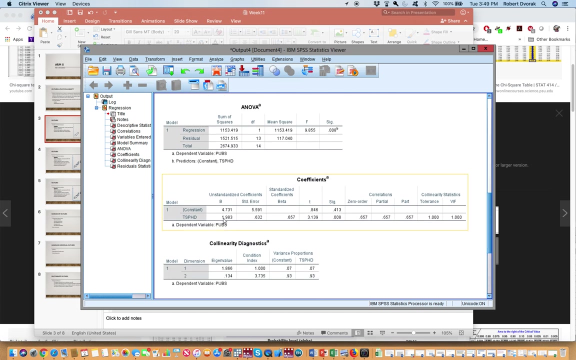 So let's do that. Options. that looks good. Let's analyze that. And Well, so here we are. We have an R squared of .43.. So this is going to be 1.7.. three, we have a regression coefficient of 1.98. it is statistically significant. 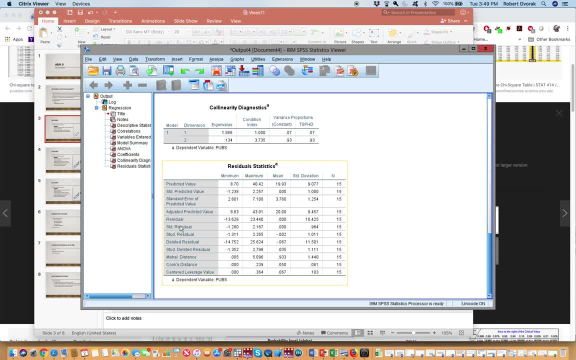 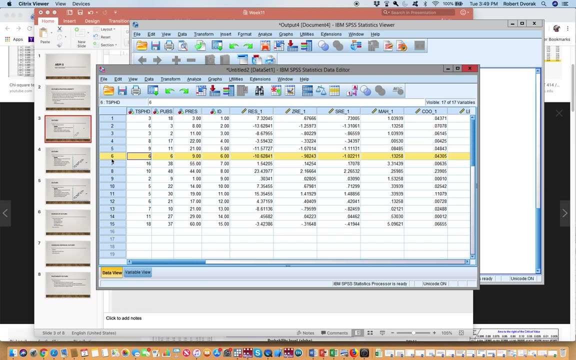 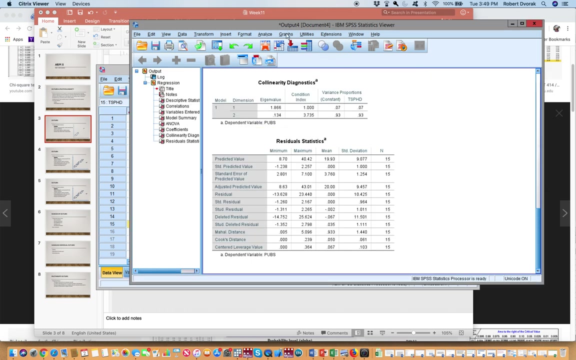 and here are all of the residual statistics, those values that we had requested. we're not going to talk too much about those just yet. what's more important is: let's monkey with this data just a little bit. let's do something. instead of 18 and 37, let's you know what? um, let's go. graph. 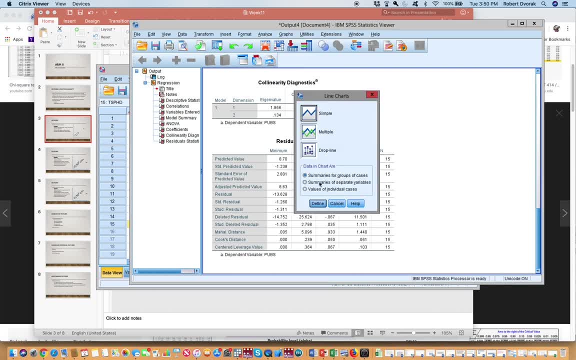 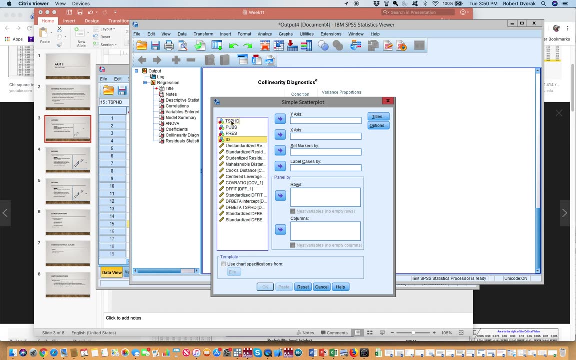 legacy dialogues line. oops, cancel. we don't want a line graph. legacy dialogues- scatter. there we go. we're going to get a simple scatter, um, and we are going to scatter time since phd and on our x-axis and publications on our y-axis. so let's get a simple chart, see. 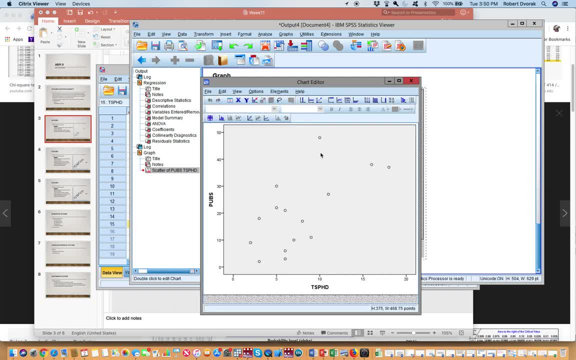 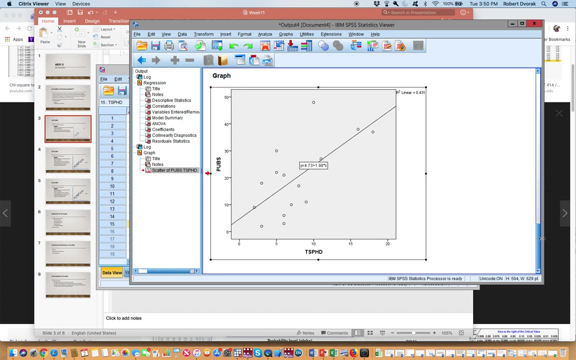 what that looks like. there's our distribution of our data. let's double click on it just for a second and let's just put a simple line in there, okay? so here's our basic regression equation: 4.73 is our intercept, 1.98 times x is our slope, and actually, if we scroll up here, 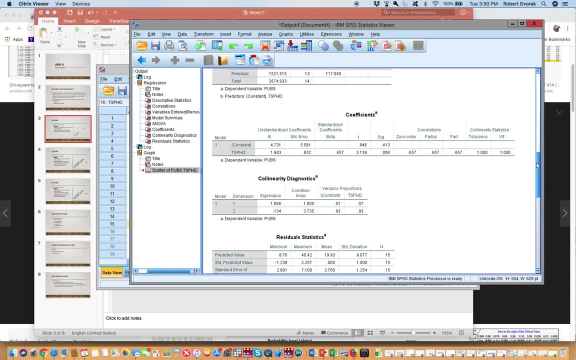 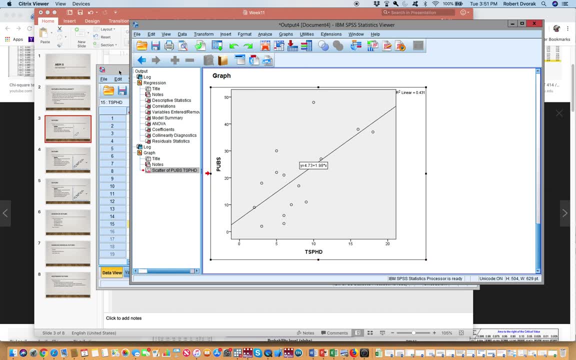 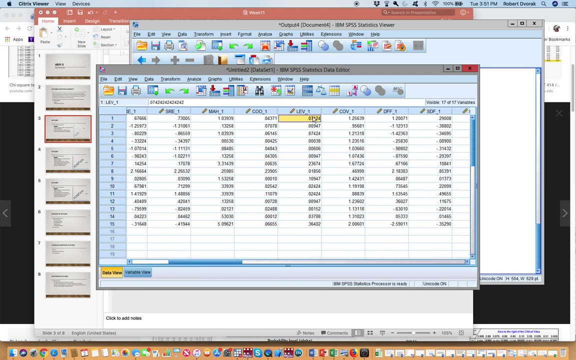 we'll see 4.73, 1.98. those should map onto our regression model and they do. they map on perfectly, and so none of these actually look that bad if we flip over and have a look at just our leverage statistics. that's what we're interested in right now. this is cook's d. here's our leverage. 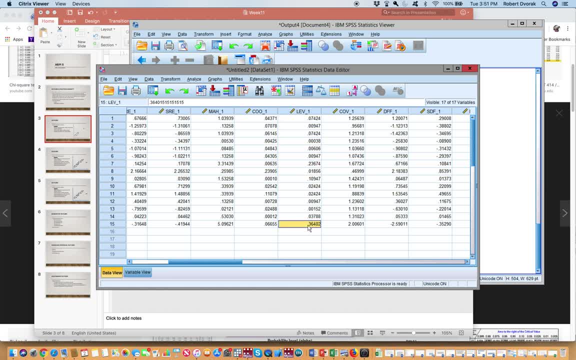 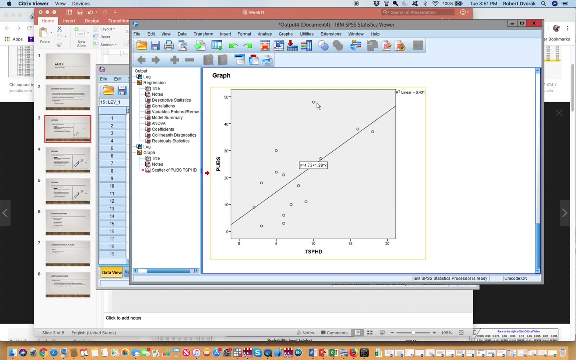 statistics, we do have a couple that look fairly extreme. we have this 0.36 here and 0.23 here. so if you look at our graph, those are these two right here. this is not causing undue leverage and you can kind of assume leverage is the dots that fall or the data points that fall, kind of. 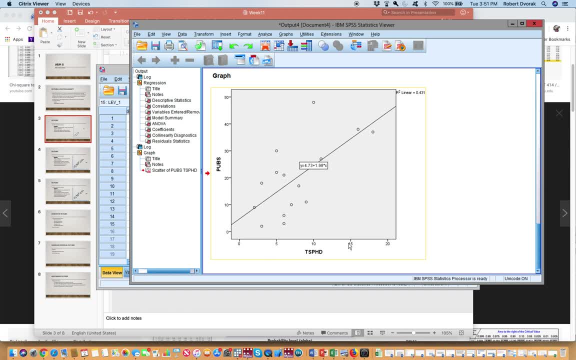 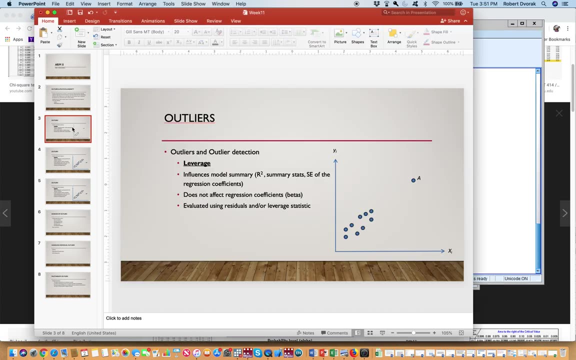 closely together along the x-axis and all of these do. and then you have some x-axis outliers here. now they're not outliers as far as the model goes, they're just extreme values on the x-axis and about when we're talking about leverage. so let's try and do something. let's. 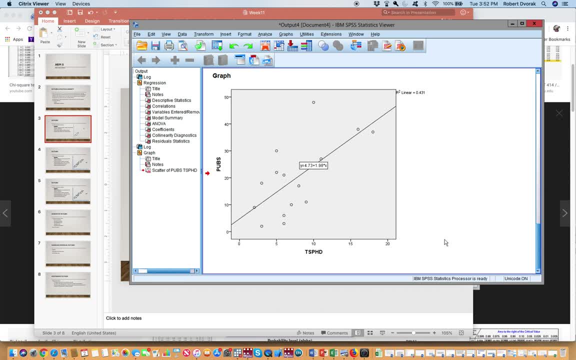 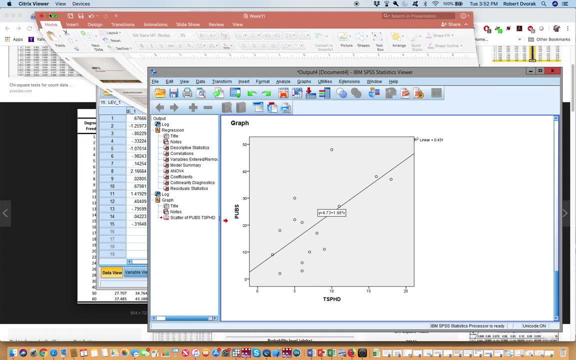 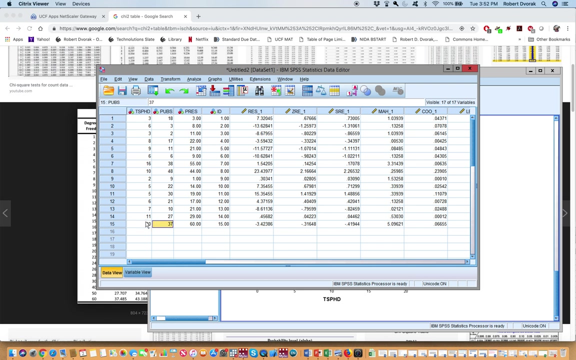 let's assume that we had 30 out here, and if we were at 30, then our dot should be right around. I don't know. 50, let's call it 50. so let's go over here. where is mine there? it is all right. so we are gonna say 30 and 50. that is a big jump here. 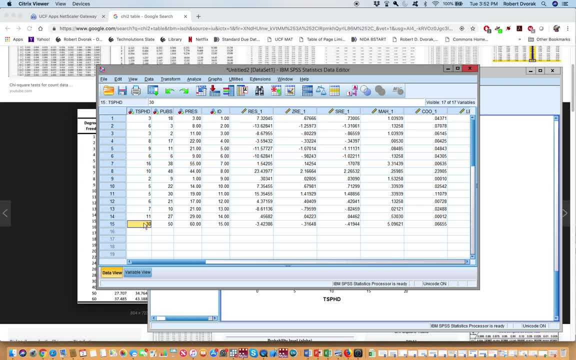 right, so we change it to 50 publications. right, so we change it to 50 publications. right, so we change it to 50 publications. 30 years since PhD. now we're expecting 30 years since PhD. now we're expecting 30 years since PhD. now we're expecting this line to be like roughly the same. 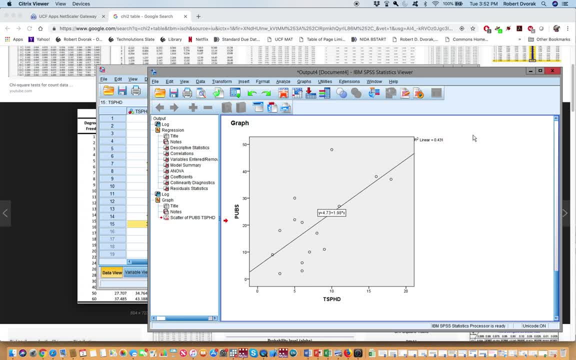 this line to be like roughly the same. this line to be like roughly the same. remember, our slope is 1.98. we'll see if, remember, our slope is 1.98. we'll see if, remember, our slope is 1.98. we'll see if it changes a lot, but we're hoping to put 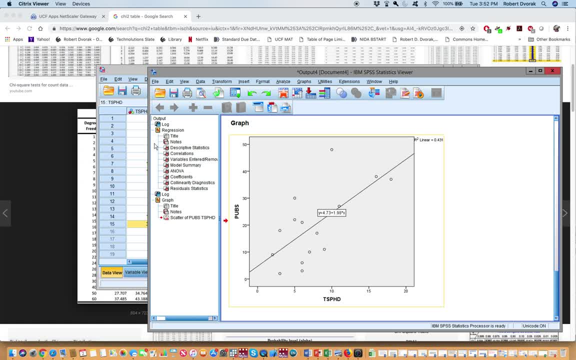 it changes a lot, but we're hoping to put. it changes a lot, but we're hoping to put a dot way out here. right, let's do that a dot way out here. right, let's do that. a dot way out here. right, let's do that. and let's see what happens to our, our. 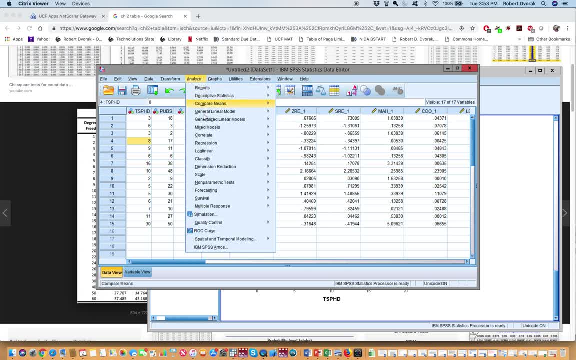 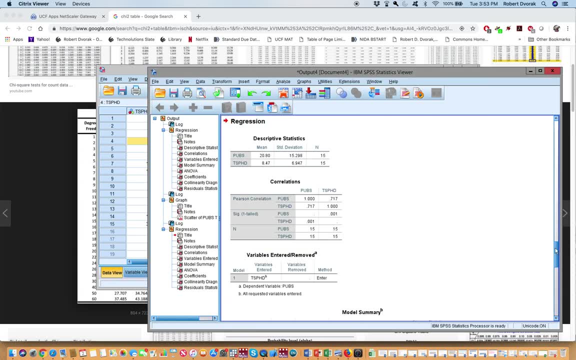 and let's see what happens to our, our and let's see what happens to our our leverage and our statistics now analyze leverage. and our statistics now analyze regression linear. we're gonna run regression linear. we're gonna run regression linear. we're gonna run everything exactly the same now in. 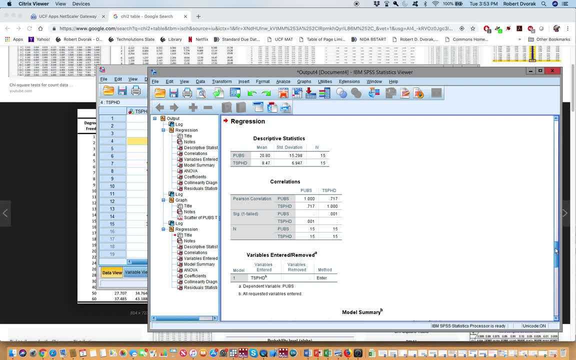 everything exactly the same now in everything exactly the same now in something that we expect to have, something that we expect to have, something that we expect to have significant leverage effects. we are significant leverage effects. we are significant leverage effects. we are expecting that our slope coefficients expecting that our slope coefficients 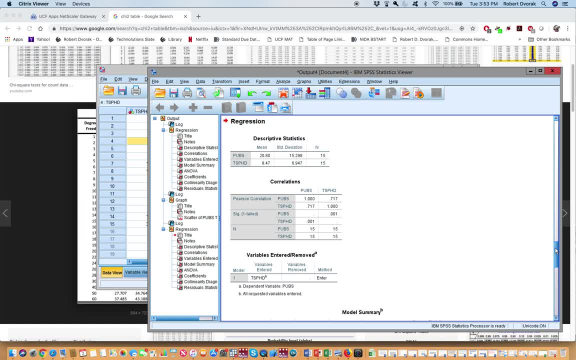 expecting that our slope coefficients will not change or should not change, will not change, or should not change, will not change or should not change. much so. we had 1.98 before, but that our much so we had 1.98 before, but that our much so. we had 1.98 before, but that our R squared should change dramatically. so 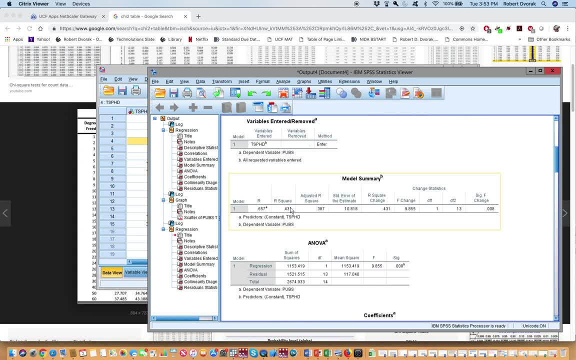 R squared should change dramatically. so R squared should change dramatically. so before we had an R squared of 0.43, let's before we had an R squared of 0.43, let's before we had an R squared of 0.43. let's see what our new R squared is by: 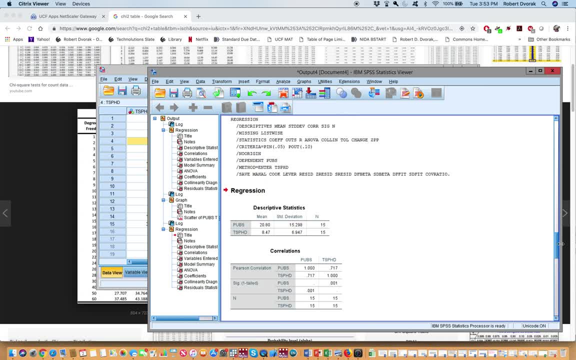 see what our new R squared is by see what our new R squared is by putting something along that line, just putting something along that line, just putting something along that line, just out here further. here's our new model, out here further. here's our new model, out here further. here's our new model: R squared jumps up to 0.51. that is quite. 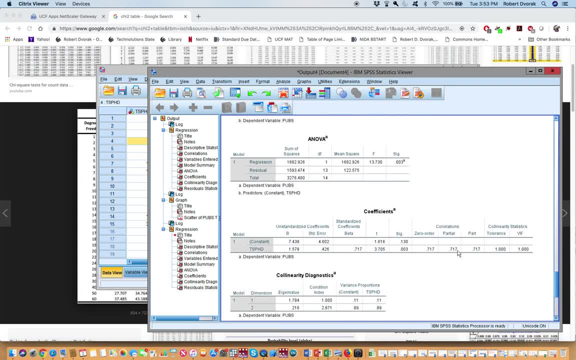 R squared jumps up to 0.51. that is quite. R squared jumps up to 0.51. that is quite a bit higher. that's almost 10% more, a bit higher. that's almost 10% more, a bit higher. that's almost 10% more. variance explained: this is 1.578, not 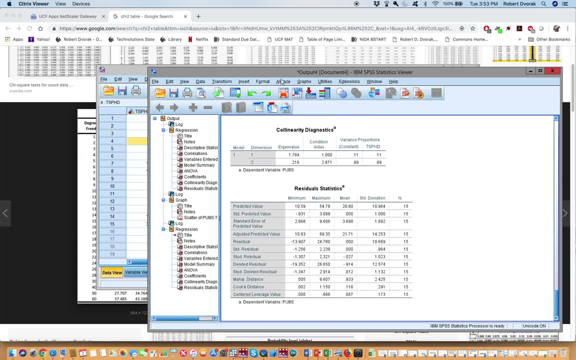 variance explained: this is 1.578. not variance explained: this is 1.578. not ideal: I mean it did drop my guess. is I ideal? I mean it did drop my guess is I ideal? I mean it did drop my guess is. I did a pretty bad job of putting that. 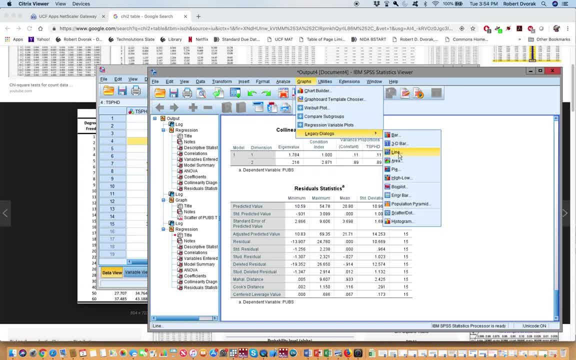 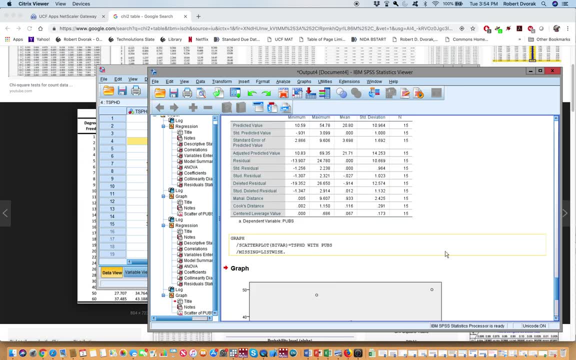 did a pretty bad job of putting that. did a pretty bad job of putting that. that on there. let's have a look and see that on there. let's have a look and see that on there. let's have a look and see where that line fits. um, oh yeah, so you. 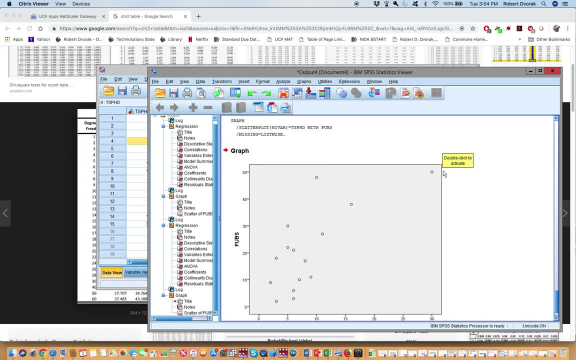 where that line fits: um, oh yeah. so you where that line fits? um, oh yeah. so you can see, I should have actually made this. can see, I should have actually made this. can see, I should have actually made this about 60. so let's do that, let's come. 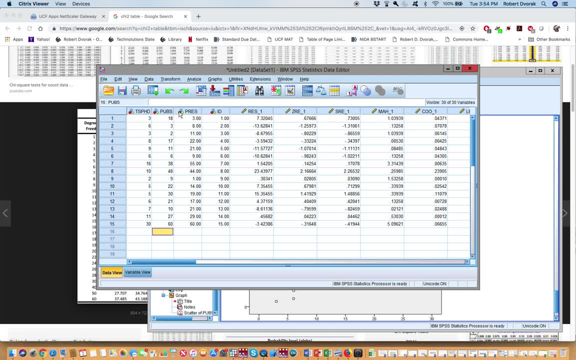 about 60, so let's do that. let's come about 60, so let's do that. let's come back over here. let's change this to 60. back over here. let's change this to 60. back over here. let's change this to 60. that should put it closer to that line. 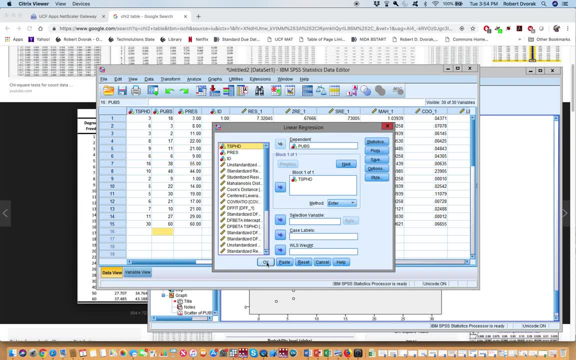 that should put it closer to that line. that should put it closer to that line. analyze regression linear. run it all. the analyze regression linear. run it all. the analyze regression linear, run it all. the same r-squared should have gone up more. same r-squared should have gone up more. 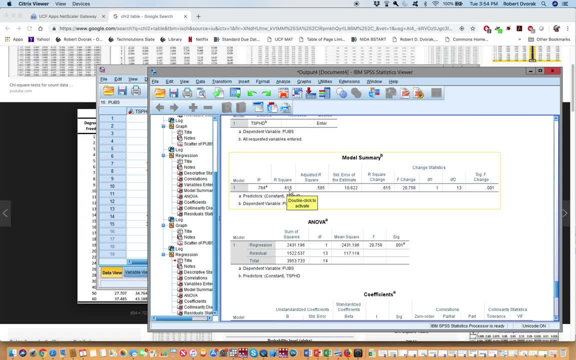 same r-squared should have gone up more. I'm guessing, oh, now it went way up. so I'm guessing, oh, now it went way up. so I'm guessing, oh, now it went way up. so now it's point six, one, five or point. now it's point six, one, five or point. 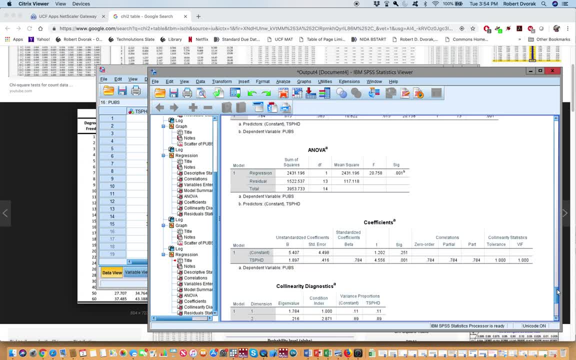 now it's point six one, five, or point six two versus point four three. that's six, two versus point four three. that's six, two versus point four three. that's almost 20% more our slope point eight, almost 20% more our slope point eight. 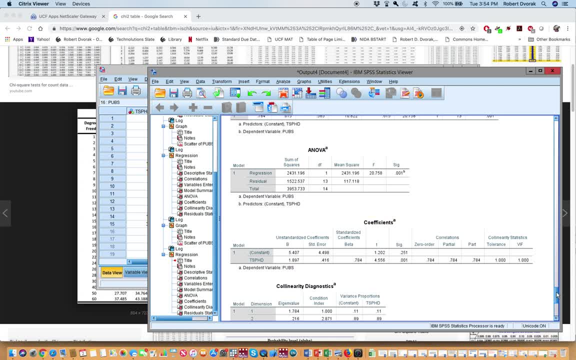 almost 20% more. our slope point eight, nine, seven, that's pretty close. point nine seven, that's pretty close point nine seven, that's pretty close point nine eight was what it was before. and if nine eight was what it was before, and if nine eight was what it was before, and if we graph this out again: graphs legacy: 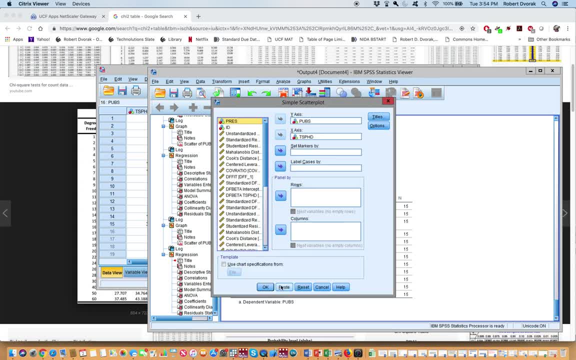 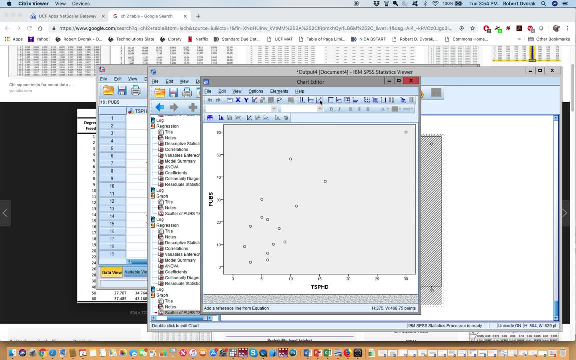 we graph this out again: graphs legacy. we graph this out again: graphs legacy: dialog scatter- let's just have a look. dialog scatter- let's just have a look. dialog scatter- let's just have a look here. yeah right, let's, let's plot our here. yeah right, let's, let's plot our. 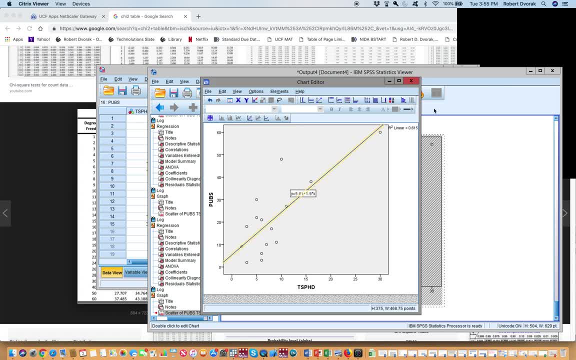 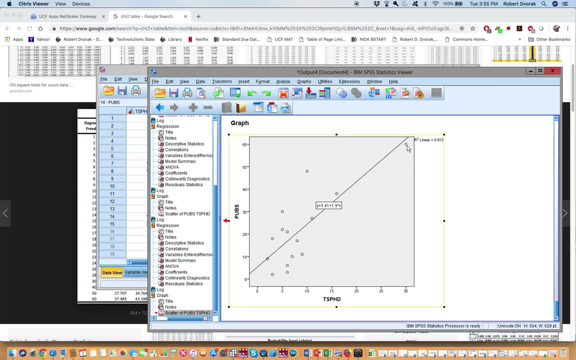 here. yeah right, let's. let's plot our line here, see how it looks. plot our line here, see how it looks. plot our line here, see how it looks. plot our line there. that line looks pretty good. line there, that line looks pretty good. line there, that line looks pretty good. but you can see that this thing here is. 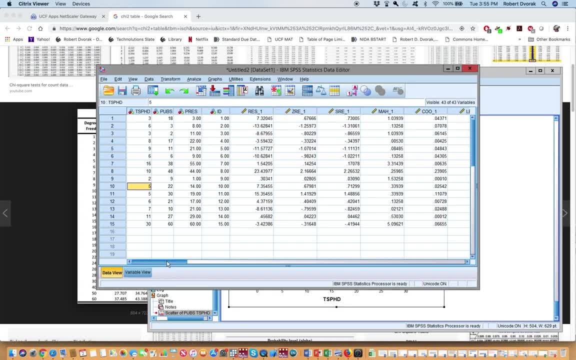 but you can see that this thing here is, but you can see that this thing here is way out here. let's go in and let's have way out here. let's go in and let's have way out here. let's go in and let's have a look at something. so, before our, in our, 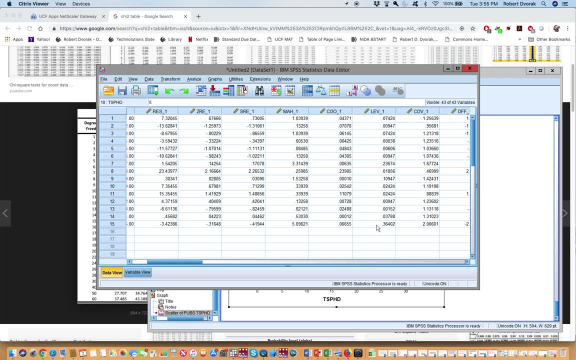 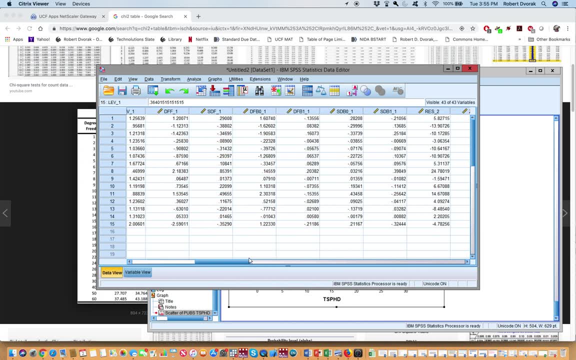 a look at something. so before our, in our, a look at something. so before our, in our very first model, we had a leverage of very first model. we had a leverage of very first model. we had a leverage of point three, six. however, now in our, point three, six. however, now in our, 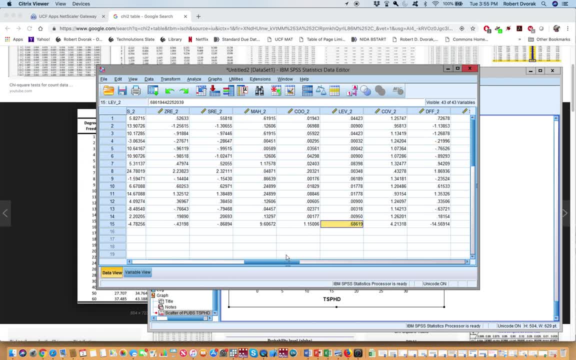 point three, six. however, now in our second model, our leverage was point six. second model, our leverage was point six. second model, our leverage was point six, eight. that's a lot higher in our last eight. that's a lot higher in our last eight. that's a lot higher in our last model. leverage: point six, eight again. 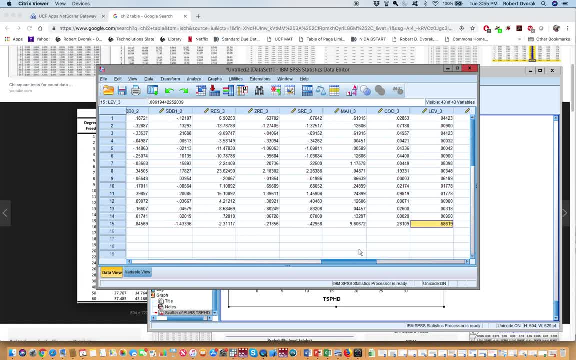 model leverage point six: eight again. model leverage point six: eight again, that's that's. that's not so bad, I'm just kidding, it's actually not so bad, I'm just kidding, it's actually not so bad, I'm just kidding, it's actually really bad. and so it's not exerting. 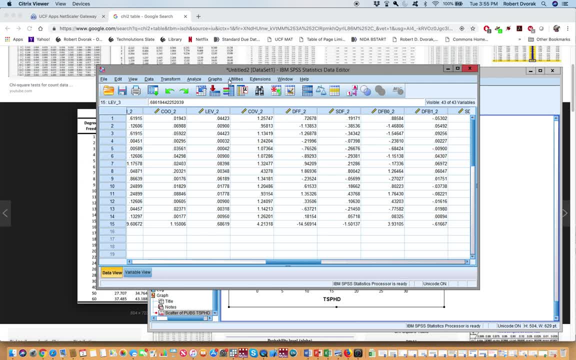 really bad and so it's not exerting really bad and so it's not exerting actually a lot more leverage than our, actually a lot more leverage than our, actually a lot more leverage than our. second model was a way to kind of look. second model was a way to kind of look. 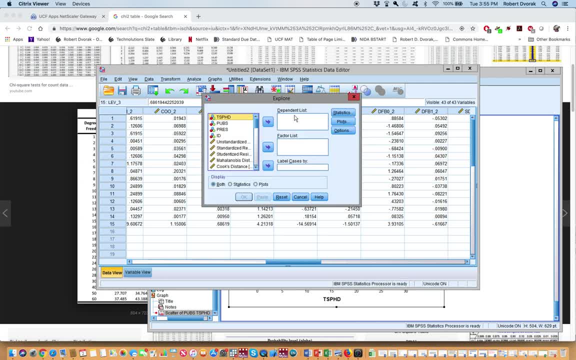 second model was a way to kind of look at this is we can go analyze at. this is we can go analyze at. this is we can go analyze descriptives explore and let's just put descriptives explore and let's just put descriptives explore and let's just put leverage over here. let's put both of. 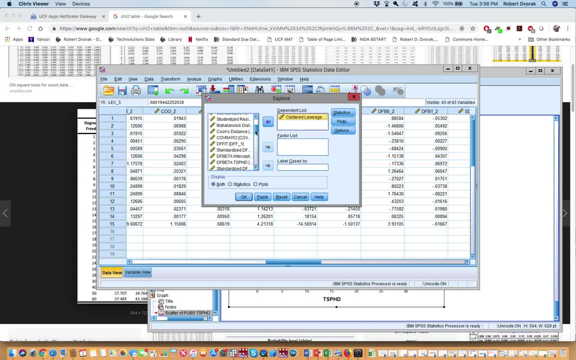 leverage over here. let's put both of leverage over here. let's put both of the leverages that we've done here. so the leverages that we've done here, so the leverages that we've done here. so let's start with this leverage value and 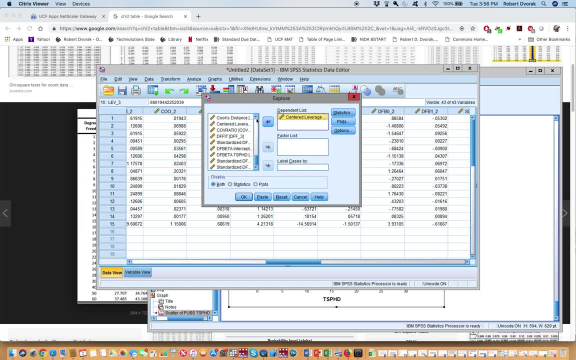 let's start with this leverage value, and let's start with this leverage value and then let's come get the leverage from then. let's come get the leverage from then let's come get the leverage from the last one that we just did and get the last one that we just did and get. 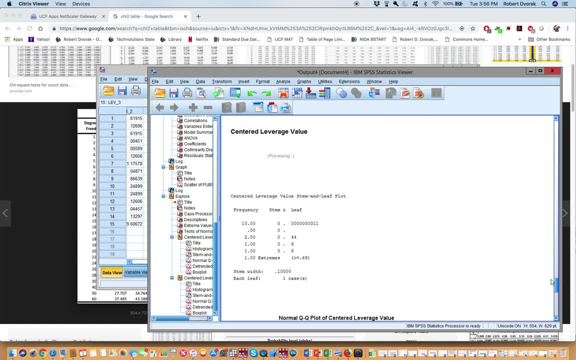 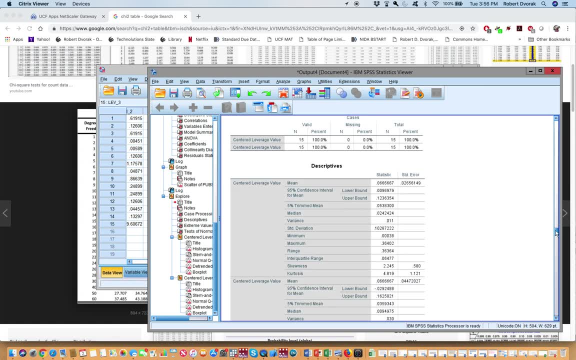 the last one that we just did and get okay, and let's have a look. oh sorry, okay. and let's have a look: oh sorry, okay. and let's have a look: oh sorry, slow, okay. here's where we ended all. slow, okay. here's where we ended all. 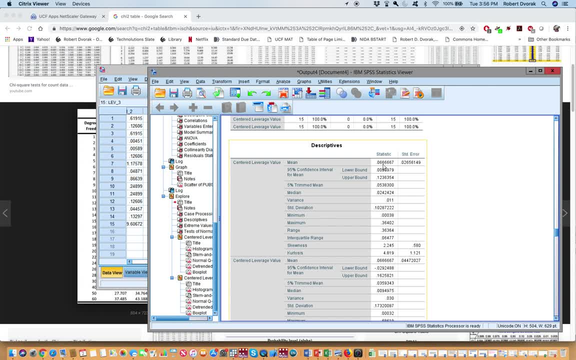 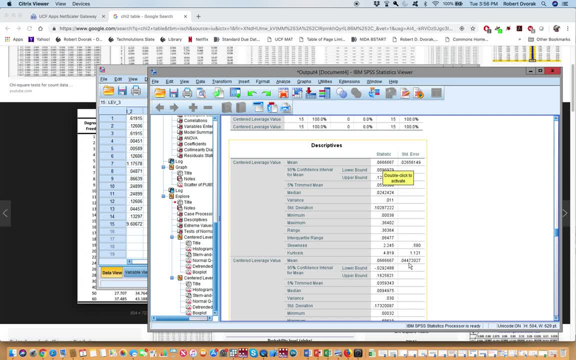 again our centered leverage here: 0.06. again our centered leverage here: 0.06. standard error is 0.02. here our standard standard error is 0.02. here our standard standard error is 0.02. here our standard error is 0.044. so with this standard, 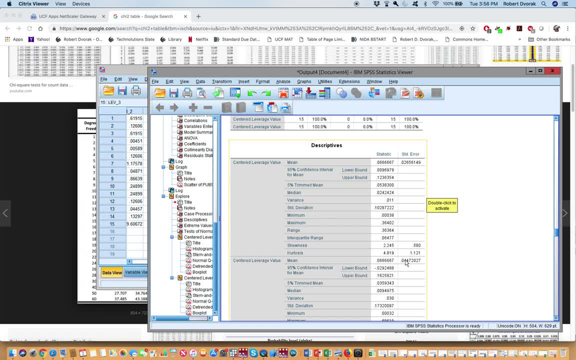 error is 0.044. so with this standard error is 0.044. so with this standard error, we can divide any value, any error. we can divide any value, any error. we can divide any value, any leverage value that we have and that will leverage value that we have and that will. 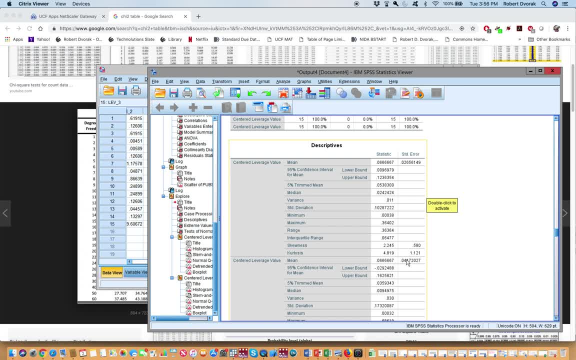 leverage value that we have and that will give us the number of the? the z-scores. give us the number of the the z-scores. give us the number of the the z-scores. away from the mean that we are and so. away from the mean that we are and so. 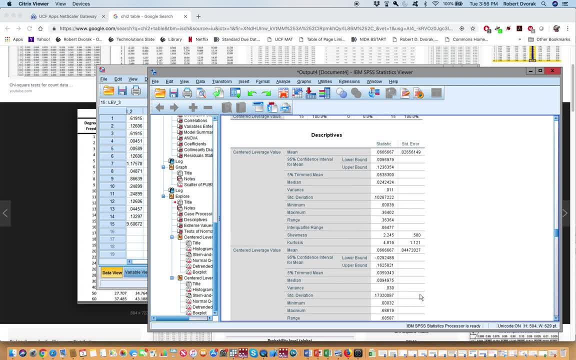 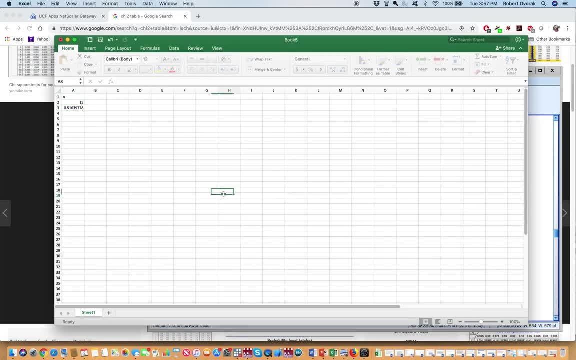 away from the mean that we are, and so our max here is 0.68. if we divide 0.68, our max here is 0.68. if we divide 0.68, our max here is 0.68. if we divide 0.68 by 0.044, let's just go- equals 0.68. 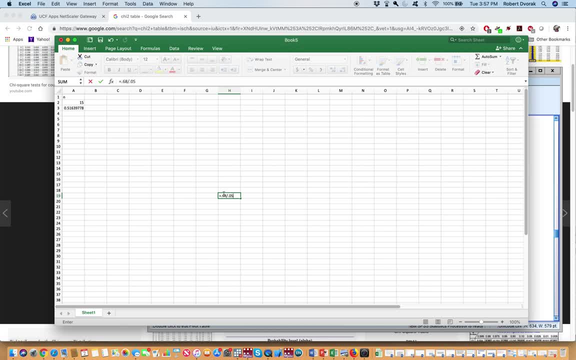 by 0.044, let's just go. equals 0.68 by 0.044. let's just go. equals 0.68 divided by 0.0. let's even call it 0.05. divided by 0.0: let's even call it 0.05. 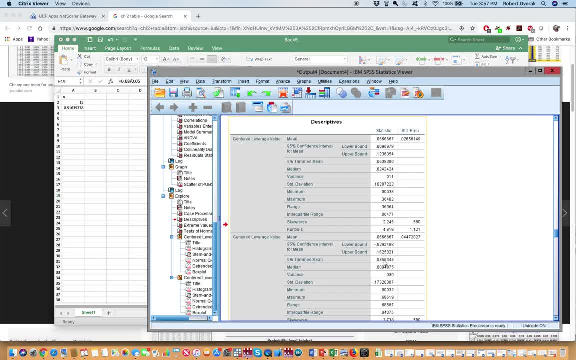 divided by 0.0. let's even call it 0.05. what the heck 13 standard deviations away? what the heck 13 standard deviations away? what the heck 13 standard deviations away? that seems like it's exerting an awful. that seems like it's exerting an awful. 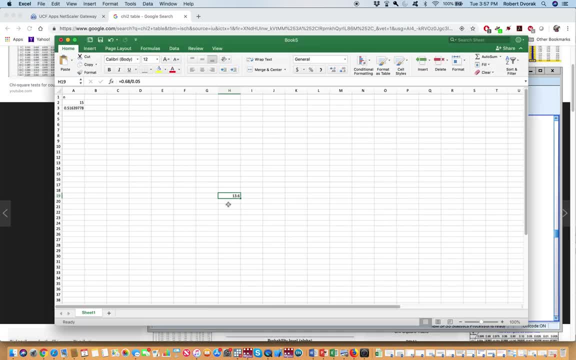 that seems like it's exerting an awful lot of leverage. if we do 0.36 by 0.03, lot of leverage. if we do 0.36 by 0.03, that's gonna be about 10 right equals. that's gonna be about 10 right equals. 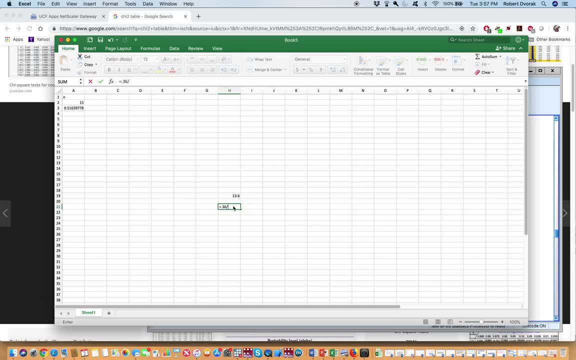 that's gonna be about 10 right equals equals 0.36 divided by 0.03 012. so even equals 0.36 divided by 0.03 012. so even equals 0.36 divided by 0.03 012. so even in the first model it was exerting quite. 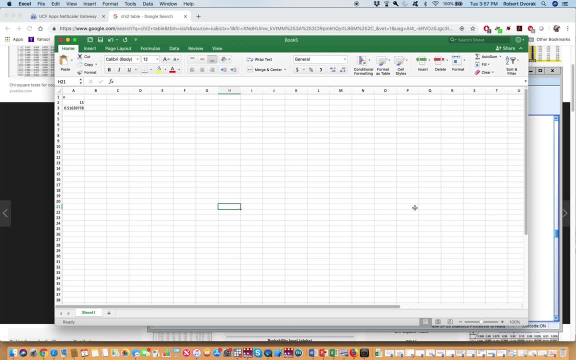 in the first model it was exerting- quite in the first model it was exerting quite a bit of leverage. the second model, also a bit of leverage. the second model, also a bit of leverage. the second model also exerting quite a bit of leverage. or the 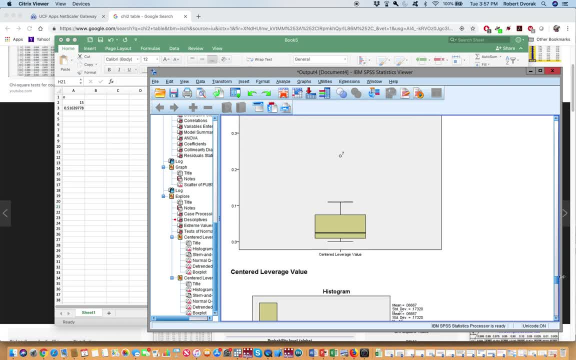 exerting quite a bit of leverage, or the exerting quite a bit of leverage, or the final model, the most important piece here, final model. the most important piece here, final model. the most important piece here is the: the change of 20- 20 percent is the, the change of 20- 20 percent. 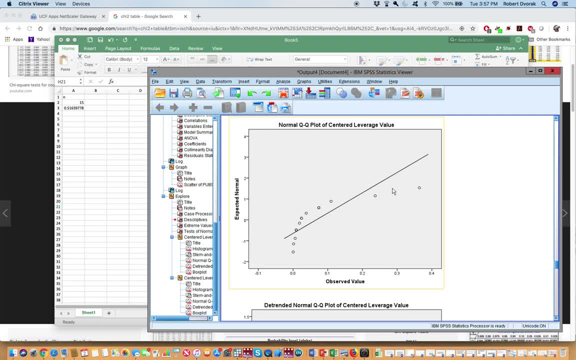 is the, the change of 20, 20 percent variance explained. you can see in our variance explained. you can see in our variance explained. you can see in our QQ plot. these, both of these observations, QQ plot, these, both of these observations, QQ plot these, both of these observations are problematic. of course, one of them. 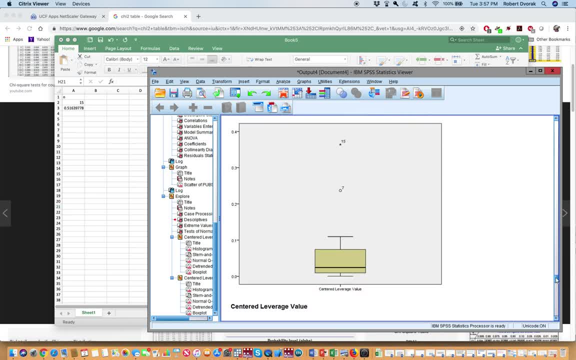 are problematic. of course one of them are problematic. of course one of them more so problematic. similarly, here we more so problematic. similarly, here we more so problematic. similarly, here we have a box plot. you can see 15 that we have a box plot. you can see 15 that we. 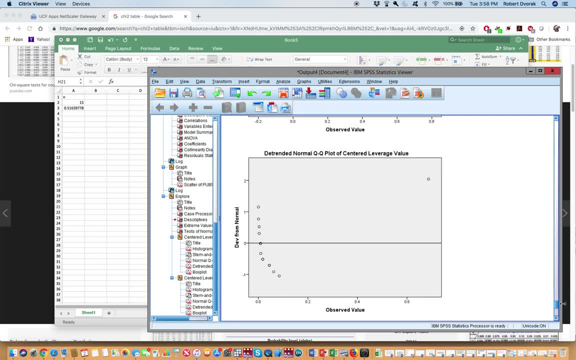 have a box plot. you can see 15 that we changed is really bad there it gets changed is really bad there it gets changed is really bad. there it gets worse as we move down here. notice that worse as we move down here. notice that worse as we move down here. notice that, as we made that one in the second. 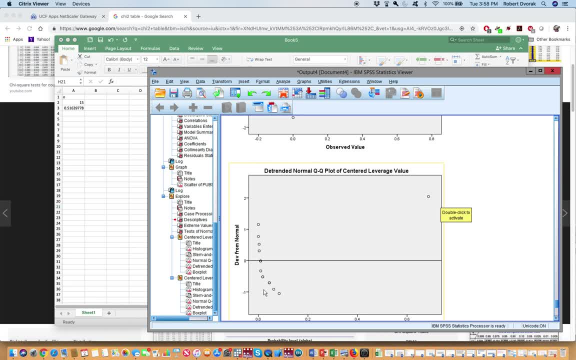 as we made that one in the second, as we made that one in the second analysis, it actually made the one. that analysis. it actually made the one, that analysis. it actually made the one that wasn't so bad, more in line, and then wasn't so bad, more in line, and then 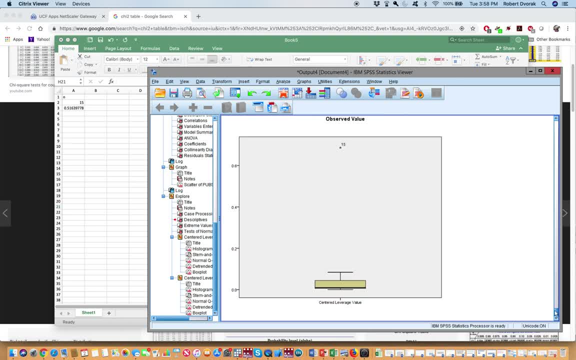 wasn't so bad, more in line, and then we've got this guy way over here. that's: we've got this guy way over here. that's: we've got this guy way over here. that's number 15. and in fact, when you have such number 15, and in fact, when you have such 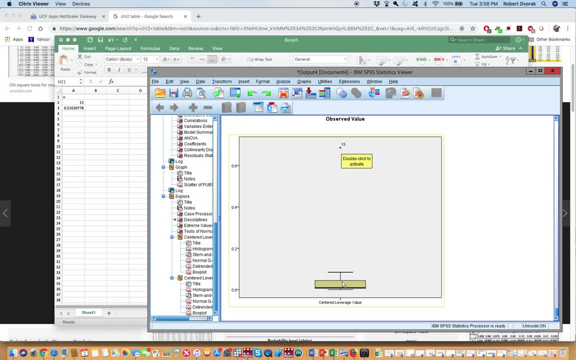 number 15 and in fact, when you have such an extreme outlier, it actually makes an extreme outlier. it actually makes an extreme outlier. it actually makes the other outliers seem like it's not. the other outliers seem like it's not. the other outliers seem like it's not nearly as bad. so the first way that we 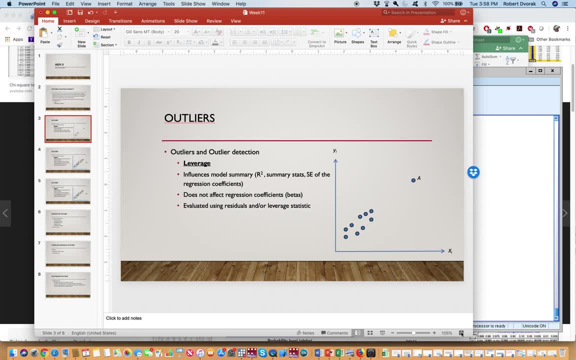 nearly as bad. so the first way that we nearly as bad. so the first way that we go about detecting outliers is by go about detecting outliers is by go about detecting outliers is by detecting leverage and examining detecting leverage and examining, detecting leverage and examining leverage through r-squared. our summary: 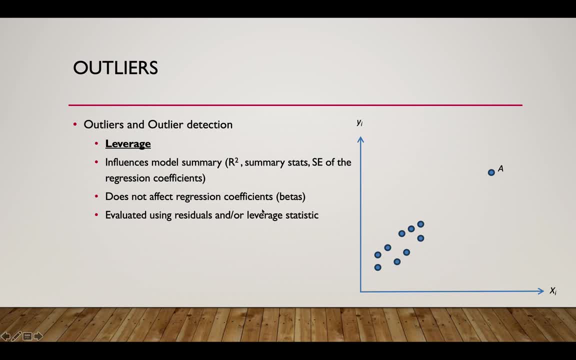 leverage through r-squared- our summary leverage through r-squared- our summary statistics. and using the, the basic statistics. and using the, the basic statistics. and using the, the basic leverage statistic, to determine whether leverage statistic to determine whether leverage statistic. to determine whether or not that should be removed or what. or not that should be removed, or what or not that should be removed, or what you're gonna do with it. it doesn't, you're gonna do with it. it doesn't, you're gonna do with it. it doesn't necessarily have to be removed and we'll. 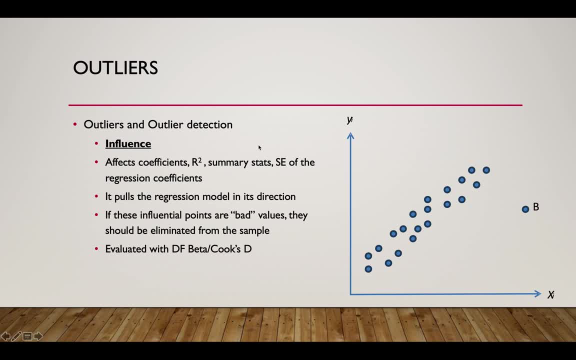 necessarily have to be removed, and we'll necessarily have to be removed, and we'll talk about that in just a little bit. alright, the next thing that we have is: alright, the next thing that we have is: alright, the next thing that we have is influence. so influence is a little bit. 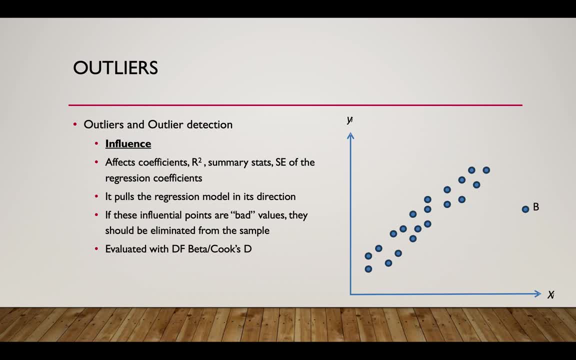 influence. so influence is a little bit influence, so influence is a little bit different right. influence affects your different right. influence affects your different right. influence affects your coefficients, your beta coefficients. it coefficients your beta coefficients. it coefficients your beta coefficients. it also affects your r-squared, your. 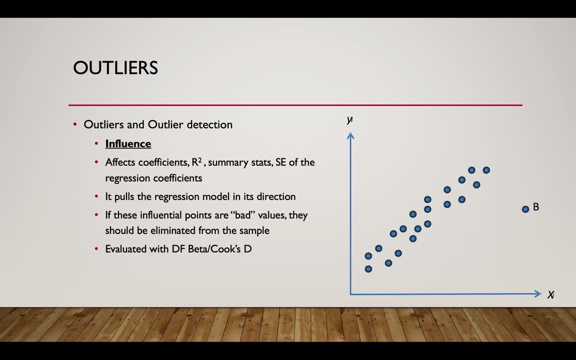 also affects your r-squared. your also affects your r-squared. your summary statistics: your standard error of summary statistics. your standard error of summary statistics. your standard error of your regression coefficients all kind. your regression coefficients all kind. your regression coefficients all kind of model related issues in general it. 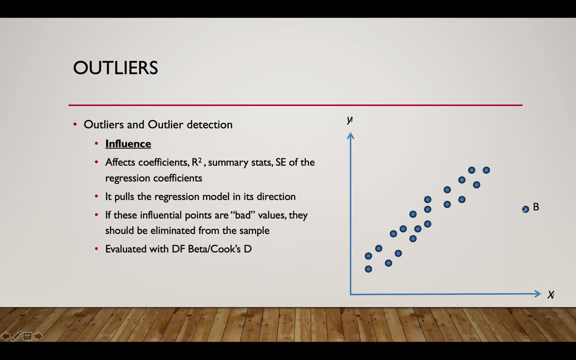 of model related issues in general. it of model related issues in general. it pulls your regression model in the. pulls your regression model in the. pulls your regression model in the direction of beta. it can move your direction of beta. it can move your direction of beta. it can move your intercept. note here that you would have. 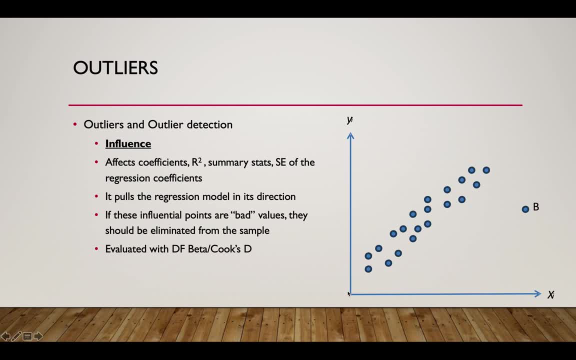 intercept. note here that you would have intercept. note here that you would have a nice line here, but, and you would have a nice line here, but, and you would have a nice line here, but, and you would have an intercept down here in contrast with an intercept down here, in contrast with. 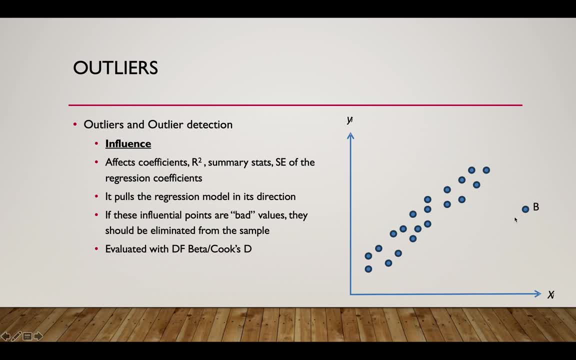 an intercept down here, in contrast with this thing here: it pulls your intercept. this thing here it pulls your intercept. this thing here it pulls your intercept up and it moves your regression line up and it moves your regression line up and it moves your regression line. these influential points are bad values. 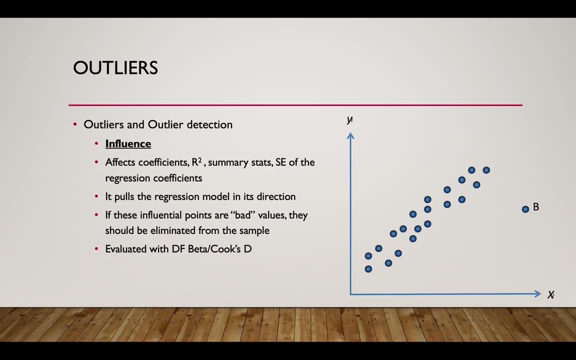 these influential points are bad values. these influential points are bad values and they should be eliminated from your and they should be eliminated from your and they should be eliminated from your sample, or, if they're, if they're bad sample, or if they're, if they're bad. 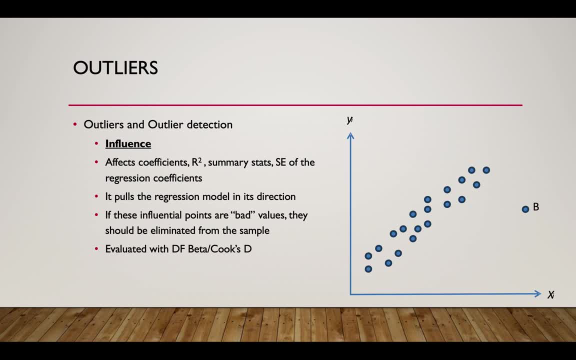 sample or, if they're, if they're bad values, they should be eliminated from values. they should be eliminated from values. they should be eliminated from your sample. you can check these with the your sample. you can check these with the your sample. you can check these with the DF, beta and cooks D. and we're gonna do. 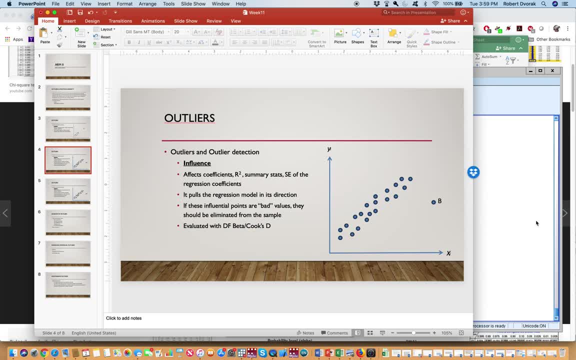 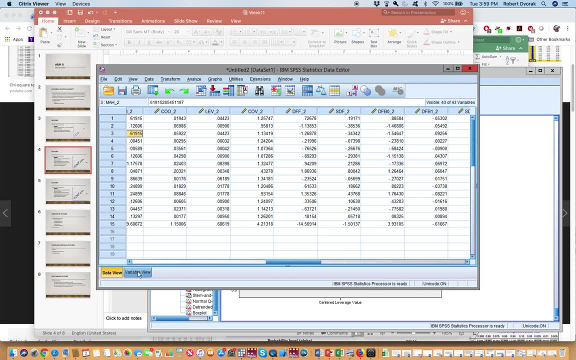 DF beta and cooks D, and we're gonna do DF beta and cooks D and we're gonna do that here in just a minute. so let's hop that here in just a minute. so let's hop that here in just a minute. so let's hop back over to SPSS and let's do this. we. 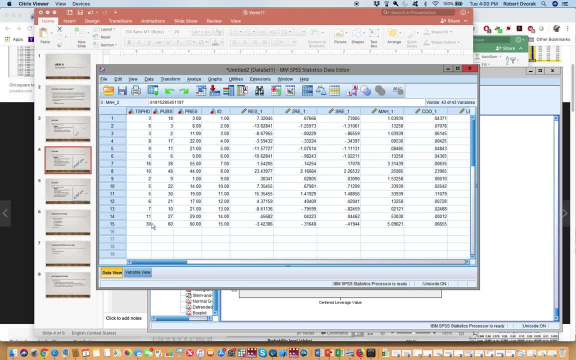 back over to SPSS, and let's do this. we back over to SPSS and let's do this. we want to look at our data. so before this, want to look at our data. so before this, want to look at our data. so before this was 18 and 37, but in 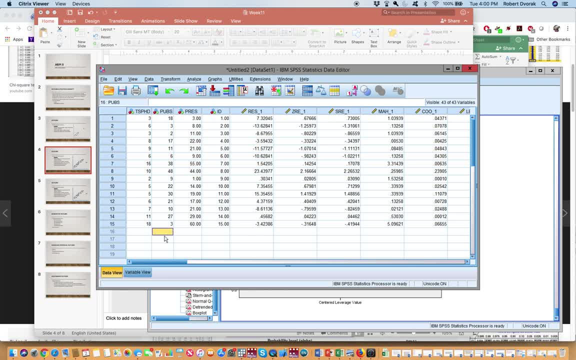 was 18 and 37, but in was 18 and 37. but in order to make this kind of cranky, let's go 18 and 3 order. to make this kind of cranky, let's go 18 and 3 order. to make this kind of cranky, let's go 18 and 3. let's go analyze. so we've. 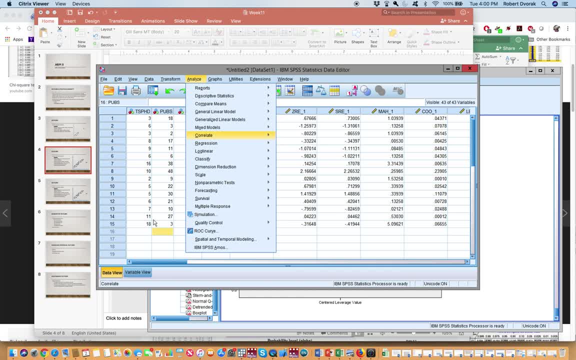 let's go analyze, so we've, let's go analyze, so we've only changed one variable. remember actually only changed one variable. remember actually only changed one variable. remember actually, let's, let's go 1837, what it was. let's let's go 1837, what it was. 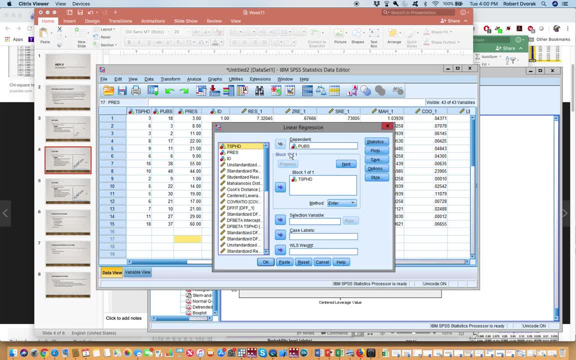 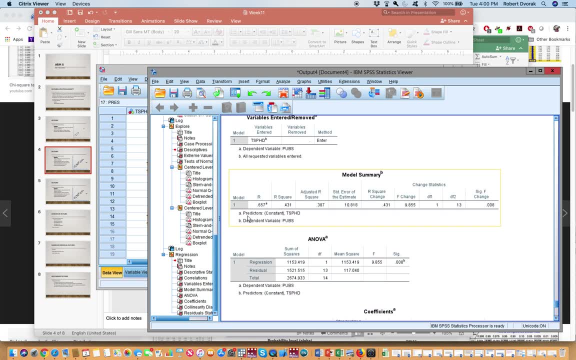 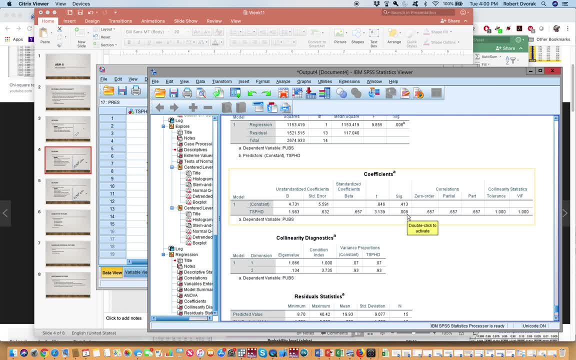 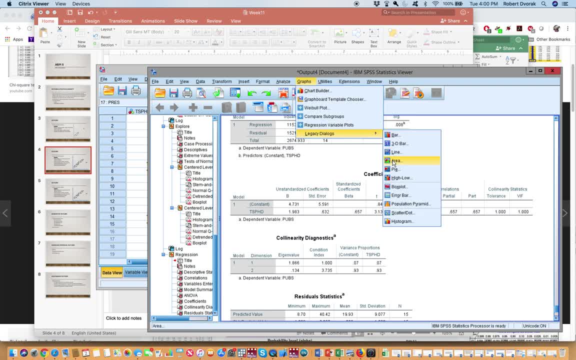 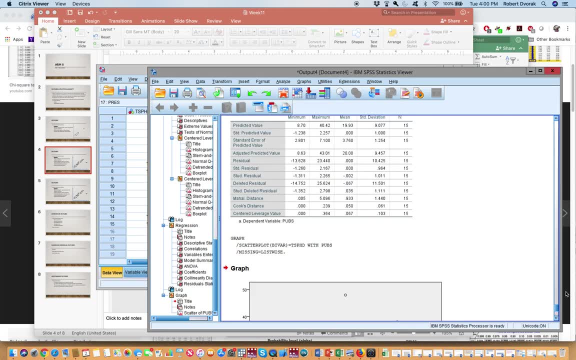 this is going to be the important piece. this is going to be the important piece. oh, let's go ahead and have a look at our. oh, let's go ahead and have a look at our. oh, let's go ahead and have a look at our box plot again. or I mean our, our basic. 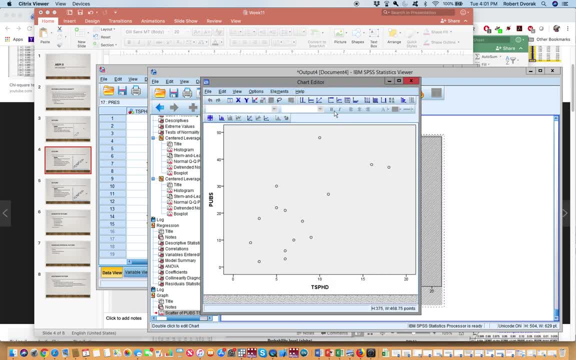 box plot again. or I mean our our basic box plot again. or I mean our our basic scatter plot, and let's throw our line in scatter plot and let's throw our line in scatter plot and let's throw our line in there. that should be there. there we go. 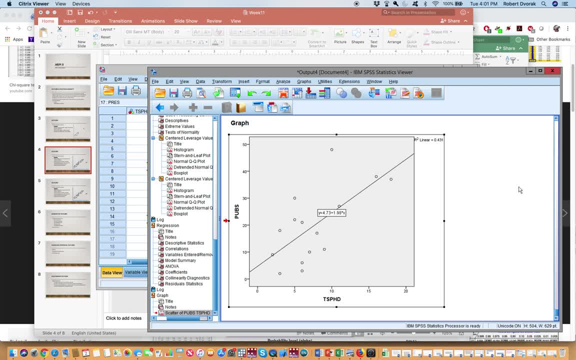 there. that should be there. there, we go there. that should be there. there we go close, that close. that this is what it close. that this is what it should look like. right? this is what our data should look like. right? this is what our data should look like. right? this is what our data normally looks like. let's change. 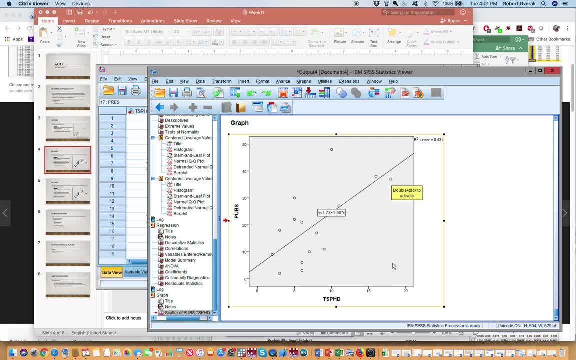 normally looks like, let's change. normally looks like, let's change just one point. we're gonna take this point, just one point. we're gonna take this point, just one point. we're gonna take this point here and we're gonna pull it down here and we're gonna pull it down. 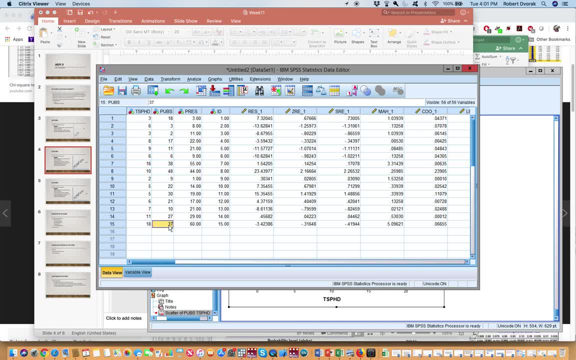 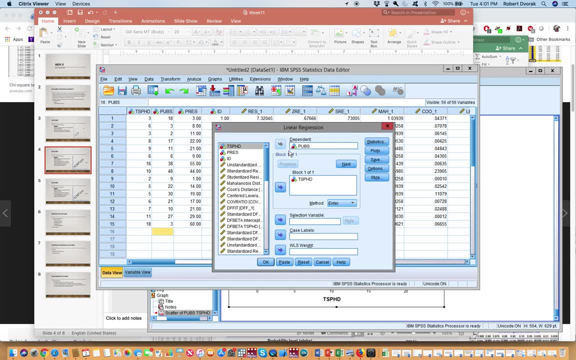 here and we're gonna pull it down here. 18 and 3 analyze regression linear. here 18 and 3 analyze regression linear. here 18 and 3 analyze regression linear. remember our R squared before was 0.43. remember our R squared before was 0.43. 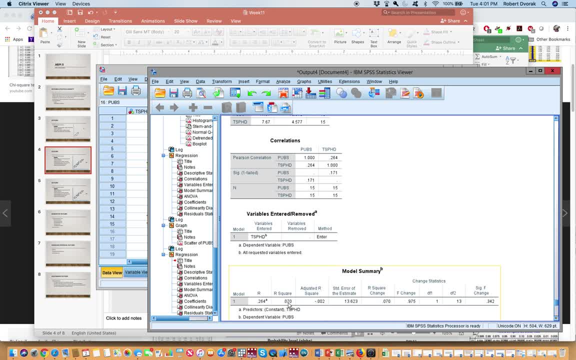 remember our R squared before was 0.43. our new R squared: 0.07. we changed one. our new R squared: 0.07. we changed one. our new R squared: 0.07. we changed one point and lost our ability to explain point and lost our ability to explain. 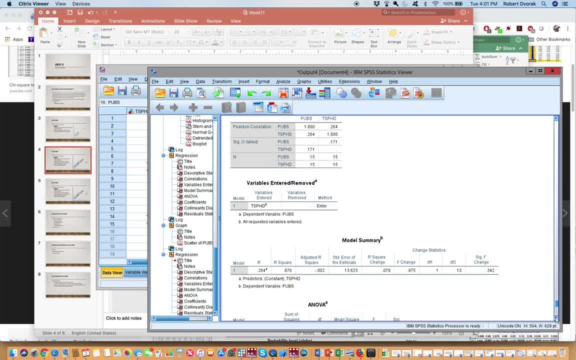 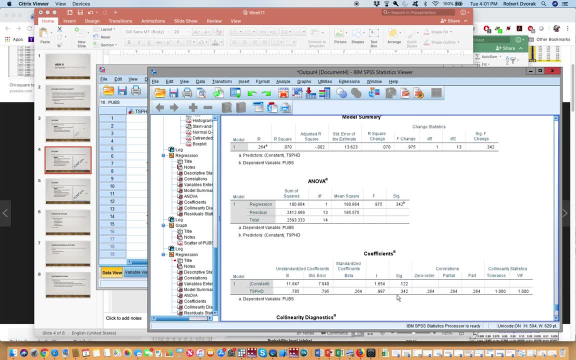 point and lost our ability to explain 35% of the variance in this model, our 35% of the variance in this model, our 35% of the variance in this model. our predictor before our beta coefficient predictor before our beta coefficient predictor, before our beta coefficient was 1.98 and it was statistically. 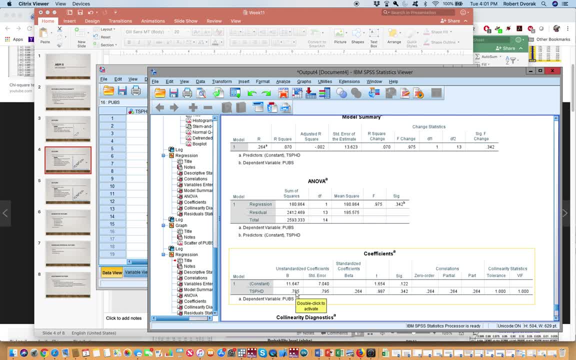 was 1.98 and it was statistically was 1.98 and it was statistically significant. now it is 0.785, still significant. now it is 0.785, still significant. now it is 0.785, still positive, but not very, not nearly, as 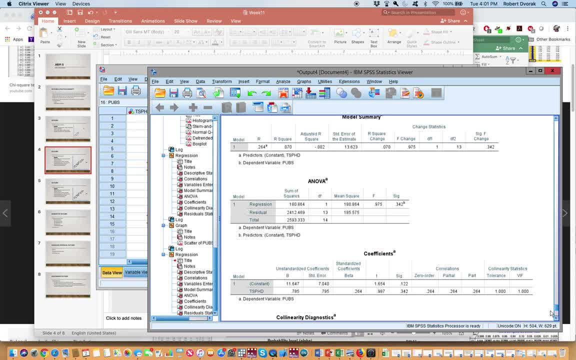 positive, but not very. not nearly as positive but not very, not nearly as strong, and the p-value is 0.342. it's no strong and the p-value is 0.342. it's no strong and the p-value is 0.342. it's no longer a significant predictor. this means 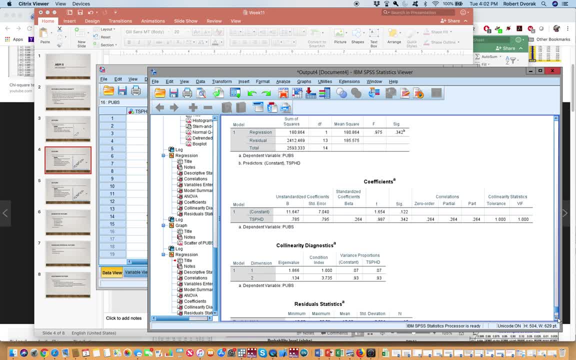 longer a significant predictor. this means longer a significant predictor. this means one outlying value. change this model so one outlying value. change this model so one outlying value. change this model so much that we no longer can explain much, that we no longer can explain much, that we no longer can explain, basically, any of the variance and our 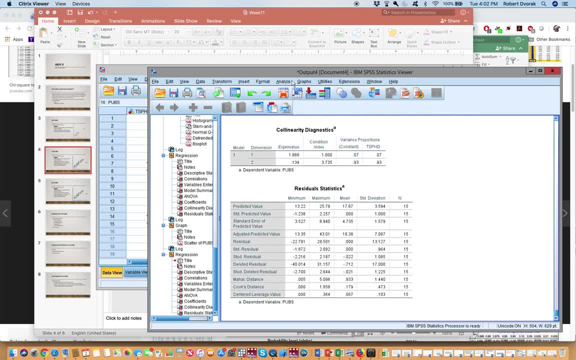 basically any of the variance and our basically any of the variance and our predictor is garbage at this point if we predictor is garbage at this point, if we predictor is garbage at this point, if we have a look at the graph that one, have a look at the graph that one. 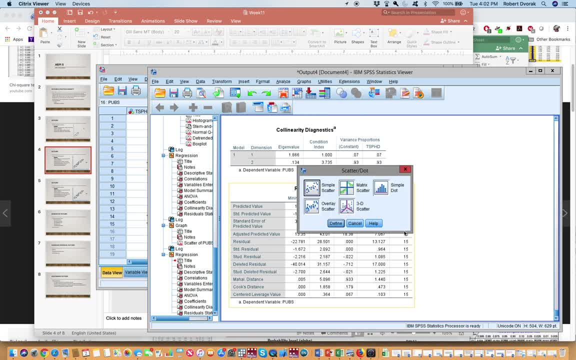 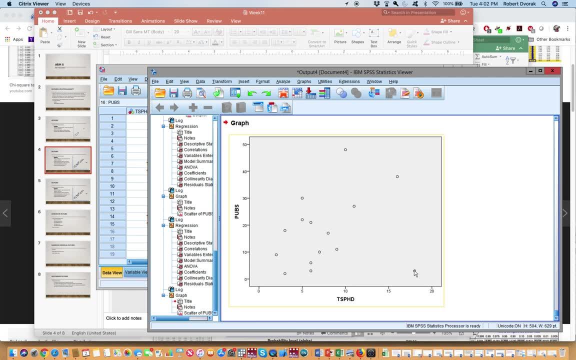 have a look at the graph that one change produces this: we have this guy down here. change produces this: we have this guy down here. change produces this: we have this guy down here. and if we want to add our line and if we want to add our line, 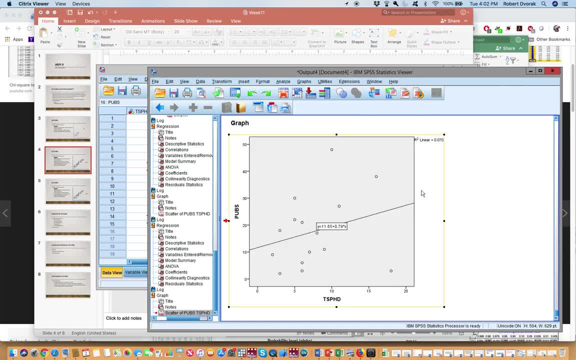 and if we want to add our line in there, in, there, in there, right, we see a very kind of drastic right. we see a very kind of drastic right. we see a very kind of drastic difference in slope and an intercept, our difference in slope and an intercept, our. 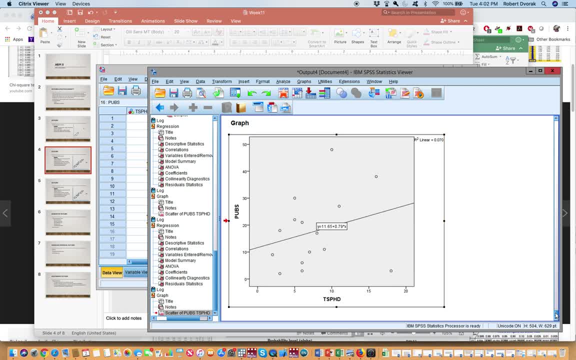 difference in slope and an intercept. our intercept is now is at 10 and our slope intercept is now is at 10 and our slope intercept is now is at 10 and our slope is almost flat. we scroll up here to our is almost flat. we scroll up here to our. 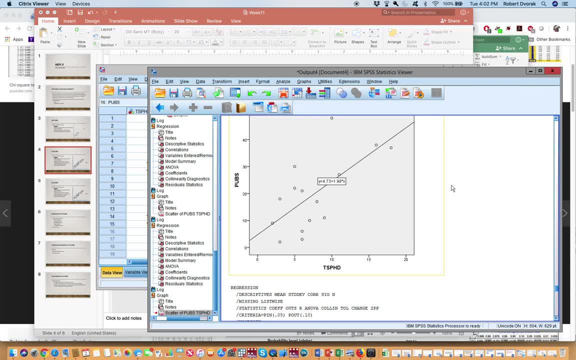 is almost flat. we scroll up here to our last one: our intercept is close to zero. last one: our intercept is close to zero. last one: our intercept is close to zero. pretty steep slope, very, very different. pretty steep slope, very, very different. pretty steep slope, very, very different. let's have a look at these statistics. 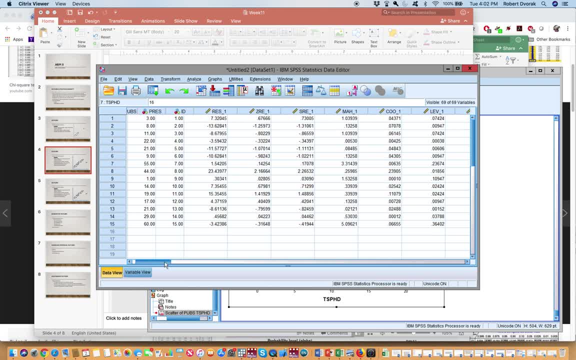 let's have a look at these statistics. let's have a look at these statistics now. so one of the ways that we can tell now. so one of the ways that we can tell now. so one of the ways that we can tell if a variable is exerting significant. 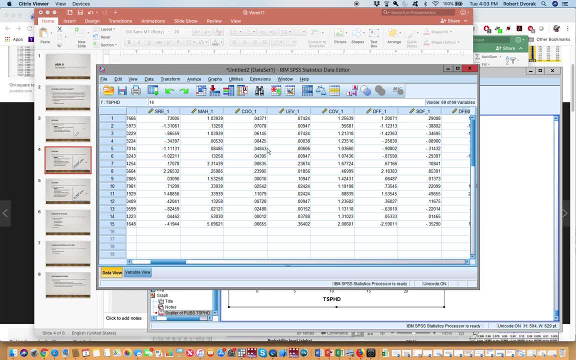 if a variable is exerting significant. if a variable is exerting significant influence or- I'm sorry, yes- significant influence or, I'm sorry, yes, significant influence or, I'm sorry, yes, significant influence is cooks D and it's called influence is cooks D and it's called. 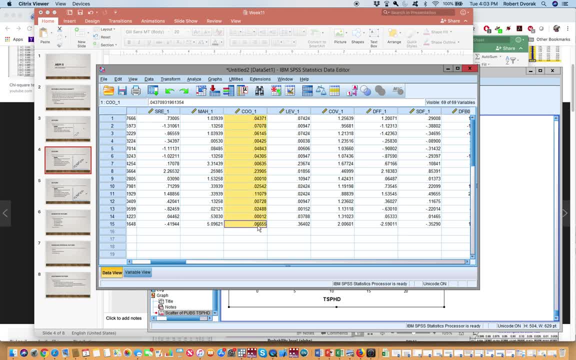 influence is cooks D, and it's called coup here in SPSS, and so we have a range coup here in SPSS, and so we have a range coup here in SPSS, and so we have a range of cooks D, and cooks D has a nice cutoff. 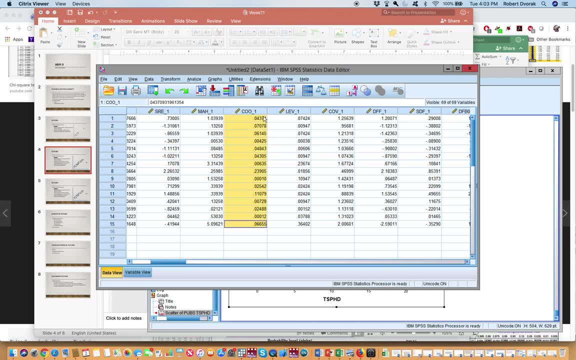 of cooks D and cooks D has a nice cutoff of cooks D and cooks D has a nice cutoff that we don't get with a lot of the. that we don't get with a lot of the. that we don't get with a lot of the other variables. but cooks D has a cutoff. 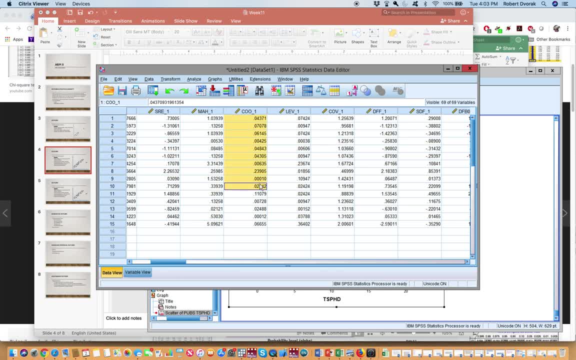 other variables, but cooks D has a cutoff. other variables, but cooks D has a cutoff of one and none of these have a cutoff of one and none of these have a cutoff of one and none of these have a cutoff of one. remember, this was our first of one. remember, this was our first. 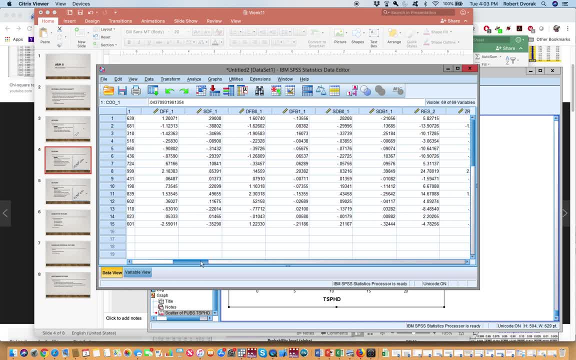 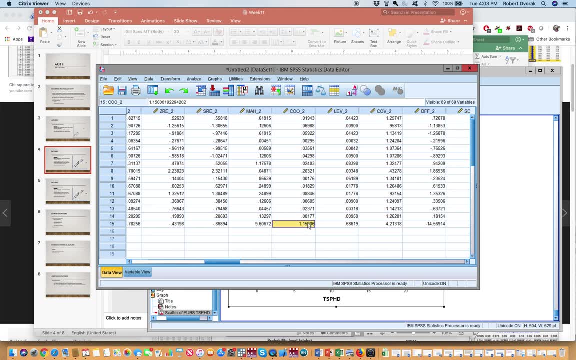 of one. remember this was our first regression model that we ran. then we ran regression model that we ran. then we ran regression model that we ran. then we ran a regression model where we put a. a regression model where we put a. a regression model where we put a variable. that was kind of way out there. 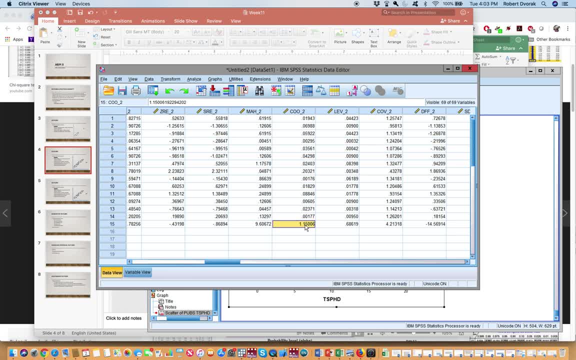 variable, that was kind of way out there. variable, that was kind of way out there. remember this was when we were looking. remember this was when we were looking. remember this was when we were looking at leverage and we have a cook- see now at leverage. and we have a cook- see now. 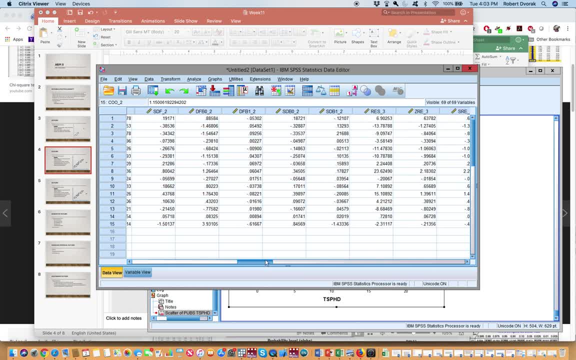 at leverage and we have a cook see now that is higher, and then we tried to that is higher and then we tried to that is higher and then we tried to recalculate that and make that a little recalculate that and make that a little recalculate that and make that a little bit closer and to the line of regression. 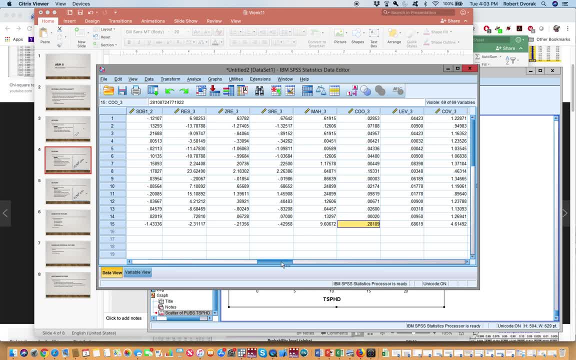 bit closer and to the line of regression, bit closer and to the line of regression. and when we did that, our cooks D came, and when we did that, our cooks D came, and when we did that our cooks D came down. then we ran another model where we 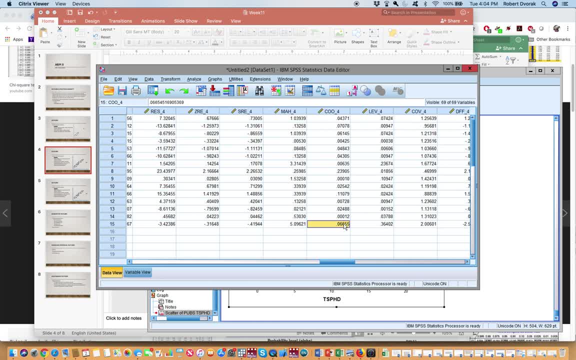 down. then we ran another model where we down. then we ran another model where we just looked at the exact same basic, just looked at the exact same basic, just looked at the exact same basic regression model. we set all of our data regression model. we set all of our data. 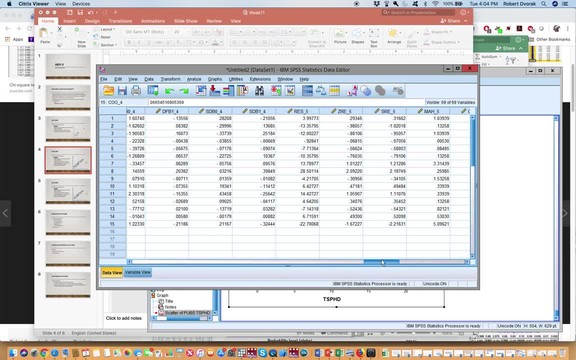 regression model. we set all of our data back to where it should be, and then our back to where it should be, and then our back to where it should be, and then our last model. here is where we moved cooks. last model: here is where we moved cooks. 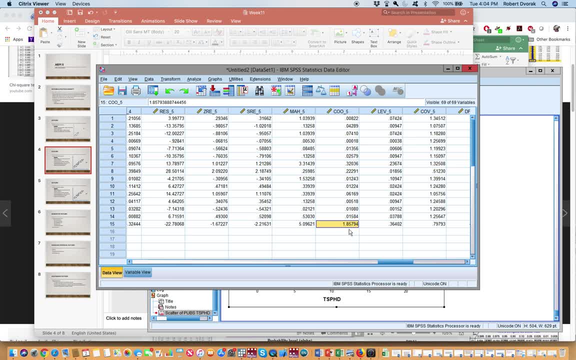 last model here is where we moved cooks D or where we moved our variable way D, or where we moved our variable way D or where we moved our variable way down and we see that our cooks D is down and we see that our cooks D is down and we see that our cooks D is almost 2. this is extreme. we can also. 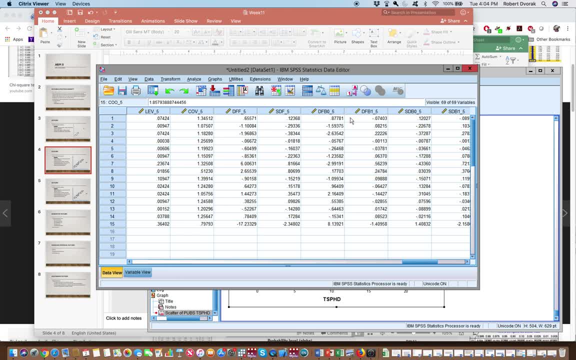 almost 2. this is extreme. we can also almost 2. this is extreme. we can also look at what's called DF, beta and DF. look at what's called DF, beta and DF. look at what's called DF, beta and DF beta. looks at the effects on both your. 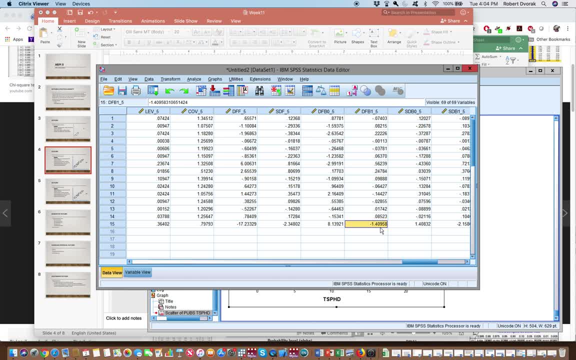 beta looks at the effects on both your beta, looks at the effects on both your intercept, but more importantly on the intercept, but more importantly on the intercept, but more importantly on the slope, and it says: how much does this one slope? and it says: how much does this one? 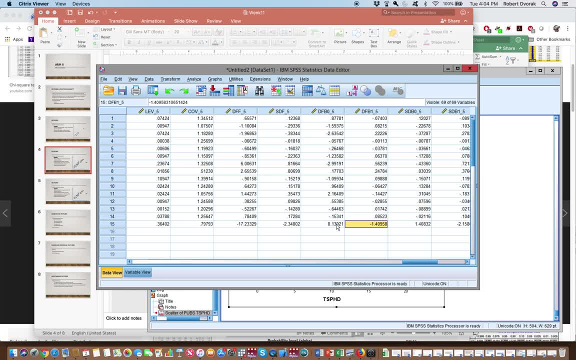 slope and it says: how much does this one value affect? either the intercept of the value affect, either the intercept of the value affect either the intercept of the slope, and if you were to remove it and slope, and if you were to remove it and slope, and if you were to remove it, and in this case, if you were to remove this, 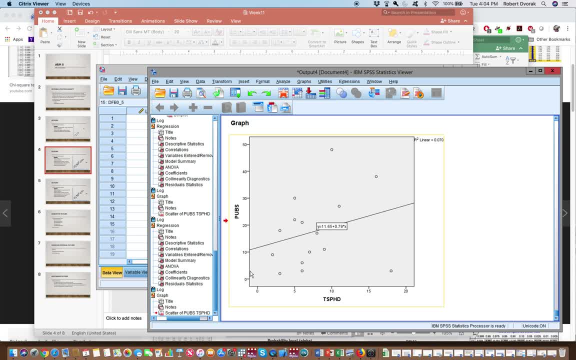 in this case, if you were to remove this, in this case, if you were to remove this one outlying value, we would drop our one outlying value. we would drop our one outlying value, we would drop our intercept by eight, by a value of whoops. 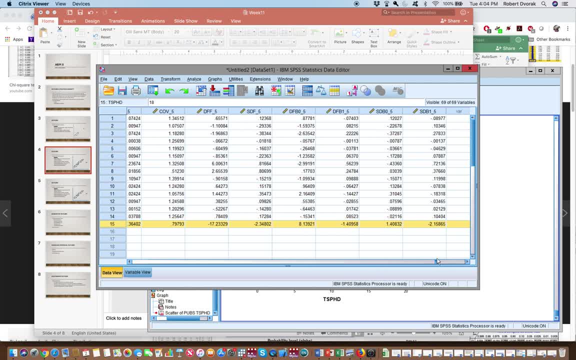 intercept by eight by a value of whoops. intercept by eight by a value of whoops. shoot, I scrolled all the way over here, shoot, I scrolled all the way over here, shoot, I scrolled all the way over here by a value of eight. point one, three and. 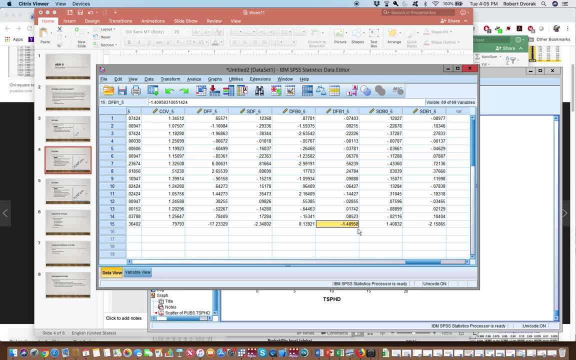 by a value of eight point one three and by a value of eight point one three, and we would increase our slope by a value. we would increase our slope by a value. we would increase our slope by a value of 1.4. this is telling you what this. 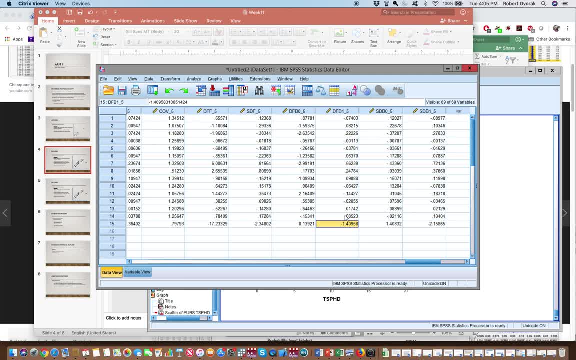 of 1.4. this is telling you what this of 1.4. this is telling you what this observation is doing to the intercept observation is doing to the intercept observation is doing to the intercept and the slope and that is pretty, and the slope and that is pretty. 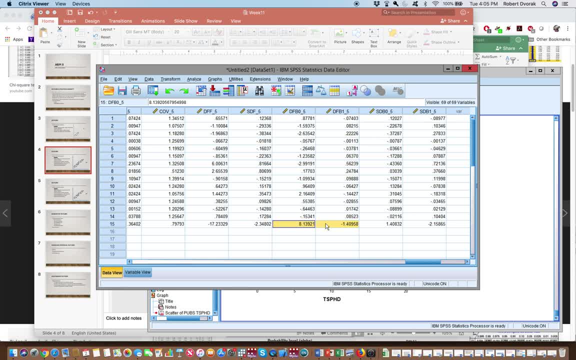 and the slope and that is pretty drastic. you can't make a really good drastic. you can't make a really good drastic. you can't make a really good description or get really good description, or get really good description or get really good comparison. these are not cutoffs here. 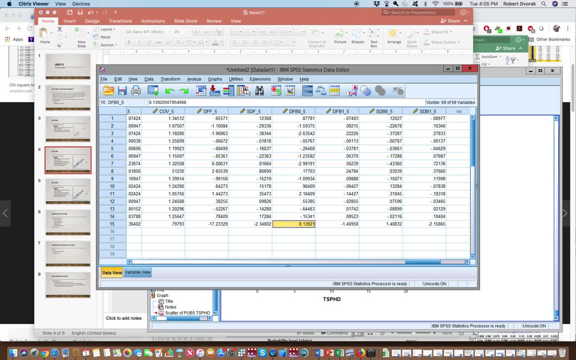 comparison: these are not cutoffs here. comparison: these are not cutoffs here, though they can be cutoffs because you, though, they can be cutoffs. because you, though, they can be cutoffs, because you can do something like this, we can go, can do something like this, we can go. 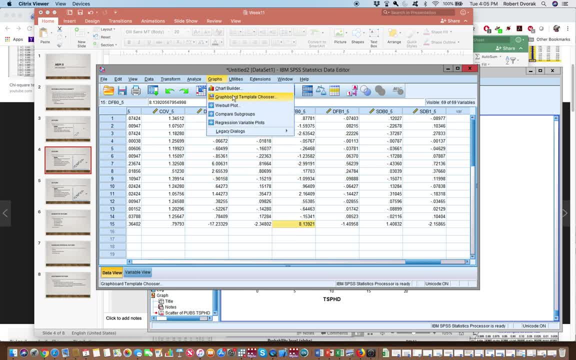 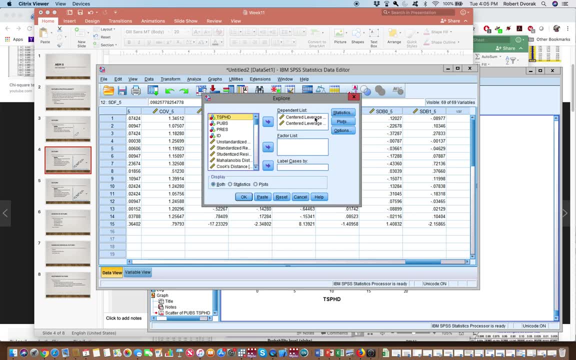 can do something like this. we can go graph: actually, let's go analyze graph. actually, let's go analyze graph. actually, let's go analyze descriptives. explore, remove leverage descriptives. explore, remove leverage descriptives. explore, remove leverage this time. and we are going to look at. 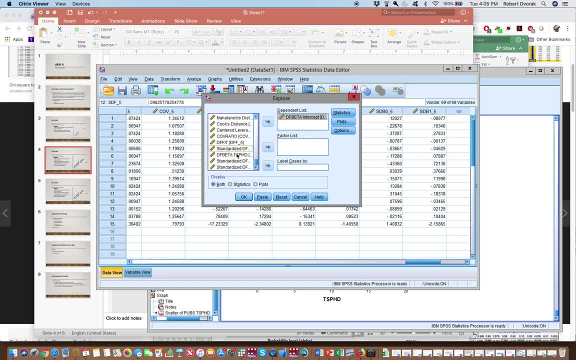 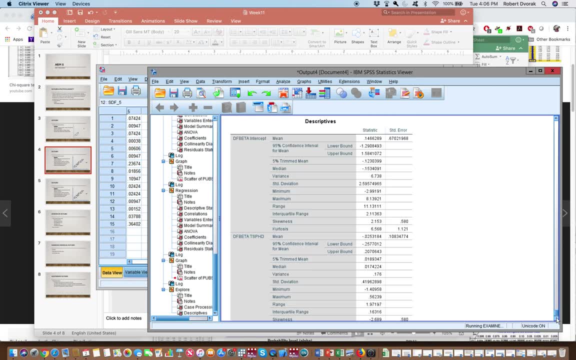 this time, and we are going to look at this time and we are going to look at DF beta intercepts and DF beta slope, DF beta intercepts and DF beta slope, DF beta intercepts and DF beta slope and and and let's just have a look at these and 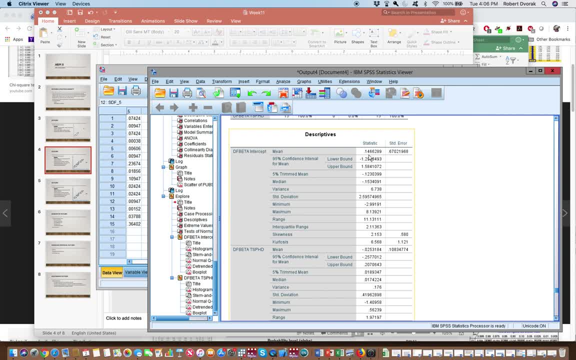 let's just have a look at these, and let's just have a look at these, and so we can see that the average change in, so we can see that the average change in, so we can see that the average change in intercepts for any one of those is 0.14. 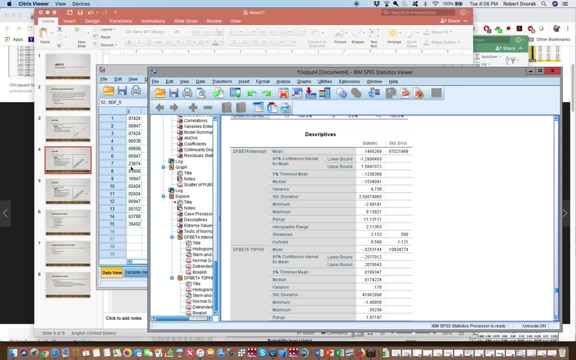 intercepts for any one of those is 0.14. intercepts for any one of those is 0.14, with a standard error of 0.67. now, if we with a standard error of 0.67, now, if we with a standard error of 0.67, now, if we divide points that that 8 by 0.67 equals. 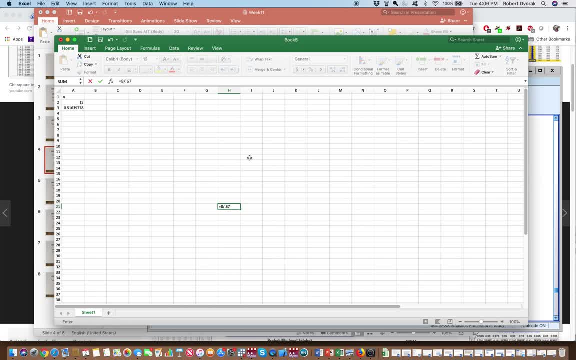 divide. points that that 8 by 0.67 equals divide. points that that 8 by 0.67 equals 8 divided by 0.67, and I'm saying 8 it, 8 divided by 0.67 and I'm saying 8 it. 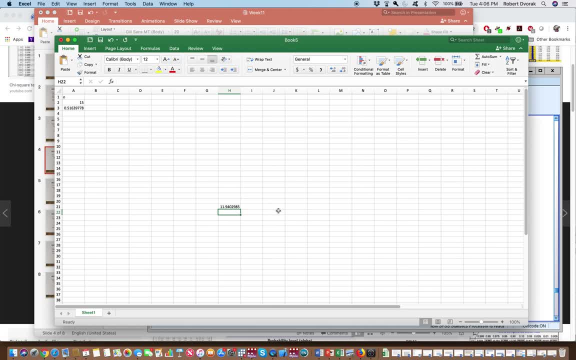 8 divided by 0.67, and I'm saying 8, it was technically 8.13, if you remember, was technically 8.13, if you remember, was technically 8.13, if you remember, because that was the effect of that, because that was the effect of that. 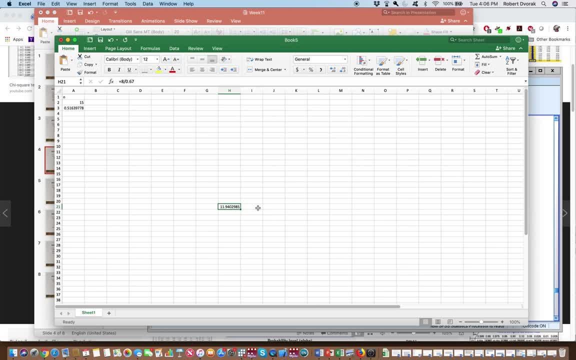 because that was the effect of that single observation on the intercept and single observation on the intercept and single observation on the intercept and we can see that this is a z-score of. we can see that this is a z-score of. we can see that this is a z-score of 11.94. that means that that observation. 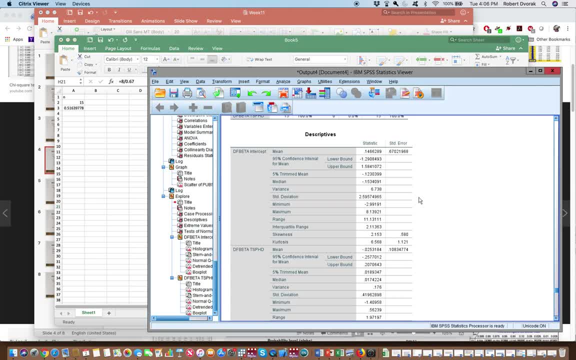 11.94. that means that that observation 11.94. that means that that observation is changing the intercept by 11, almost is changing the intercept by 11, almost is changing the intercept by 11, almost. 12 standard deviations- the other piece. 12 standard deviations- the other piece. 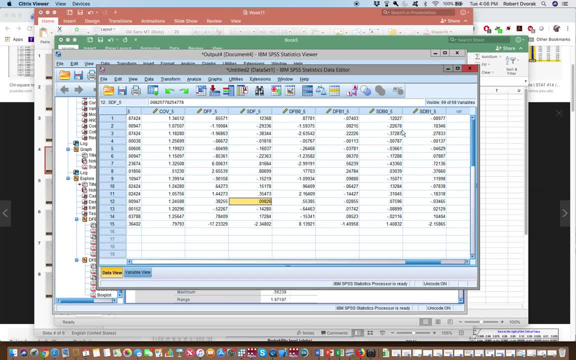 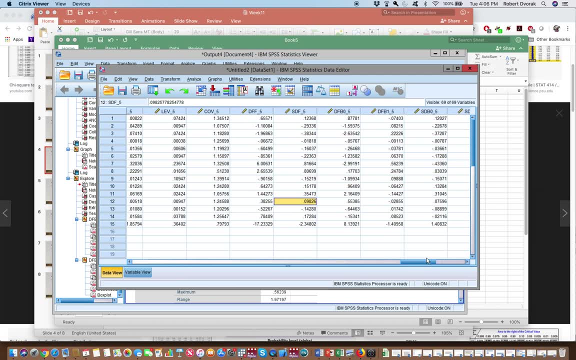 12 standard deviations. the other piece, the other data here is our slope, our df. the other data here is our slope, our df. the other data here is our slope, our df, beta slope, beta slope. where's my df beta? thank you, so we had. where's my df beta? thank you, so we had. 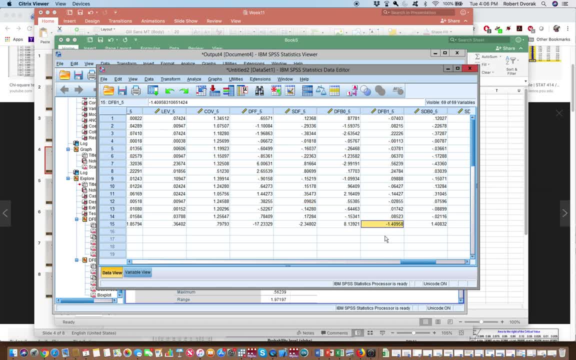 where's my df beta? thank you. so we had eight point one. three minus one point eight point one. three minus one point eight point one. three minus one point four one. let's look on our output. what four one? let's look on our output. what four one? let's look on our output. what is our standard error for the slope? it? 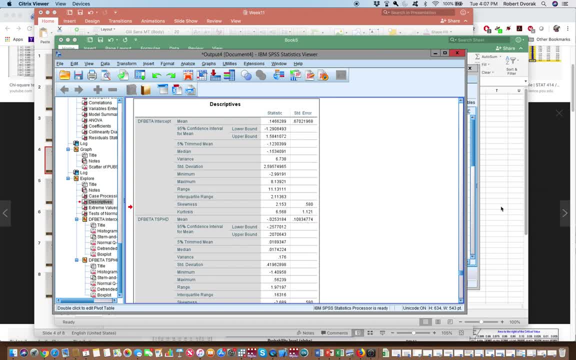 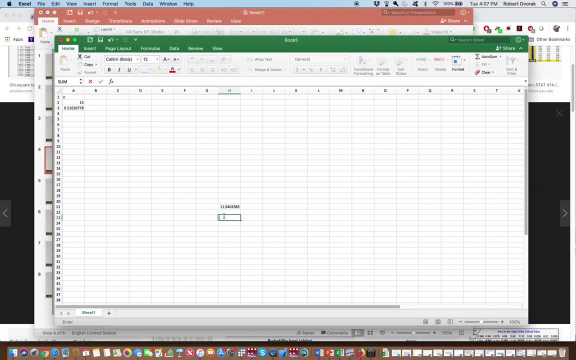 is our standard error for the slope. it is our standard error for the slope. it is point zero. we'll call point one. one is point zero. we'll call point one. one is point zero. we'll call point one one. so minus point one, four, oops, equals. 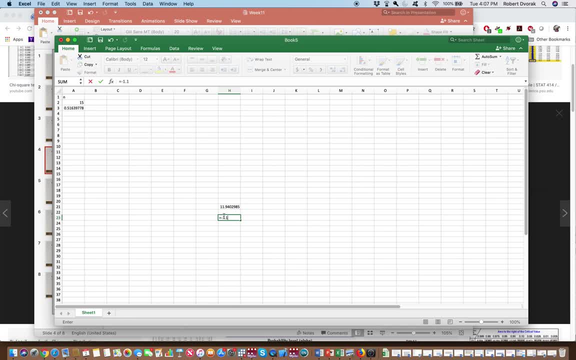 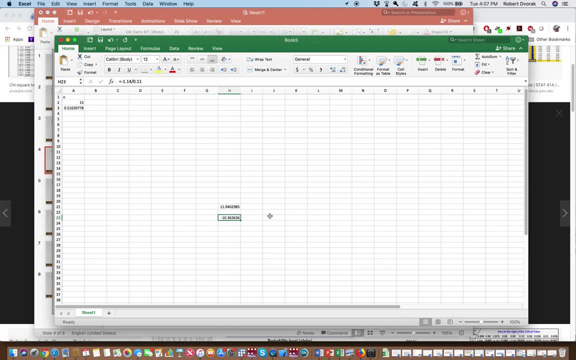 and it is affecting the slope by about ten. and it is affecting the slope by about ten standard deviations- a z-score of ten standard deviations. a z-score of ten standard deviations. a z-score of ten. that is pretty a pretty dramatic effect. that is pretty a pretty dramatic effect. 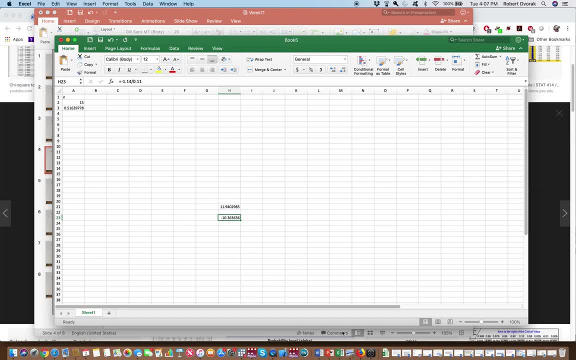 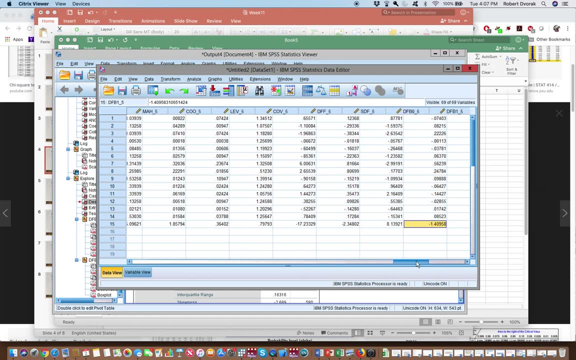 that is pretty a pretty dramatic effect on the slope. and so we can conclude from on the slope, and so we can conclude from on the slope, and so we can conclude from these that at least that observation is these, that at least that observation is these, that at least that observation is having a pretty significant effect on 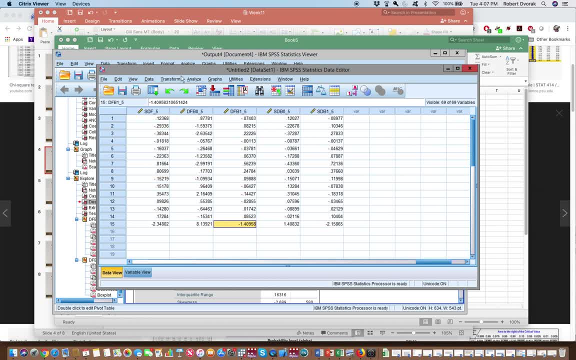 having a pretty significant effect on having a pretty significant effect on these right and if you want, we can do these right, and if you want, we can do these right and if you want, we can do. you can do something like this, you can go. you can do something like this, you can go. 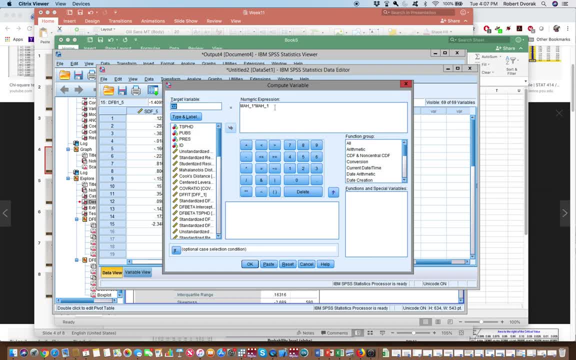 you can do something like this: you can go transform compute variable and we can transform compute variable and we can transform compute variable and we can say D F I effect and this is going to say D F I effect, and this is going to say D F I effect and this is going to give us the effect of the intercept. or 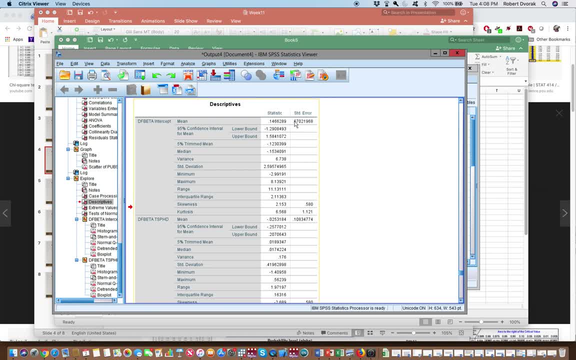 give us the effect of the intercept, or give us the effect of the intercept, or the effect of every single observation, the effect of every single observation, the effect of every single observation on the intercept. real quick, it was point on the intercept. real quick. it was point on the intercept. real quick. it was point six. seven, okay, divided by point six. 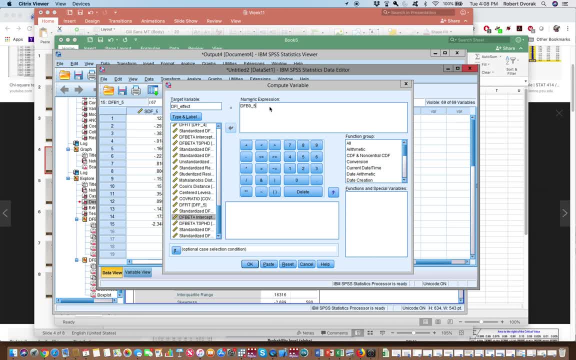 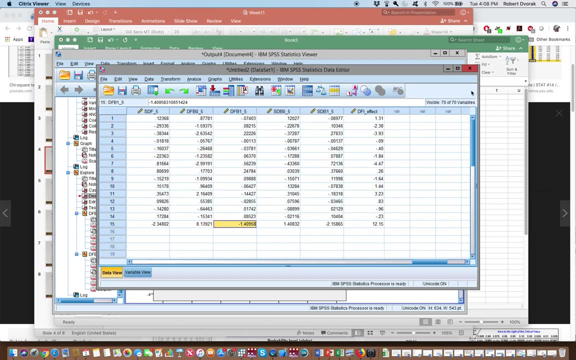 six, seven, okay, divided by point six, six, seven, okay, divided by point six, seven, seven, seven, seven. come on slow computer divided by point. come on slow computer divided by point. come on slow computer divided by point six, seven, all right, and let's hop over here. let's. 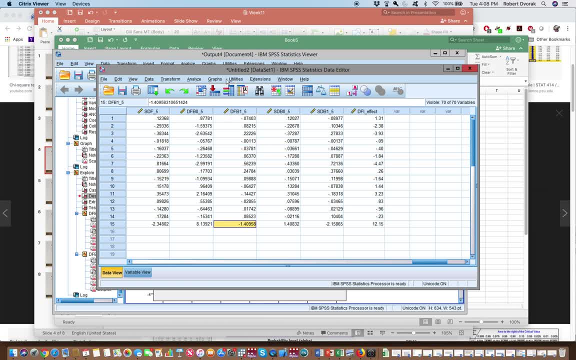 all right and let's hop over here. let's all right and let's hop over here. let's look at our data. we can actually do look at our data. we can actually do look at our data. we can actually do something after we've done that, we can. 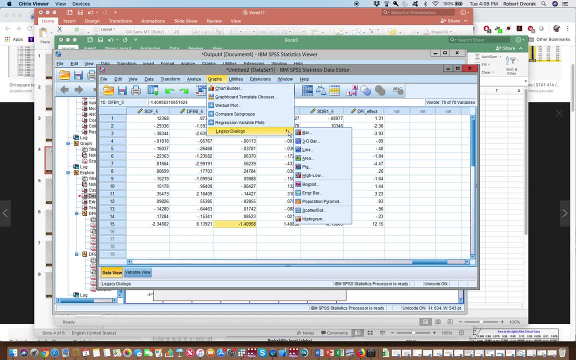 something. after we've done that, we can something after we've done that. we can go graph legacy dialog and we can just go graph legacy dialog and we can just go graph legacy dialog and we can just do a bar chart, do a bar chart, do a bar chart. actually, let's not do a bar chart, let's go. 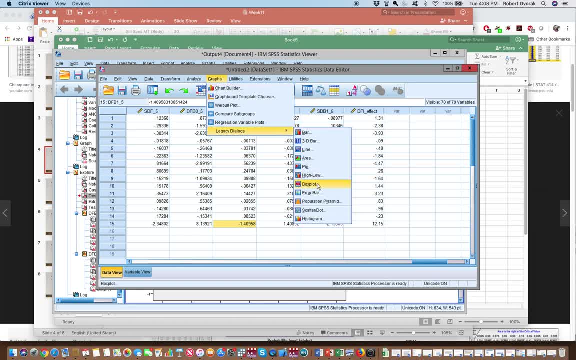 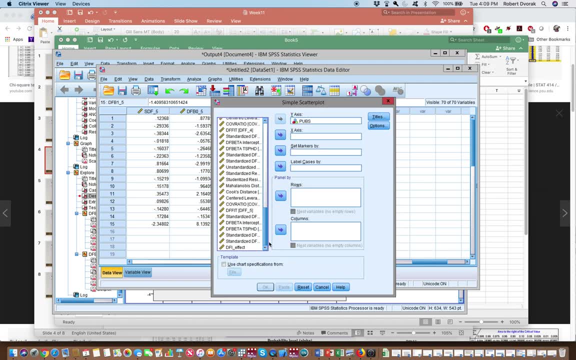 actually, let's not do a bar chart, let's go actually, let's not do a bar chart, let's go graphs- legacy dialog scatter. and let's graphs- legacy dialog scatter. and let's graphs- legacy dialog scatter. and let's go on our x-axis, let's just put people. 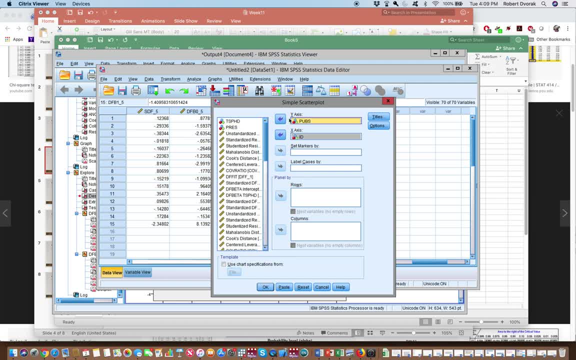 go on our x-axis, let's just put people. go on our x-axis, let's just put people ID and on our y-axis let's put this ID and on our y-axis let's put this ID and on our y-axis let's put this effect on the intercept, and this will. 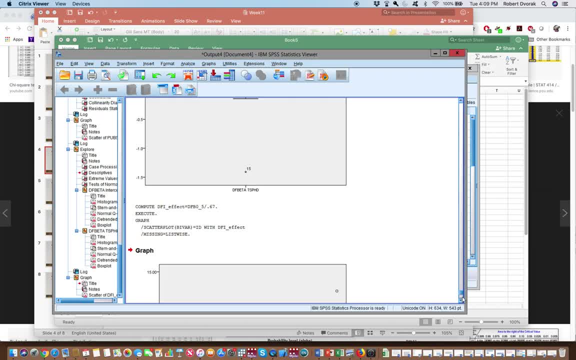 effect on the intercept and this will effect on the intercept and this will give us a graph of people by their effect. give us a graph of people by their effect. give us a graph of people by their effect on the intercept, and you can effect on the intercept and you can. 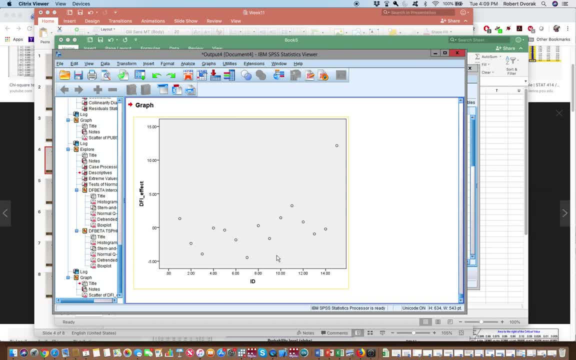 effect on the intercept. and you can see that we have like a fairly normal see, that we have like a fairly normal see, that we have like a fairly normal distribution of effects on the intercept. distribution of effects on the intercept. distribution of effects on the intercept across people, with one person causing a. 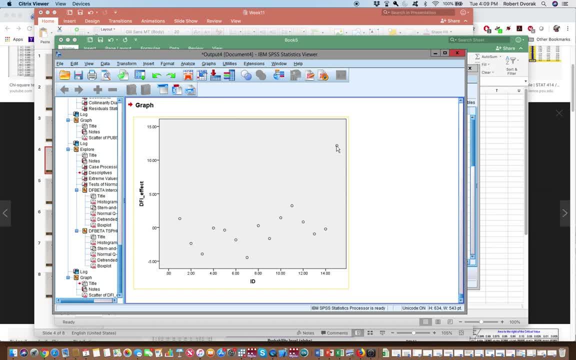 across people with one person causing a, across people with one person causing a pretty dramatic effect. I would say that pretty dramatic effect. I would say that pretty dramatic effect. I would say that this guy is problematic for the, this guy is problematic for the, this guy is problematic for the intercept. we can do the exact same thing. 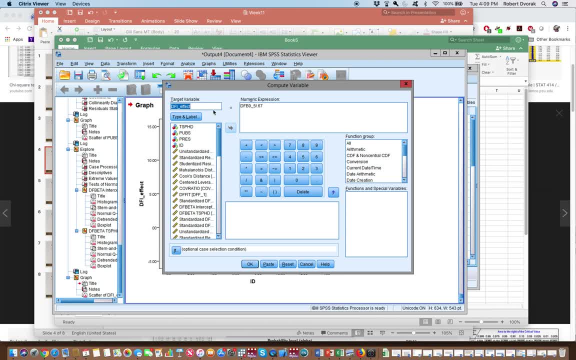 intercept, we can do the exact same thing. intercept, we can do the exact same thing. data oops- transform compute, and let's go. data oops- transform compute, and let's go. data oops- transform compute, and let's go DFS effect. this is going to be the 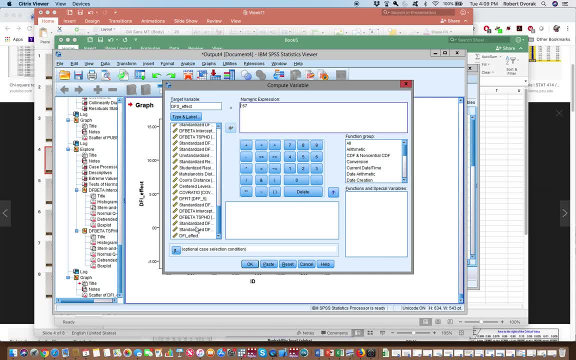 DFS effect. this is going to be the DFS effect. this is going to be the effect of on our slope, and so we have effect of on our slope, and so we have effect of on our slope. and so we have D F, beta s PhD, and it was 0.11 was our. 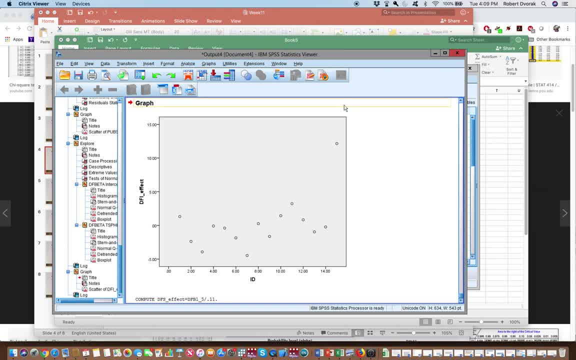 D F beta s PhD, and it was 0.11. was our D F beta s PhD, and it was 0.11. was our standard error there, calculate that and standard error there, calculate that and standard error there, calculate that, and then again we can go grass legacy. 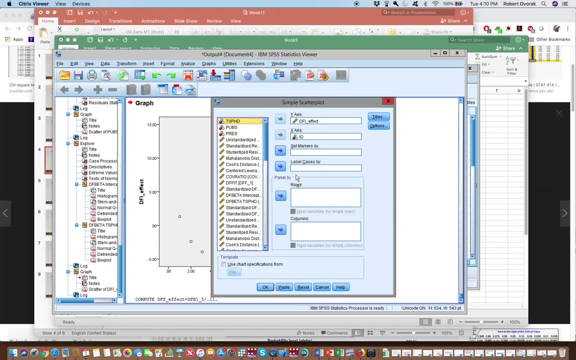 then again we can go grass legacy. then again we can go grass legacy. dialogues scatter. okay, we're going to do dialogues scatter. okay, we're going to do dialogues scatter. okay, we're going to do DFS effect this time instead of DFI. DFS effect this time instead of DFI. 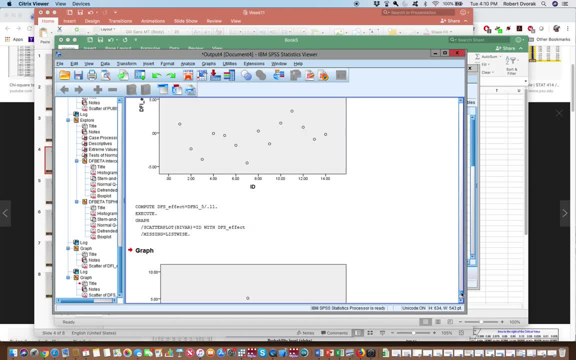 DFS effect this time instead of DFI effect. and what we see here effect and what we see here here effect. and what we see here here is again, these are the kind of general is again. these are the kind of general is again. these are the kind of general effects that we have on the intercept. 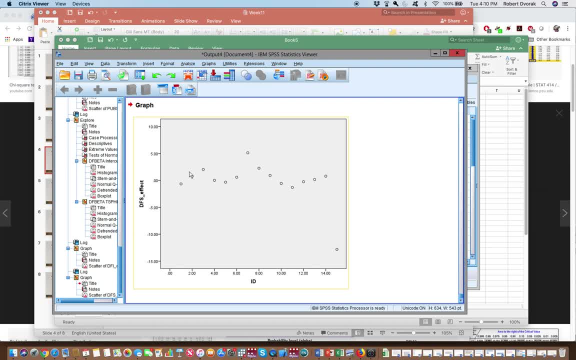 effects that we have on the intercept, effects that we have on the intercept, if we were to remove any one of these. and if we were to remove any one of these, and if we were to remove any one of these- and they're pretty close to zero, right. 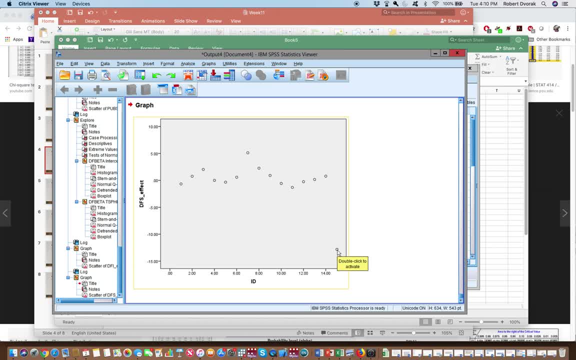 they're pretty close to zero, right? they're pretty close to zero, right, but we have this one person who is, but we have this one person who is. but we have this one person who is exerting a dramatic effect on our slope, exerting a dramatic effect on our slope. 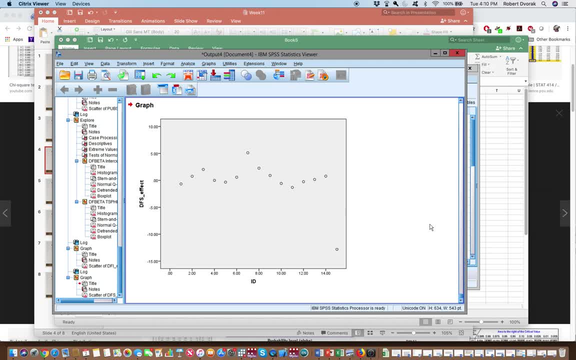 exerting a dramatic effect on our slope. this person is problematic for sure, and this person is problematic for sure, and this person is problematic for sure, and that is significant influence another, that is significant influence another, that is significant influence another. and so that is looking at the DF. 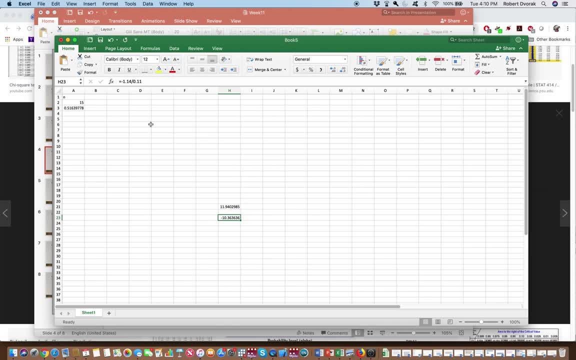 and so that is looking at the DF, and so that is looking at the DF statistics for both the intercept and statistics for both the intercept and statistics for both the intercept and the slope. you can also look at that, the slope. you can also look at that, the slope. you can also look at that Cook's distance to get roughly a similar. 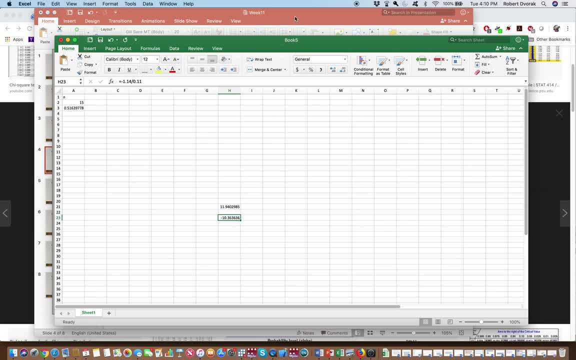 Cook's distance to get roughly a similar Cook's distance to get roughly a similar effect. though Cook's distance doesn't effect. though Cook's distance doesn't effect. though Cook's distance doesn't, give you the intercept and the slope, give you the intercept and the slope. 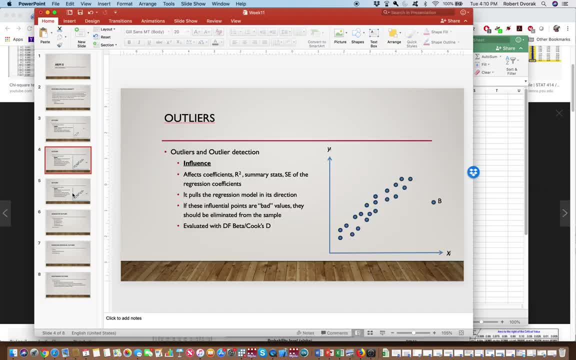 give you the intercept and the slope effects. it just gives you an overall effects. it just gives you an overall effects. it just gives you an overall effect. so I have the same thing there- effect. so I have the same thing there- effect. so I have the same thing there. let's open this back up. all right, let's. 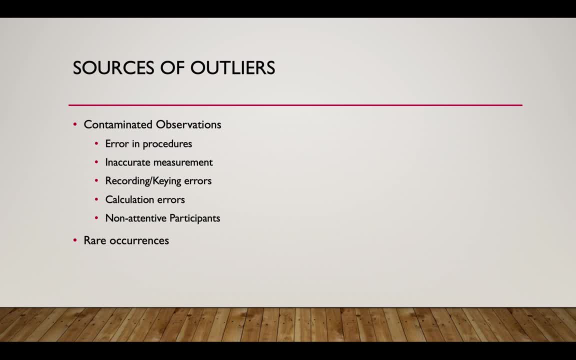 let's open this back up, all right, let's let's open this back up, all right. let's talk a little bit about sources of talk a little bit about sources of talk a little bit about sources of outliers, so they can come from all sorts outliers, so they can come from all sorts. 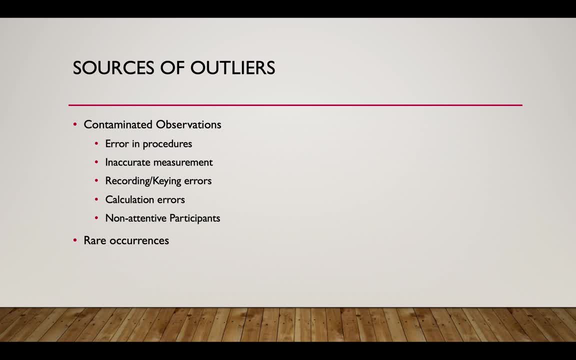 outliers so they can come from all sorts of issues. remember I said that this is a of issues. remember I said that this is a of issues. remember I said that this is a messy data problem. usually these come messy data problem. usually these come messy data problem. usually these come from some sort of contamination in our 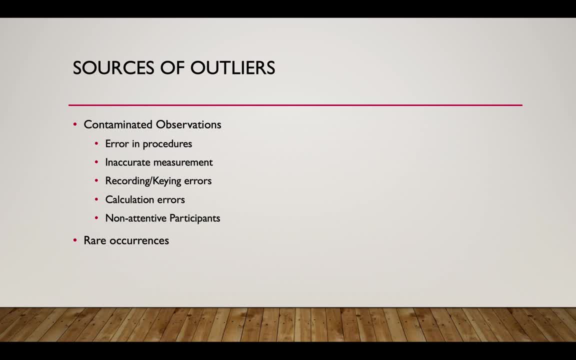 from some sort of contamination in our, from some sort of contamination in our observations. it can be an error in our observations. it can be an error in our observations. it can be an error in our procedures, a problem with how we procedures, a problem with how we procedures, a problem with how we collected the data, and that falls on us. 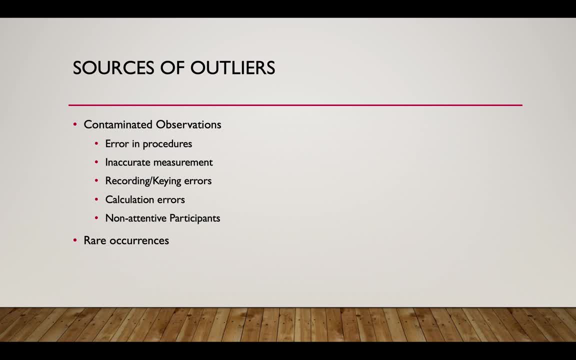 collected the data and that falls on us: collected the data and that falls on us. it can come from inaccurate measurements. it can come from inaccurate measurements. it can come from inaccurate measurements, so, for example, if you have poor so, for example, if you have poor. so, for example, if you have poor reliability or validity, but especially 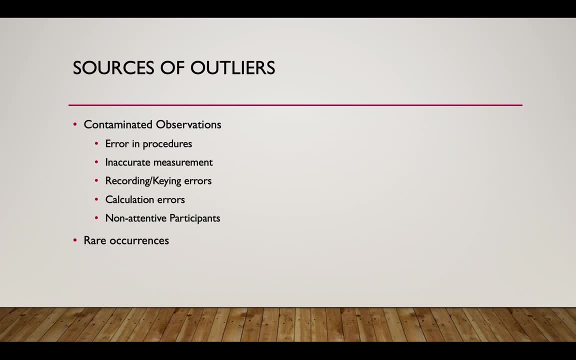 reliability or validity, but especially reliability, or validity, but especially reliability. think about if you've got reliability. think about if you've got reliability. think about if you've got people coming in that are getting on a people coming in that are getting on a people coming in that are getting on a scale, and that scale is not very. 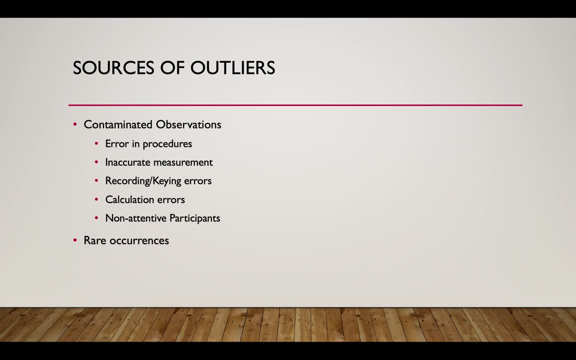 scale and that scale is not very scale and that scale is not very accurate. you can get a really messy data accurate. you can get a really messy data accurate. you can get a really messy data. or possibly there is something going on, or possibly there is something going on. 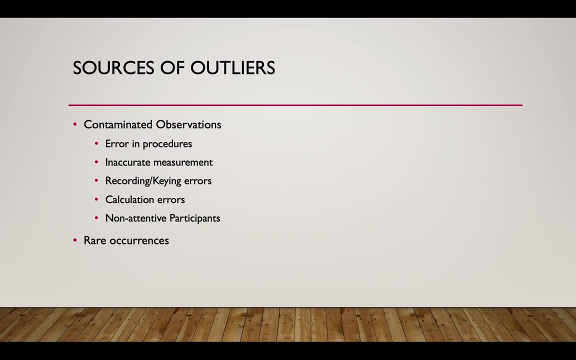 or possibly there is something going on where a person puts their hand on the, where a person puts their hand on the, where a person puts their hand on the table as they step on the scale and you table as they step on the scale and you table as they step on the scale and you don't get an accurate measure of their 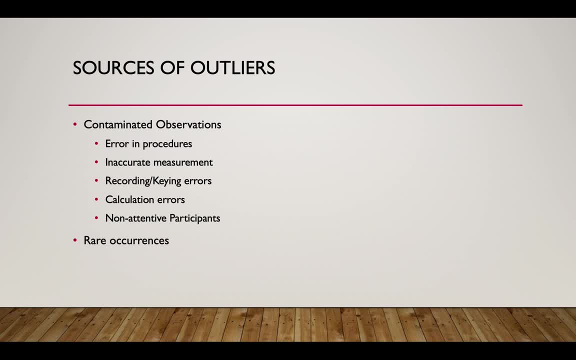 don't get an accurate measure of their, don't get an accurate measure of their weight. regardless, you wind up having weight regardless. you wind up having weight regardless. you wind up having either an error in the procedure or some. either an error in the procedure or some. either an error in the procedure or some sort of inaccuracy in the measurement. 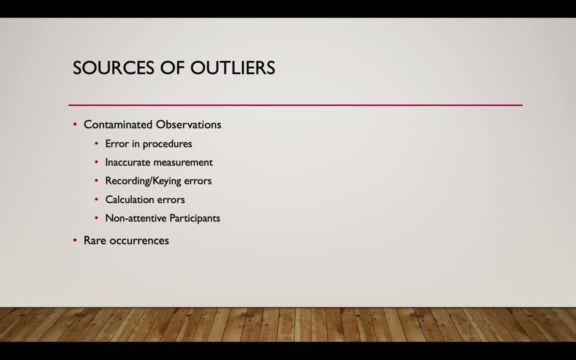 sort of inaccuracy in the measurement, sort of inaccuracy in the measurement, recording or keying errors. you know if recording or keying errors. you know if recording or keying errors. you know if you're using paper and pencil measures. you're using paper and pencil measures. 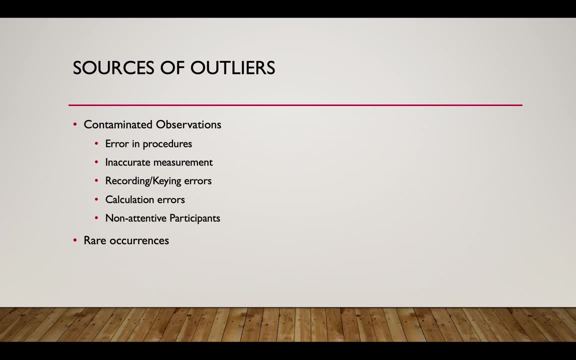 you're using paper and pencil measures and people are just plugging data into and people are just plugging data into and people are just plugging data into papers and pencils, or plugging data into papers and pencils, or plugging data into papers and pencils or plugging data into the computer after it's been copied on. 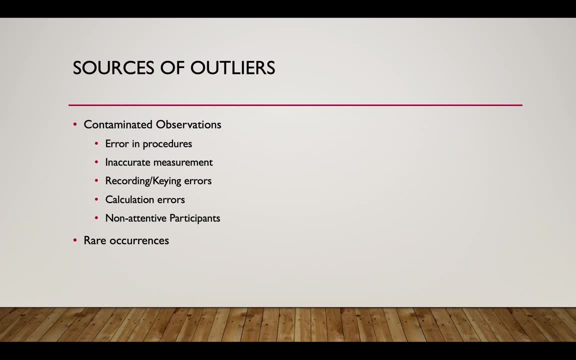 the computer after it's been copied on the computer, after it's been copied on paper or pencil, it can be problematic, paper or pencil, it can be problematic. paper or pencil, it can be problematic. you can have all kinds of recording. or you can have all kinds of recording or 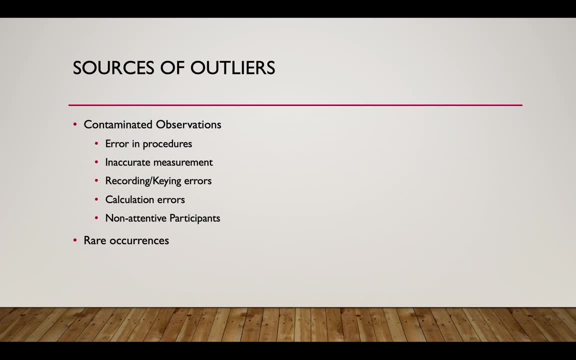 you can have all kinds of recording or keying errors. this becomes a real issue. keying errors: this becomes a real issue. keying errors: this becomes a real issue when you're using undergraduate research, when you're using undergraduate research, when you're using undergraduate research assistants to enter your data. there can. 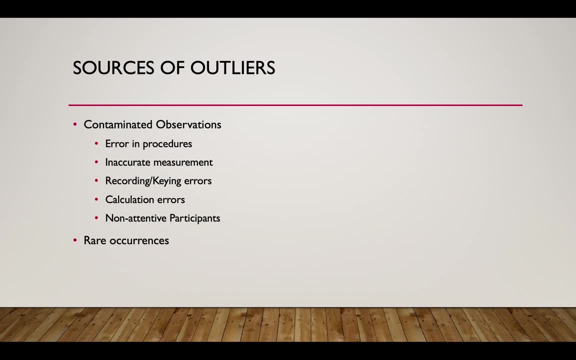 assistants to enter your data. there can assistants to enter your data. there can also be problems with calculation errors also be problems with calculation errors also be problems with calculation errors. so some of the stuff that we do with our. so some of the stuff that we do with our. 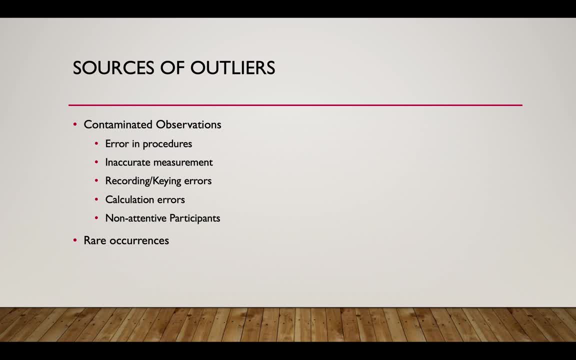 so some of the stuff that we do with our data, is we wind up making some sort of data? is we wind up making some sort of data? is we wind up making some sort of transformation or adding something, or transformation, or adding something, or transformation, or adding something or multiplying something, and so it's. 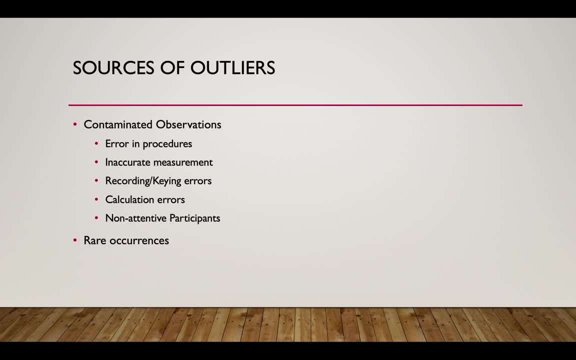 multiplying something, and so it's multiplying something, and so it's possible. in fact, just just yesterday, I possible, in fact, just just yesterday, I possible. in fact, just just yesterday, I was meeting with Sarah and we were was meeting with Sarah and we were was meeting with Sarah and we were trying to work through a calculation. 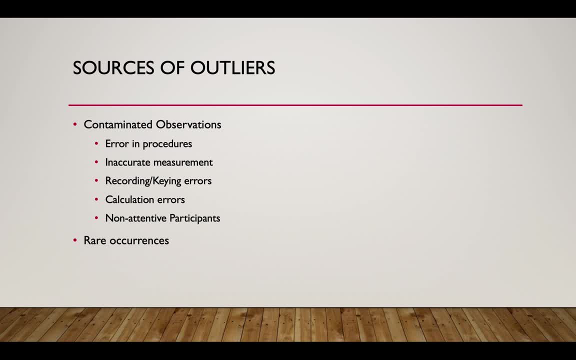 trying to work through a calculation, trying to work through a calculation error and we eventually figured it out- error and we eventually figured it out- error and we eventually figured it out. but it you can, you can run into these. but it you can, you can run into these. 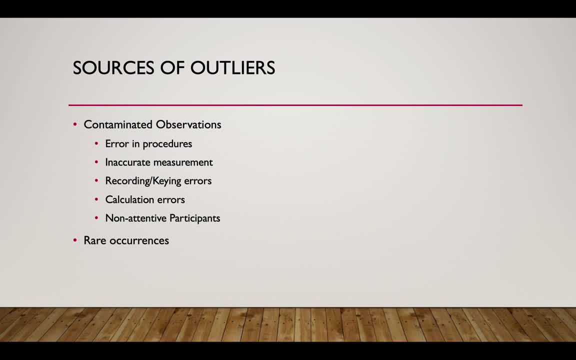 but it you can, you can run into these issues and this can help you identify issues and this can help you identify issues and this can help you identify. going through and looking at your, your going through and looking at your. your going through and looking at your, your influence, your leverage, can help you. 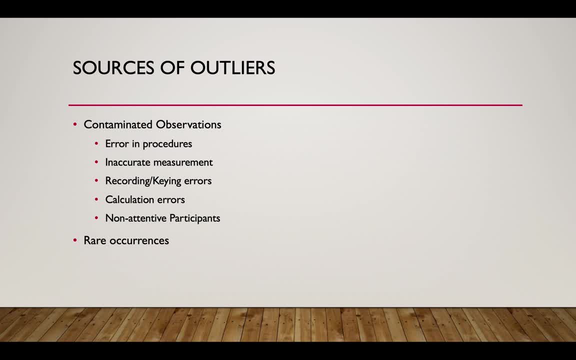 influence your leverage. can help you influence your leverage. can help you identify if you've made a calculation. identify if you've made a calculation. identify if you've made a calculation error or if it's a true error in your error or if it's a true error in your. 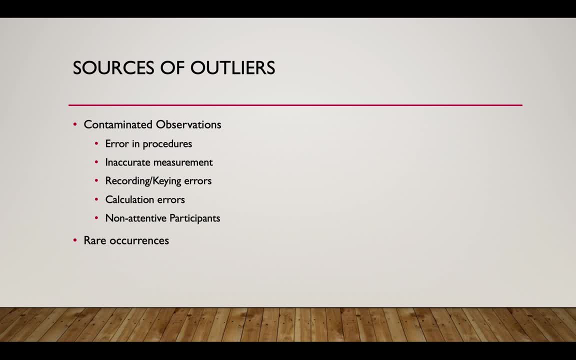 error or if it's a true error in your data, and then just kind of non-attentive data and then just kind of non-attentive data and then just kind of non-attentive participants- right, people that are just participants, right? people that are just. 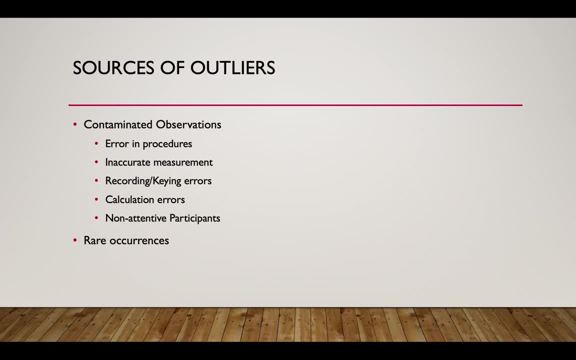 participants, right, people that are just going along plugging in any answer, that going along plugging in any answer, that going along plugging in any answer that they want, not paying attention to what they want, not paying attention to what they want, not paying attention to what they're doing. another possible source is: 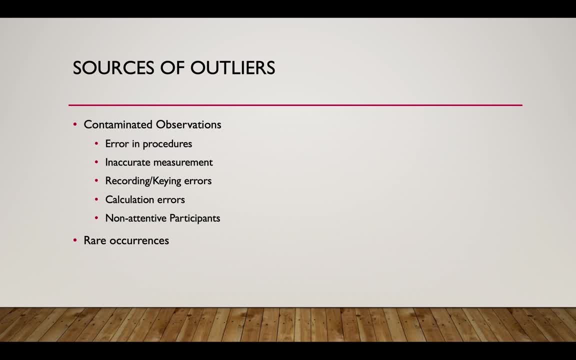 they're doing. another possible source is they're doing. another possible source is rare occurrences. so I can tell you that rare occurrences. so I can tell you that rare occurrences. so I can tell you that, as someone who does substance use, as someone who does substance use, as someone who does substance use, research, this happens, this happens. I 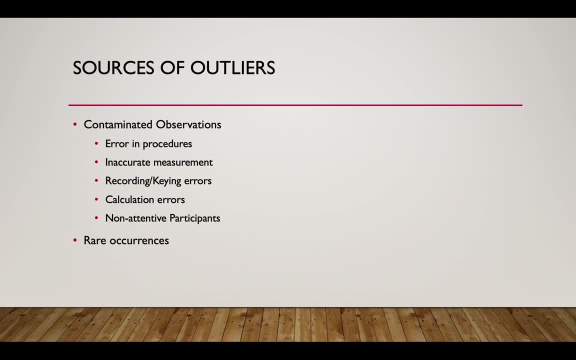 research. this happens. this happens. I research, this happens. this happens. I have a bunch of people who will drink on. have a bunch of people who will drink on. have a bunch of people who will drink on average two or three or four drinks a average two or three or four drinks a. 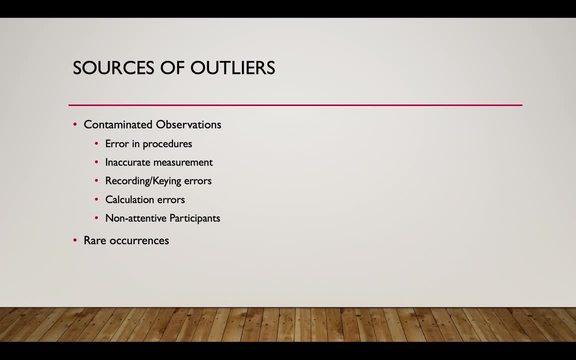 average two or three or four drinks a night, and then I have that one person night, and then I have that one person night, and then I have that one person that drinks 27 drinks on a given night, that drinks 27 drinks on a given night, that drinks 27 drinks on a given night right, and oftentimes this person is- is a. 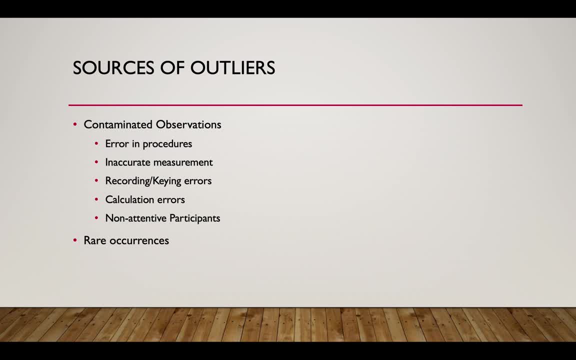 right, and oftentimes this person is is a right, and oftentimes this person is is a, an imp or a leveraged person, but not an. an imp or a leveraged person, but not an- an imp or a leveraged person, but not an influence person. and so I'll see them. 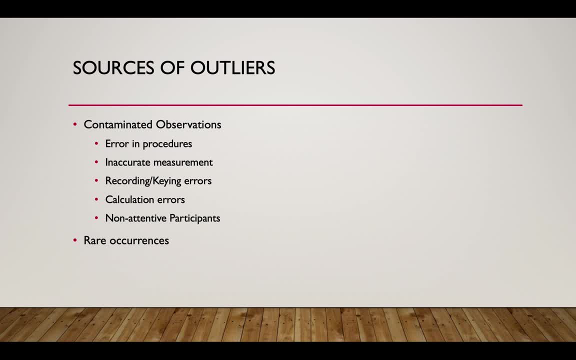 influence person, and so I'll see them influence person, and so I'll see them fitting on the line where they're fitting on the line where they're fitting on the line where they're supposed to be but accounting for, or supposed to be but accounting for, or 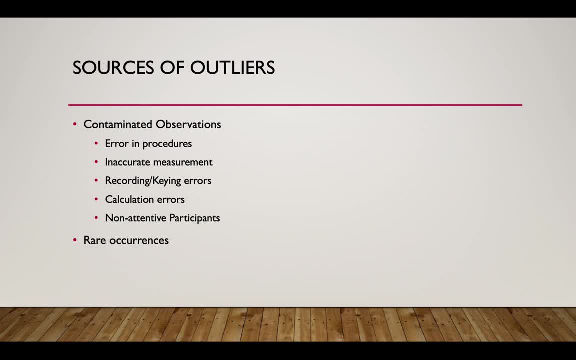 supposed to be, but accounting for or resulting in substantially more, are resulting in substantially more, are resulting in substantially more, are squared than what I should have, because squared than what I should have, because squared than what I should have because of that person. so how do we do it? what? 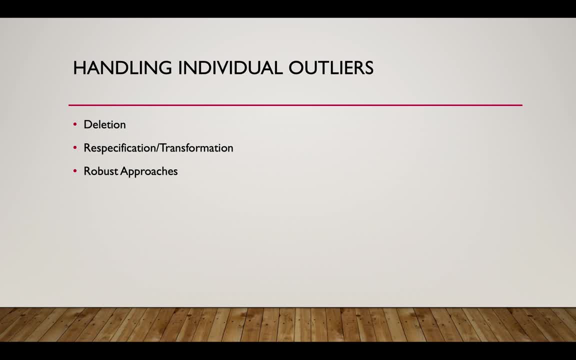 of that person. so how do we do it? what of that person? so how do we do it? what do we do? how do we handle these? well, we do we do. how do we handle these well, we do we do. how do we handle these? well, we can do a few different things. the 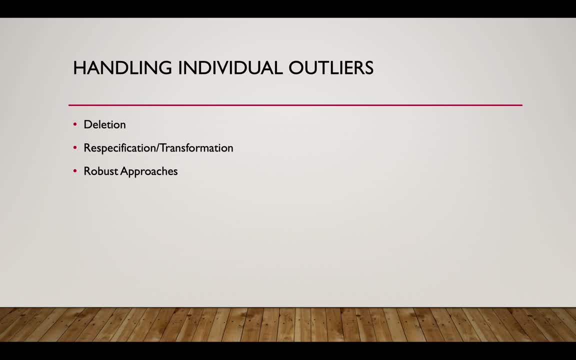 can do a few different things. the can do a few different things. the easiest and most common way to handle an easiest and most common way to handle an easiest and most common way to handle an outlier is to just delete them of outlier is to just delete them of. 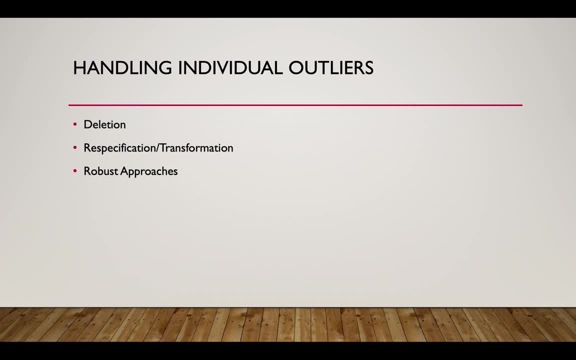 outlier is to just delete them. of course this is a problem. because you course this is a problem. because you course this is a problem. because you want to have, you're always trying to want to have, you're always trying to want to have, you're always trying to strike a balance between giving the best. 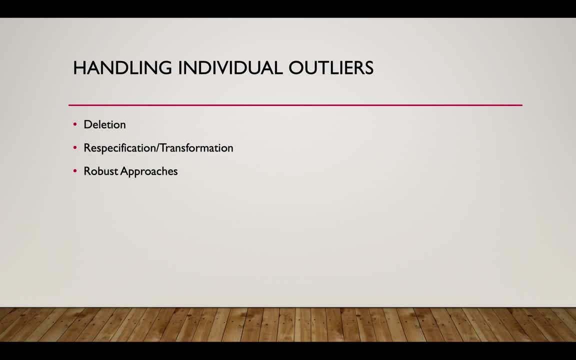 strike a balance between giving the best strike, a balance between giving the best possible explanation of what's going on, possible explanation of what's going on, possible explanation of what's going on in the population and having to explain in the population, and having to explain in the population and having to explain, or an ex having an explanatory model. 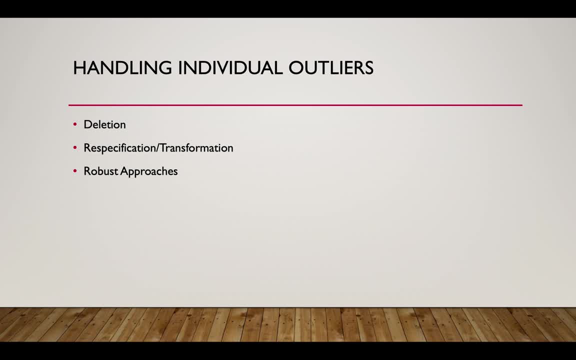 or an ex having an explanatory model or an ex having an explanatory model that accounts for these rare occurrences. that accounts for these rare occurrences. that accounts for these rare occurrences. if you're able to identify that it's a. if you're able to identify that it's a. 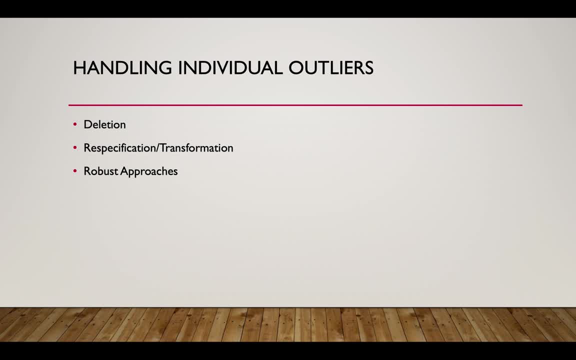 if you're able to identify that it's a rare occurrence, you have to make a rare occurrence. you have to make a rare occurrence. you have to make a judgment call about what you want to do. judgment call about what you want to do. judgment call about what you want to do with that observation if you pull it out. 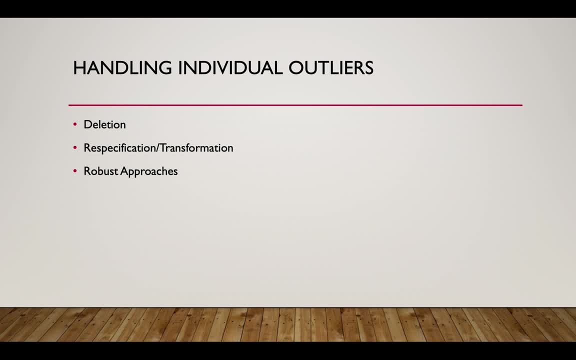 with that observation, if you pull it out, with that observation, if you pull it out, you will lose some of the explanatory. you will lose some of the explanatory, you will lose some of the explanatory power of your model and that could have power of your model and that could have 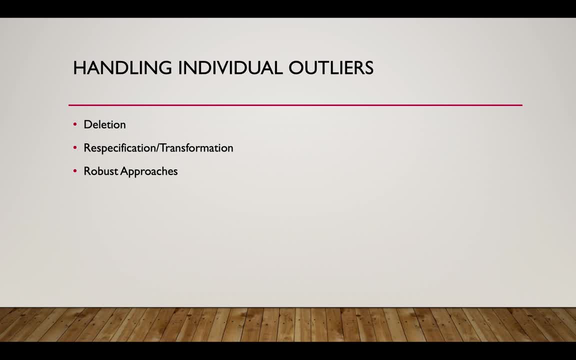 power of your model and that could have real-world implications, especially if real-world implications, especially if real-world implications, especially if that rare occurrence is- is important, if that rare occurrence is is important, if that rare occurrence is is important, if you leave it in and it's not a true rare. 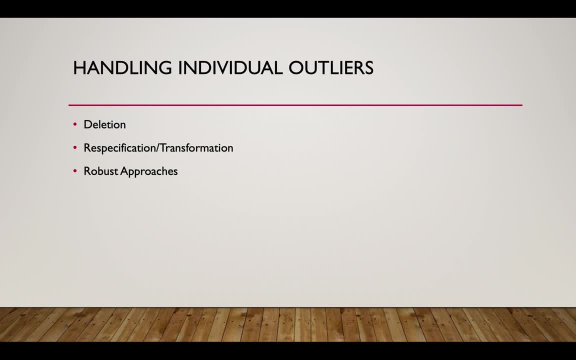 you leave it in and it's not a true rare. you leave it in and it's not a true rare occurrence. it can lead to model occurrence. it can lead to model occurrence. it can lead to model specification. it winds up being a specification. it winds up being a. 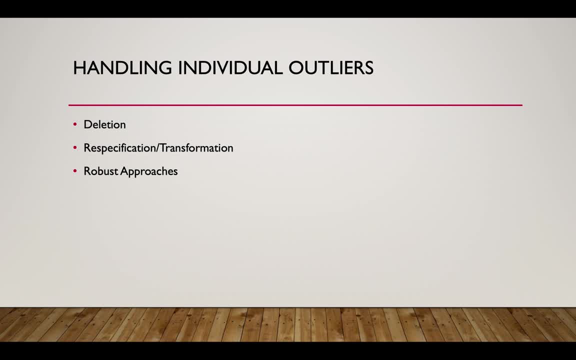 specification, it winds up being a researcher call. either way, the important researcher call. either way, the important researcher call. either way, the important thing is that you talk through what you thing is that you talk through what you thing is that you talk through what you did. you present your data and you make. 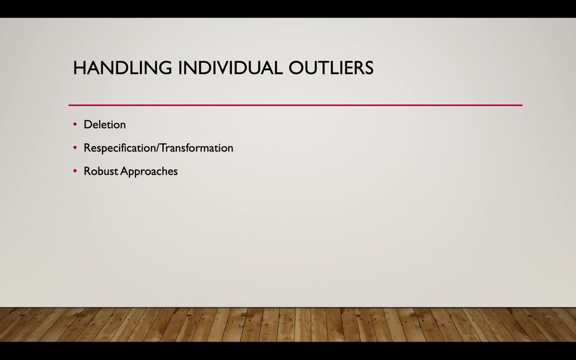 did you present your data and you make, did you present your data and you make sure that at least in the footnotes, if sure that, at least in the footnotes, if sure that at least in the footnotes, if not in the text explicitly, it says this: 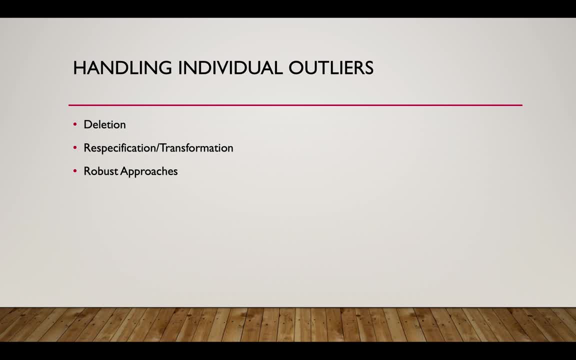 not in the text explicitly. it says this not in the text explicitly. it says this is what things look like with and is what things look like with, and is what things look like with and without that observation, and this is without that observation and this is without that observation, and this is called sensitivity and specificity, and 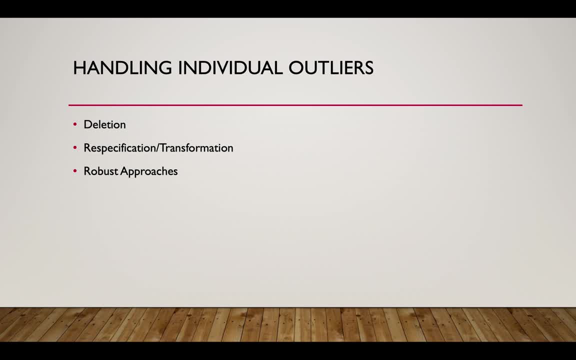 called sensitivity and specificity, and called sensitivity and specificity, and so it's important to discuss the, so it's important to discuss the, so it's important to discuss the sensitivity and specificity of your model, sensitivity and specificity of your model, sensitivity and specificity of your model in the context of influence and. 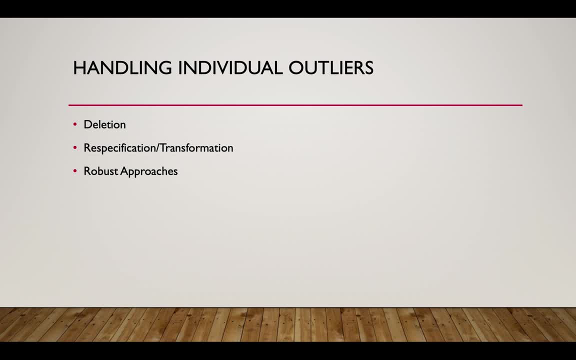 in the context of influence, and in the context of influence and leverage- sorry the another possibility, leverage. sorry the another possibility, leverage. sorry. the another possibility is re specification and or is re specification and or is re specification and or transformations. we've talked a little bit transformations: we've talked a little bit. 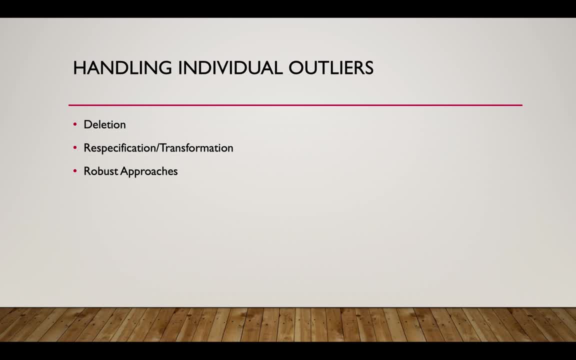 transformations. we've talked a little bit about transformations in the past. if you about transformations in the past, if you about transformations in the past, if you have data that is becoming heavily have, data that is becoming heavily have, data that is becoming heavily skewed and it is resulting in influence. 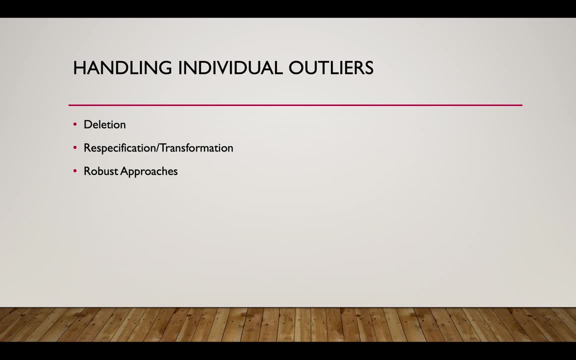 skewed and it is resulting in influence. skewed and it is resulting in influence or leverage you may want to think about, or leverage. you may want to think about or leverage, you may want to think about doing some sort of data transformation, doing some sort of data transformation, doing some sort of data transformation. this is a this is a good, solid reason. 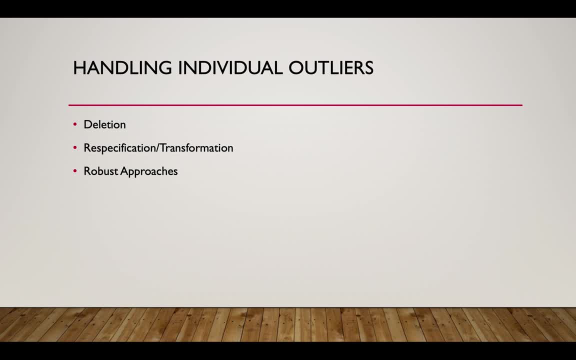 this is a. this is a good, solid reason. this is a. this is a good, solid reason for a data transformation outside of the, for a data transformation outside of the, for a data transformation outside of the potential for an inaccurate distribution, potential for an inaccurate distribution, potential for an inaccurate distribution of residuals or homogeneous. I'm sorry. 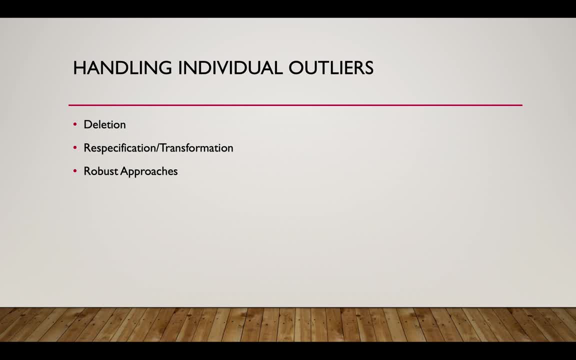 of residuals or homogeneous, I'm sorry. of residuals or homogeneous, I'm sorry. distribution of residuals, so you might. distribution of residuals, so you might. distribution of residuals, so you might have skewed data. you might do a an have skewed data. you might do a an have skewed data. you might do a, an examination of your residuals and find. 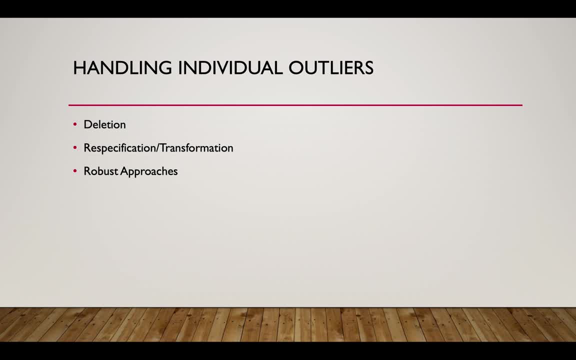 examination of your residuals and find examination of your residuals and find that your residuals are normally, that your residuals are normally, that your residuals are normally distributed, despite the fact that your distributed, despite the fact that your distributed, despite the fact that your data is skewed, however, that skew and 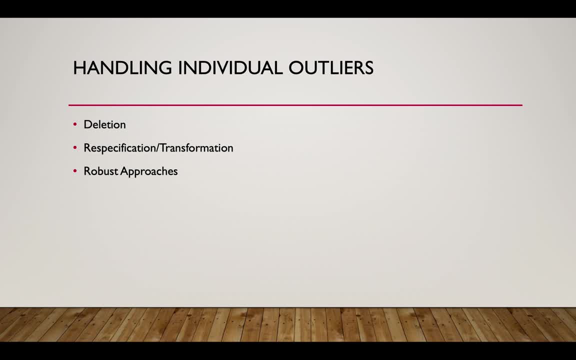 data is skewed, however that skew, and data is skewed, however that skew, and your data results in high influence and your data results in high influence and your data results in high influence and or high leverage, and consequently, higher or high leverage, and consequently, higher or high leverage, and consequently, higher R squared. it may be worth transforming. 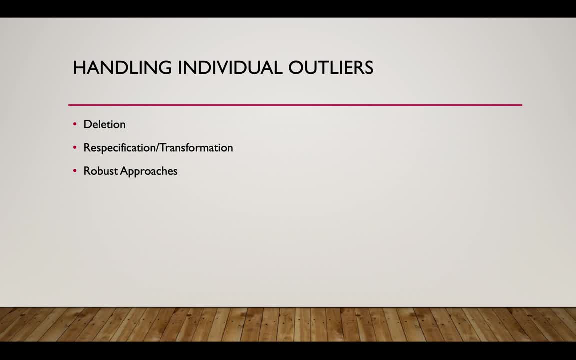 R squared. it may be worth transforming R squared. it may be worth transforming that data to make a more comprehensive that data, to make a more comprehensive that data, to make a more comprehensive model. finally, one thing that I really model, finally, one thing that I really like doing, is using more robust. 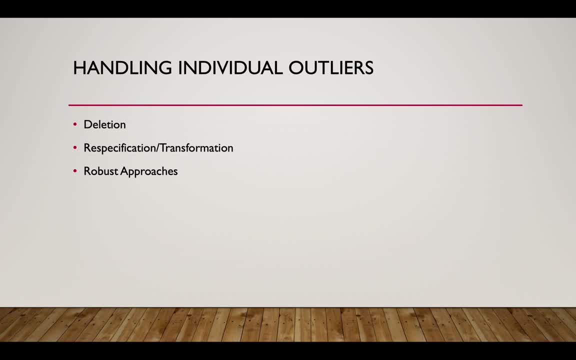 like doing is using more robust. like doing is using more robust approaches. some of these involve doing approaches. some of these involve doing approaches. some of these involve doing things like Windsor ring, where you chop things like Windsor ring. where you chop things like Windsor ring, where you chop off portions of standard deviations at 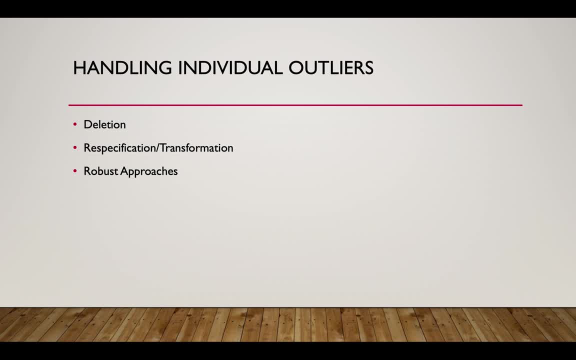 off portions of standard deviations at off portions of standard deviations at the extremes. or you use things like the extremes or you use things like the extremes. or you use things like negative binomial models or gamma negative binomial models or gamma negative binomial models or gamma district distributed outcome models. these 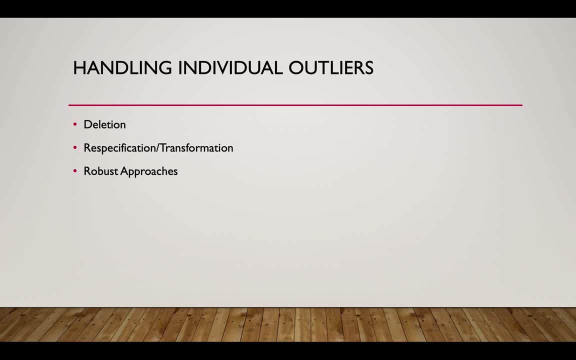 district distributed outcome models. these district distributed outcome models, these are models that still fall within the, are models that still fall within the, are models that still fall within the generalized linear model framework, which generalized linear model framework, which generalized linear model framework, which is the same as OLS, the same as 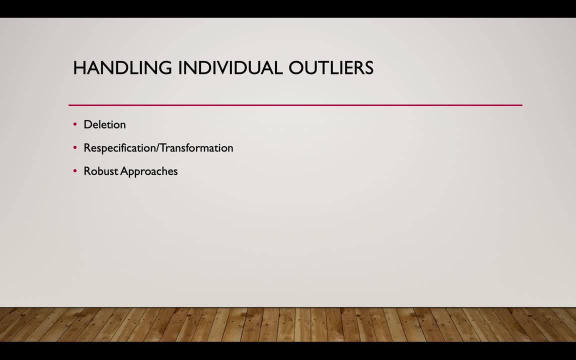 is the same as OLS, the same as is the same as OLS, the same as regression and ANOVA, but they allow for regression and ANOVA. but they allow for regression and ANOVA, but they allow for a more robust understanding of both. 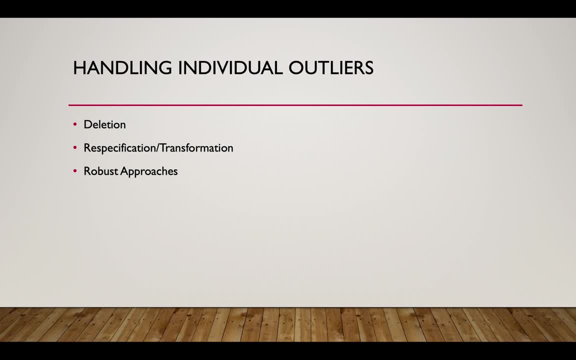 a more robust understanding of both. a more robust understanding of both- predictors and of outcomes. some of the predictors and of outcomes. some of the predictors and of outcomes. some of the ways that you can handle outcomes is by ways that you can handle outcomes is by ways that you can handle outcomes is by changing the outcomes to negative. 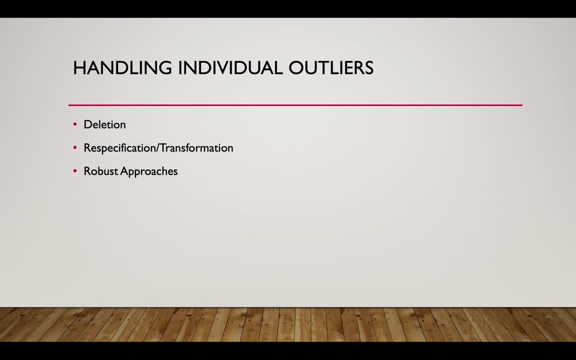 changing the outcomes to negative. changing the outcomes to negative, binomial or gamma or so on. as I said, binomial or gamma or so on. as I said, binomial or gamma or so on. as I said, some of the ways you can handle, some of the ways you can handle. 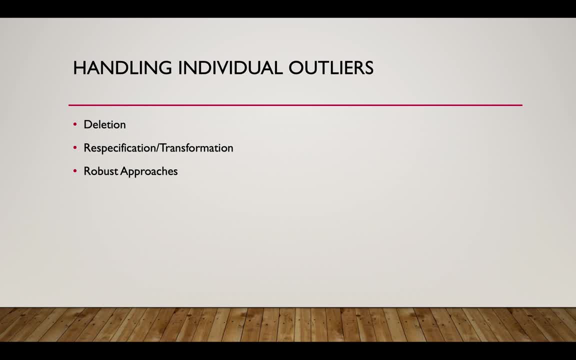 some of the ways you can handle predictors is by utilizing things like predictors is by utilizing things like predictors is by utilizing things like bootstrapping to recalculate your bootstrapping, to recalculate your bootstrapping to recalculate your standard errors and or a jackknife. 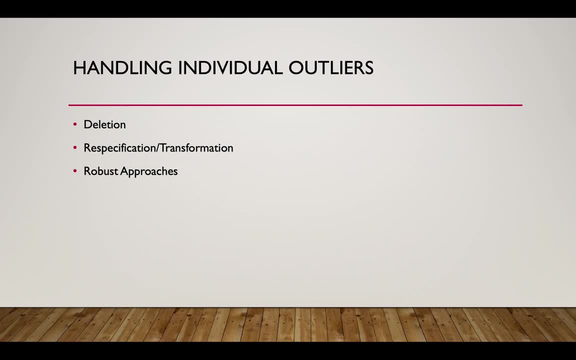 standard errors and or a jackknife standard errors and or a jackknife approach to get more appropriate approach to get more appropriate approach to get more appropriate standard errors, or using simple bias standard errors, or using simple bias standard errors or using simple bias correction methods that we see. 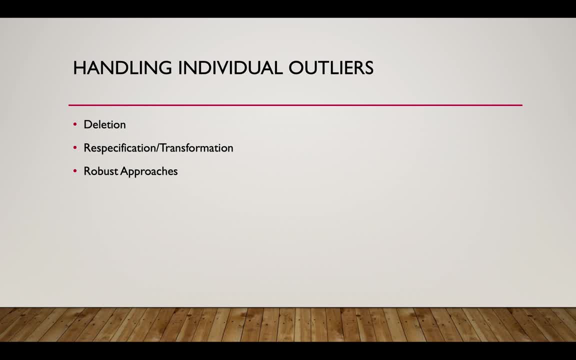 correction methods that we see, correction methods that we see, oftentimes in maximum likelihood, oftentimes in maximum likelihood, oftentimes in maximum likelihood, estimation- all right. so that's estimation all right. so that's estimation all right. so that's, that is how we can handle individual. that is how we can handle individual. 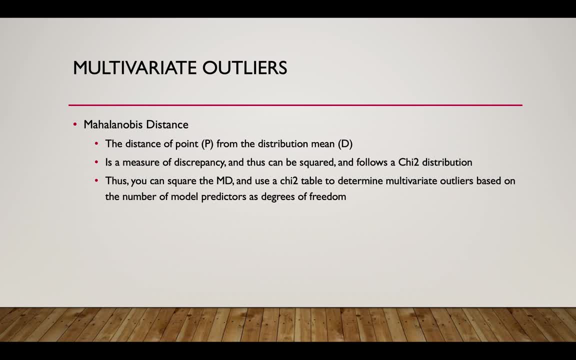 that is how we can handle individual outliers, however, sometimes the case is outliers. however, sometimes the case is outliers. however, sometimes the case is that we have multivariate outliers and that we have multivariate outliers and that we have multivariate outliers and multivariate outliers. the the most. 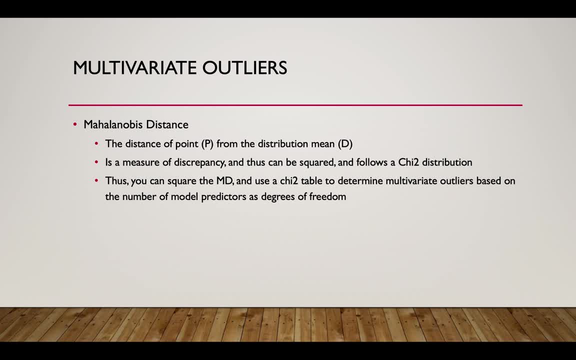 multivariate outliers: the the most multivariate outliers, the the most common way to at least test for common way to at least test for common way to at least test for multivariate outliers is to use my multivariate outliers, is to use my multivariate outliers, is to use my halinobis distance. that I say it's the. 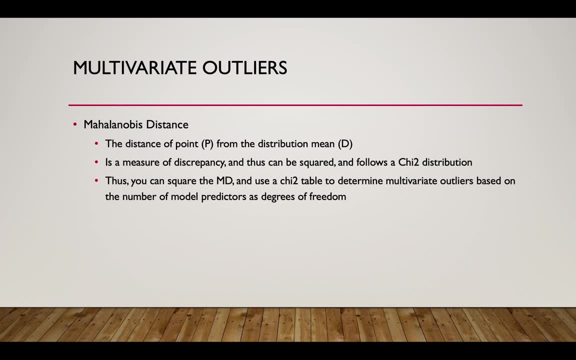 halinobis distance. that I say it's the halinobis distance. that I say it's the most common way. I say I say it's the most common way. I say I say it's the most common way. I say I say it's the most common way for people who use SPSS. 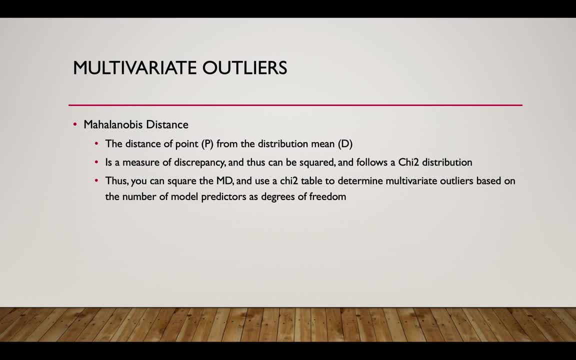 most common way for people who use SPSS, most common way for people who use SPSS, and so this is what I'm going to teach, and so this is what I'm going to teach, and so this is what I'm going to teach you guys. my halinobis distance is the. 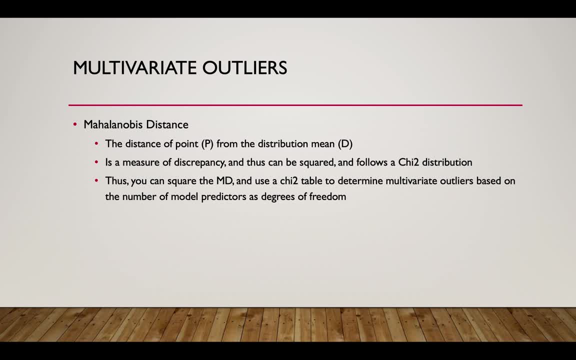 you guys, my halinobis distance is the. you guys, my halinobis distance is the distance of a point and the point being distance of a point and the point being distance of a point and the point being any given observation, any given person. any given observation, any given person. 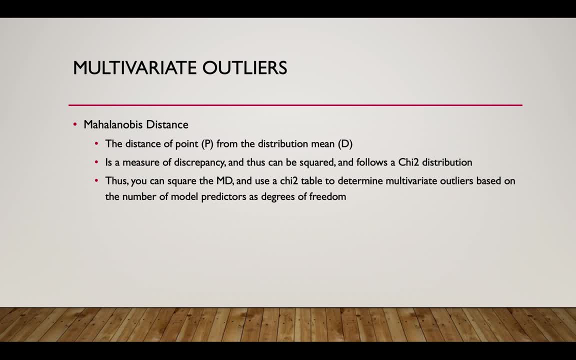 any given observation, any given person, from the total distribution of the mean, from the total distribution of the mean, from the total distribution of the mean of your data cloud in your, in your full of your data cloud, in your, in your full of your data cloud, in your, in your full regression model. this is your really. 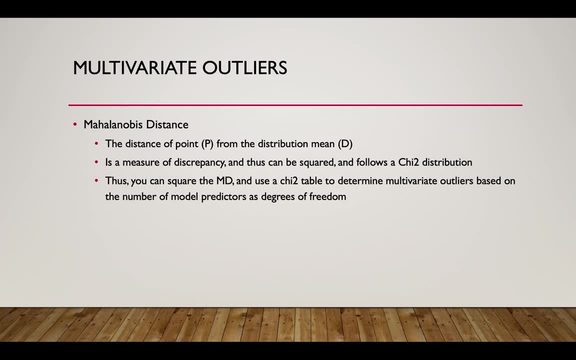 regression model. this is your really regression model. this is your really your data cloud of residuals. it is a your data cloud of residuals. it is a your data cloud of residuals. it is a measure of discrepancy that takes into measure of discrepancy, that takes into measure of discrepancy that takes into account all of the model predictors and 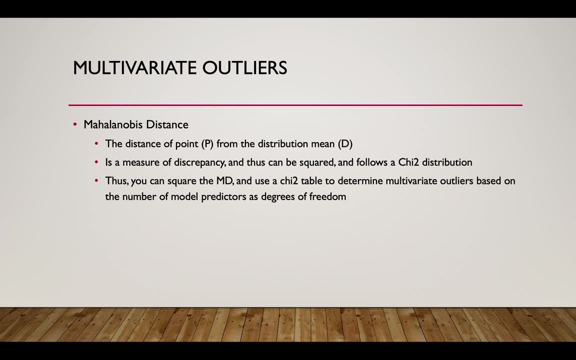 account all of the model predictors and account all of the model predictors, and I want you to keep in mind that all of I want you to keep in mind, that all of I want you to keep in mind that all of those model predictors wind up being a. 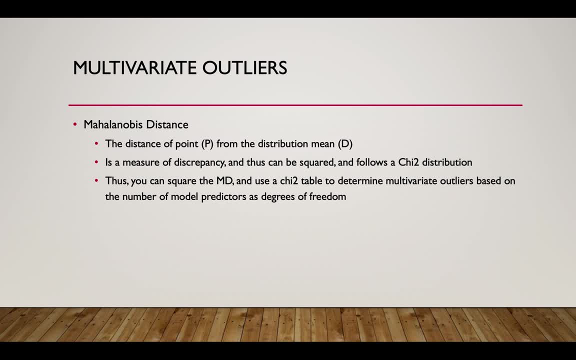 those model predictors wind up being a. those model predictors wind up being a degree of freedom for each predictor. degree of freedom for each predictor within the context of this discrepancy, within the context of this discrepancy, within the context of this discrepancy or this distance measure, and so this, 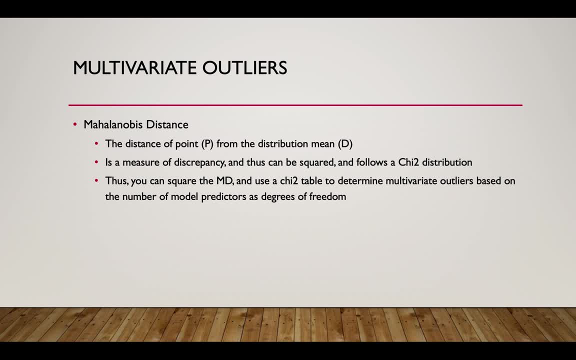 or this distance measure, and so this or this distance measure, and so this distance measure winds up following a distance measure, winds up following a distance measure, winds up following a chi-square distribution. when that, that chi-square distribution, when that that chi-square distribution, when that that discrepancy is squared, we're gonna hop. 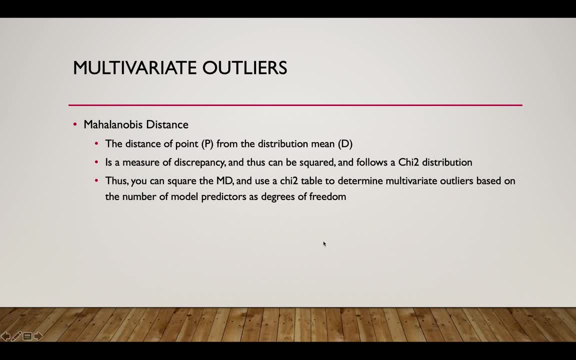 discrepancy is squared. we're gonna hop. discrepancy is squared. we're gonna hop over to SPSS in just a moment and we're over to SPSS in just a moment. and we're over to SPSS in just a moment and we're gonna look at squaring it in order to do. 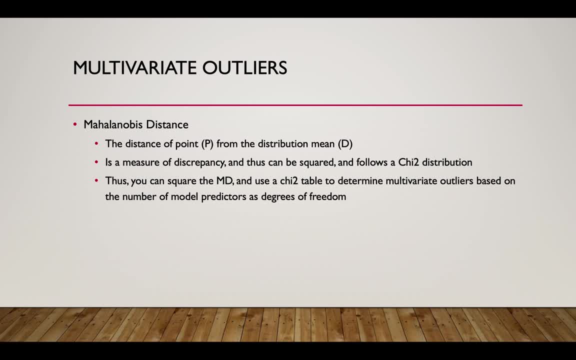 gonna look at squaring it in order to do. gonna look at squaring it in order to do this, but what? what it ultimately means this, but what? what it ultimately means this, but what? what it ultimately means is: you can square Mahalan obis distance is you can square Mahalan obis distance. 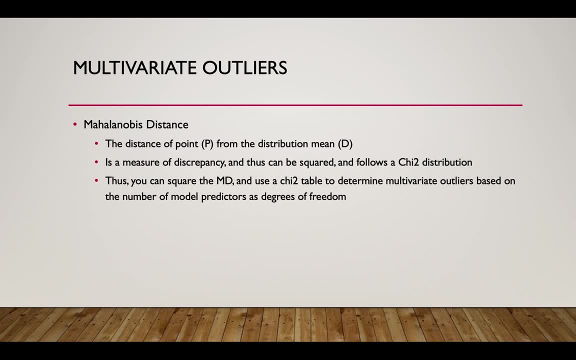 is. you can square Mahalan obis distance. use a chi-square table to determine if. use a chi-square table to determine if. use a chi-square table to determine if your multivariate outliers are in your multivariate outliers are in. your multivariate outliers are in excess of some sort of degree of freedom. so 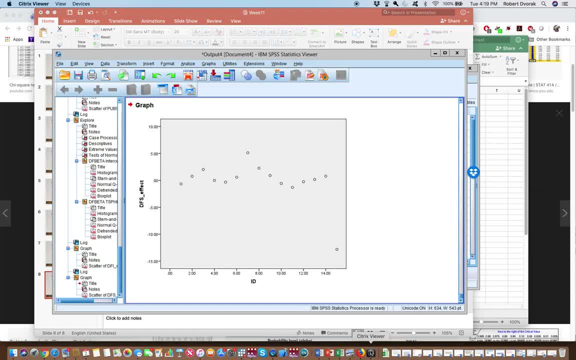 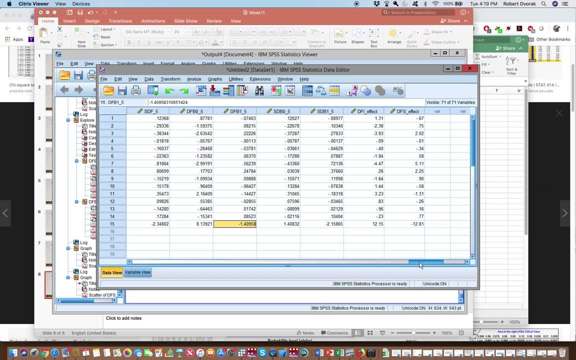 excess of some sort of degree of freedom. so excess of some sort of degree of freedom. so let's do this. let's look at SPSS and let's do this. let's look at SPSS and let's do this. let's look at SPSS and let's. we're gonna leave all of those in. 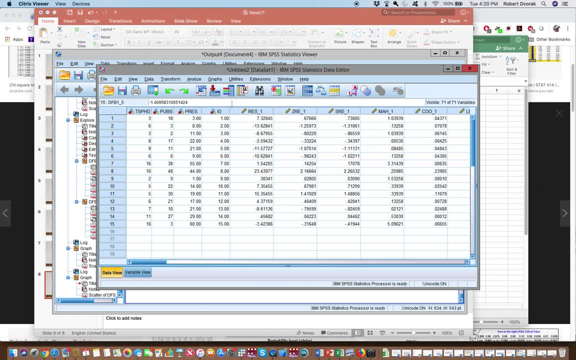 let's, we're gonna leave all of those in there for right now. the way that you get there for right now, the way that you get there for right now, the way that you get Mahalan obis distance, I'm going to Mahalan obis distance. I'm going to. 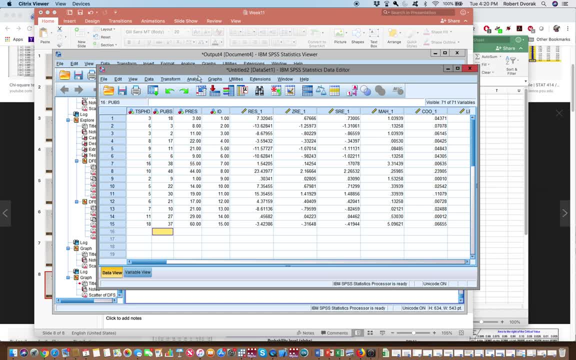 Mahalan obis distance. I'm going to change this back to 37, which is what it change this back to 37, which is what it change this back to 37, which is what it was before you can go analyze regression. was before you can go analyze regression. 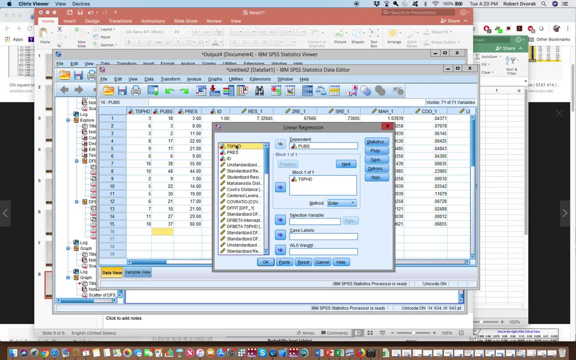 was before. you can go analyze regression- linear and we are going to add linear. and we are going to add linear and we are going to add presentations as another predictor. now we presentations as another predictor. now we presentations as another predictor. now we have multiple predictors in the model. we 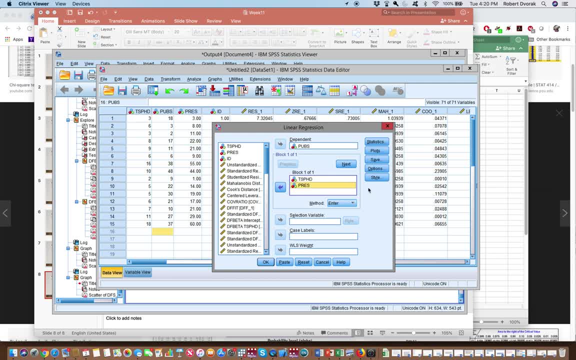 have multiple predictors in the model. we have multiple predictors in the model. we have a multivariate model. before we only have a multivariate model. before we only had a univariate model or a simple had a univariate model or a simple had a univariate model or a simple bivariate model, where we didn't actually 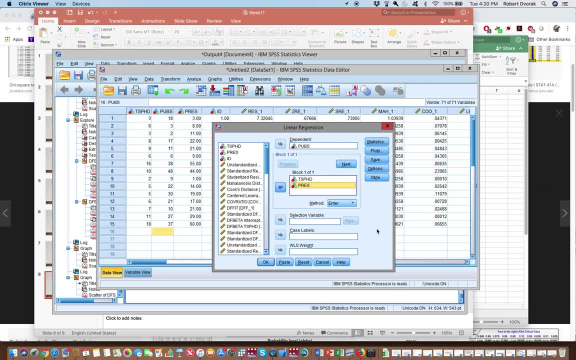 bivariate model where we didn't actually bivariate model where we didn't actually have the Mahalan obis distance under. have the Mahalan obis distance under, have the Mahalan obis distance under. that specification will be very, very, that specification will be very, very. 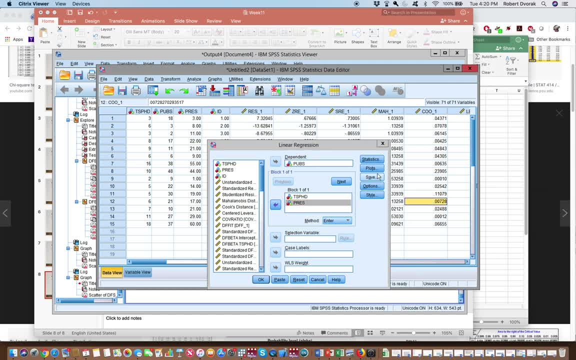 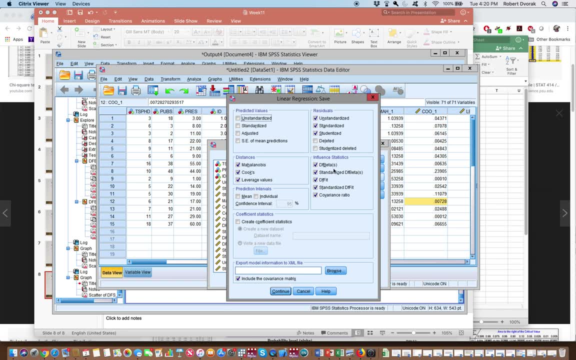 that specification will be very, very close to a simple leverage statistic. if close to a simple leverage statistic, if close to a simple leverage statistic, if we now change it to this: oops and we go. we now change it to this: oops and we go. we now change it to this: oops and we go save and we select Mahalan obis distance. save and we select Mahalan obis distance. save and we select Mahalan obis distance. we've already looked at cooks and we've we've already looked at cooks and we've we've already looked at cooks and we've looked at leverage, so now we're gonna. 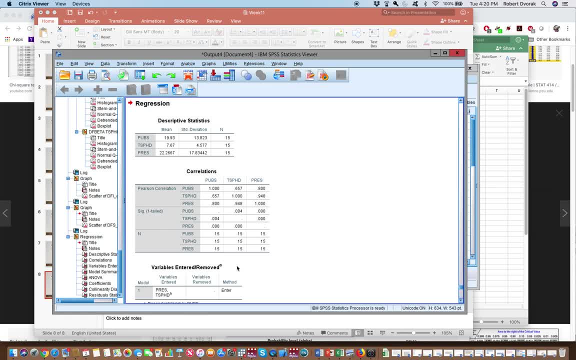 looked at leverage. so now we're gonna looked at leverage. so now we're gonna look at my Helen of assistance. we can go look at my Helen of assistance. we can go look at my Helen of assistance. we can go: okay, let's look at our data again here. 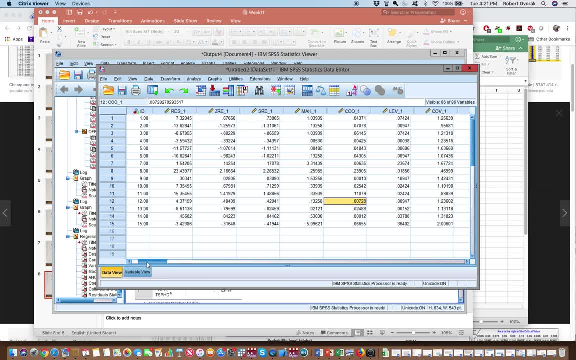 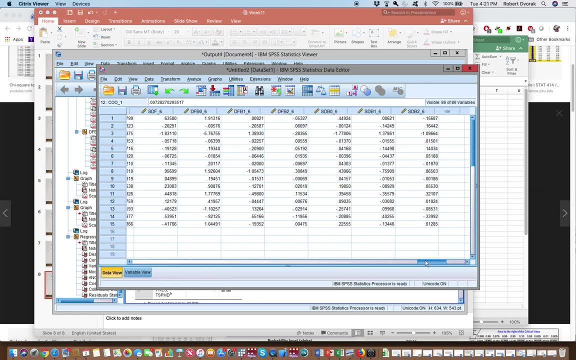 okay, let's look at our data again here. okay, let's look at our data again here: real quick, and so if we come all the way, real quick and so if we come all the way, real quick and so if we come all the way to the end, here are our new values, and 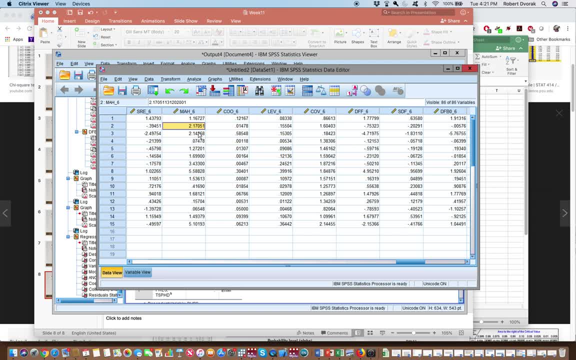 to the end, here are our new values. and to the end, here are our new values. and here's our my Helen of assistance 1.16. here's our my Helen of assistance 1.16. here's our my Helen of assistance 1.16. 2 to 7. we have two extreme Mahalan of. 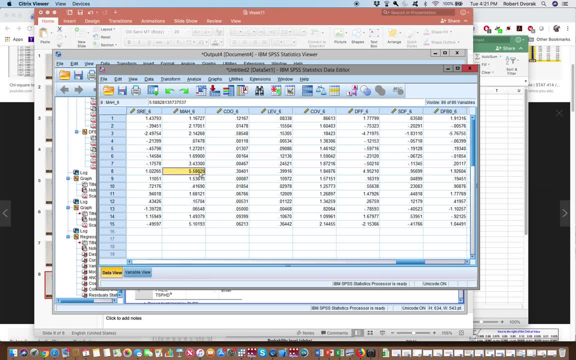 2 to 7. we have two extreme Mahalan of 2 to 7. we have two extreme Mahalan of assistance values: 5.10 and 5.88. and so assistance values 5.10 and 5.88, and so assistance values 5.10 and 5.88. and so if we want to test this to see if these 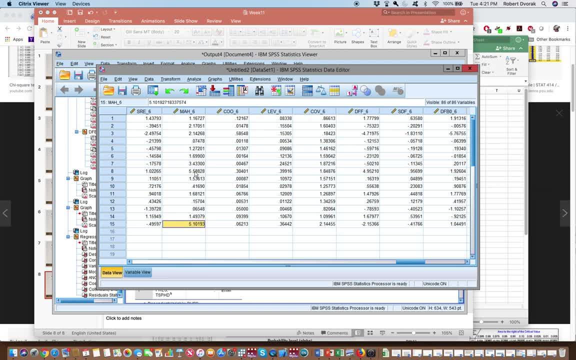 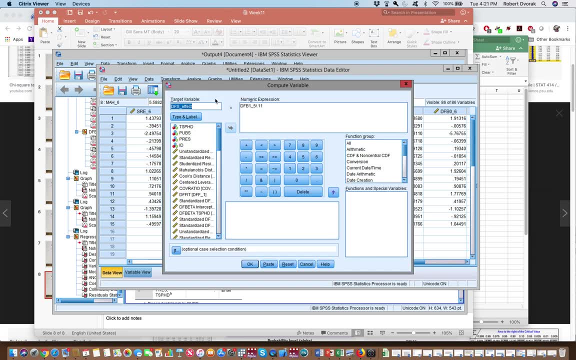 if we want to test this to see if these, if we want to test this to see if these are statistically significant, are statistically significant, are statistically significant multivariate outliers- we can do this, we multivariate outliers. we can do this. we multivariate outliers. we can do this. we can go transform compute. we're gonna. 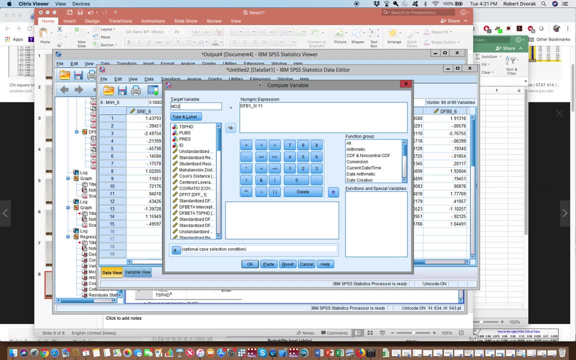 can go transform compute. we're gonna. can go transform compute. we're gonna call this, call this, call this md2 and we're gonna come down here. we're md2 and we're gonna come down here. we're md2 and we're gonna come down here. we're gonna find my Helen Elvis distance. it's. 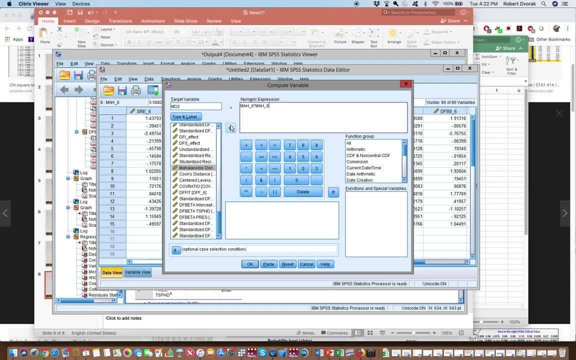 gonna find my Helen Elvis distance. it's gonna find my Helen Elvis distance. it's right there and we are going to square right there and we are going to square right there and we are going to square it, okay, and squaring my Helen Elvis. it okay, and squaring my Helen Elvis. 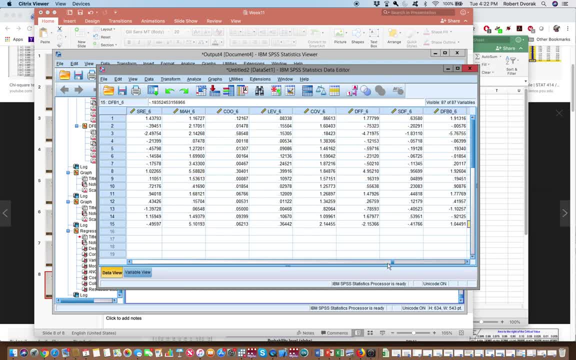 it okay, and squaring my Helen Elvis distance. all it does is add another distance. all it does is add another distance. all it does is add another variable in here for us. it's right here. variable in here for us. it's right here. variable in here for us. it's right here. my Helen Elvis distance squared. and now 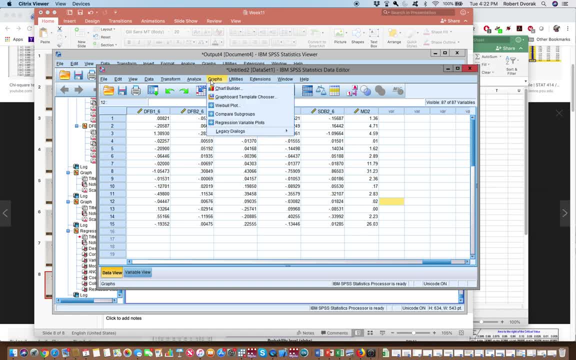 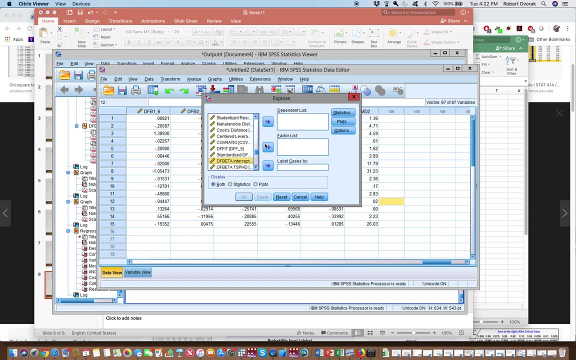 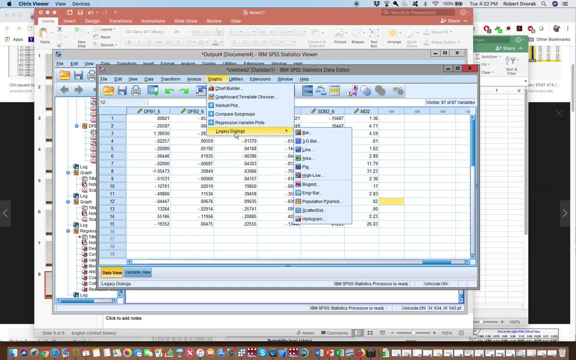 don't even need to do. let's not do that. don't even need to do. let's not do that. let's, let's just grab this for a second. let's, let's just grab this for a second. let's, let's just grab this for a second. let's go legacy dialogues scatter, okay. 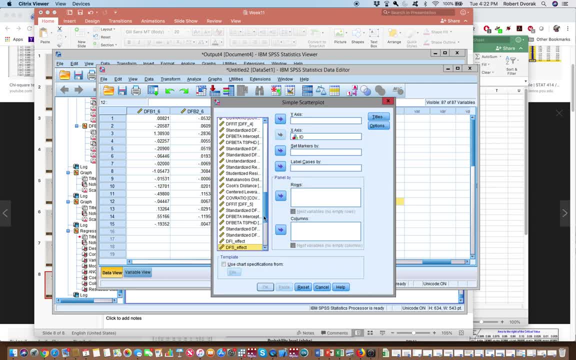 let's go legacy dialogues scatter. okay, let's go legacy dialogues scatter. okay, we're gonna leave ID in there and this, we're gonna leave ID in there and this, we're gonna leave ID in there and this time we're gonna look at the time, we're gonna look at the. 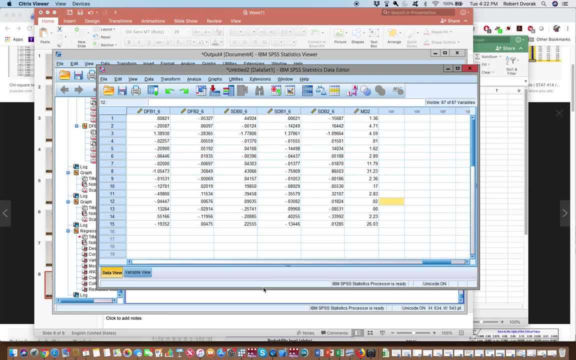 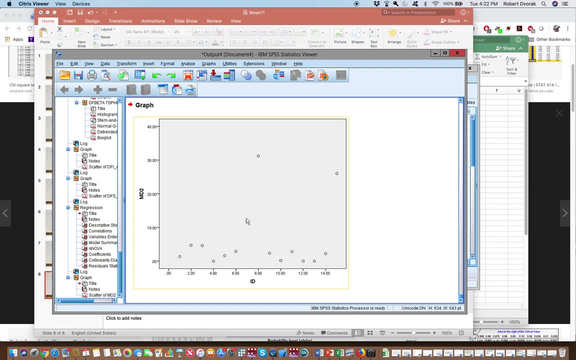 time we're gonna look at the distribution of our chi-squared by distribution of our chi-squared by distribution of our chi-squared by participant. okay, you can see we have participant. okay, you can see we have participant. okay, you can see we have what looked to be like three potential. 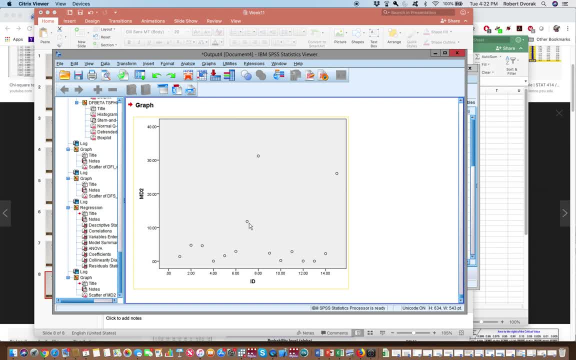 what looked to be like three potential- what looked to be like three potential- outliers on the hellenov assistance. it's outliers on the hellenov assistance. it's outliers on the hellenov assistance. it's questionable whether or not this is an questionable, whether or not this is an. 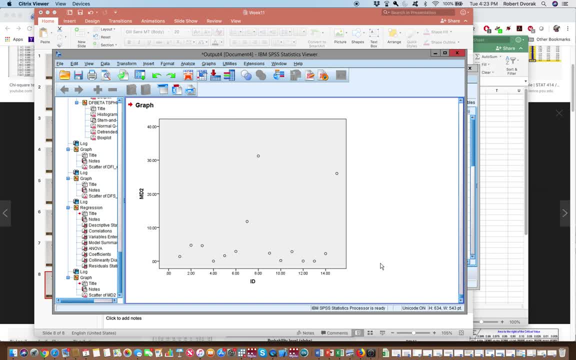 questionable whether or not this is an outlier, but we do know that we have two outlier. but we do know that we have two outlier, but we do know that we have two predictors in this model and an predictors in this model and an predictors in this model and an intercept, and so we have basically three. 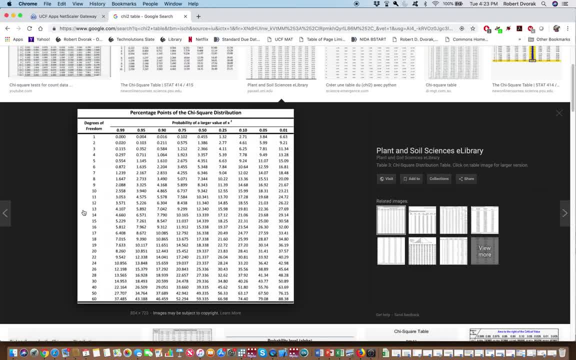 intercept, and so we have basically three intercept and so we have basically three degrees of freedom. so let's come over degrees of freedom. so let's come over degrees of freedom. so let's come over here and let's look at our chi-square here and let's look at our chi-square. 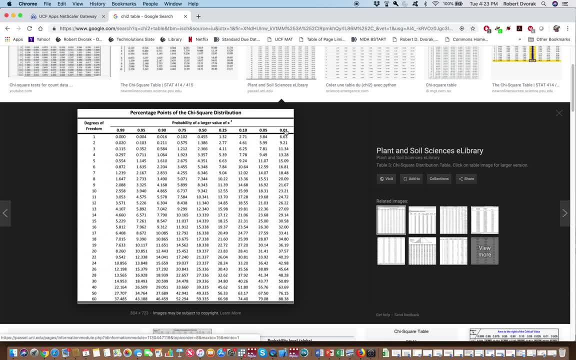 here and let's look at our chi-square table. you can use 0.05. I like to use table. you can use 0.05. I like to use table. you can use 0.05. I like to use 0.01 or even deeper than 0.01: 0.001 if. 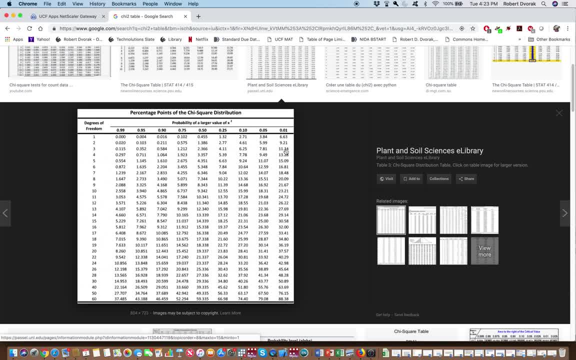 0.01 or even deeper than 0.01, 0.001 if 0.01 or even deeper than 0.01, 0.001 if you want, with three degrees of freedom, you want with three degrees of freedom, you want with three degrees of freedom at 0.01, 11.34 would be a significant. 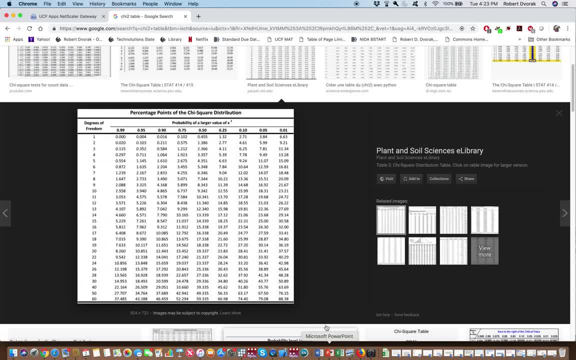 at 0.01, 11.34 would be a significant. at 0.01, 11.34 would be a significant outlier at two, you know point the 99th outlier at two. you know point the 99th outlier at two. you know, point the 99th percentile. so if we flip back to our 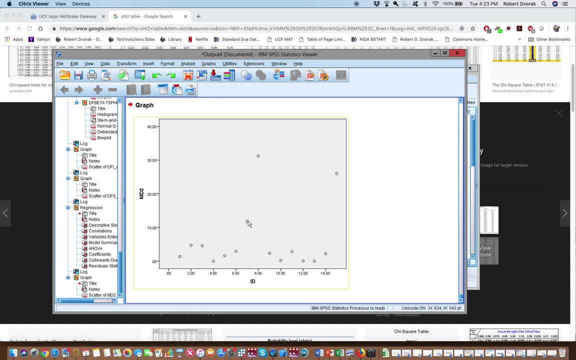 percentile. so if we flip back to our percentile, so if we flip back to our data, we have this value might be close data. we have this value might be close data. we have this value might be close. what did we say? it was 11.34. let's see. 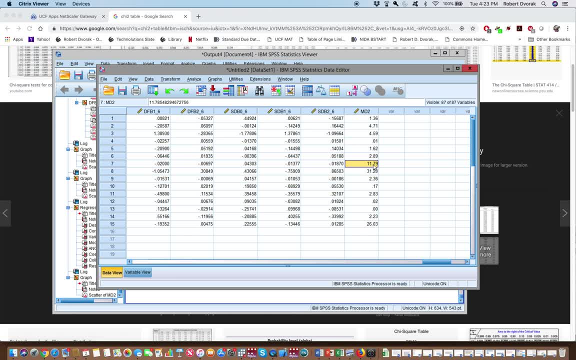 what did we say? it was 11.34. let's see what did we say? it was 11.34. let's see what we have here: oh, we have an 11.79. what we have here: oh, we have an 11.79. what we have here: oh, we have an 11.79. so this one right here might be a. 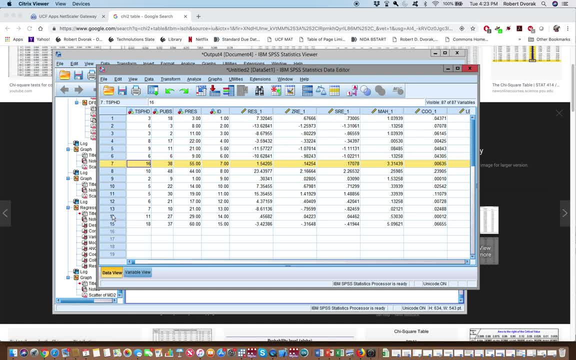 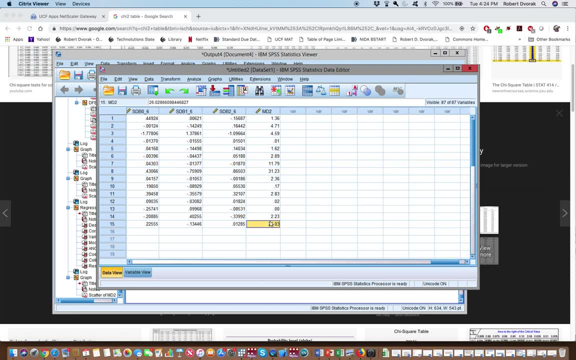 so this one right here might be a, so this one right here might be a problematic outcome. the other ones: 8- problematic outcome. the other ones: 8- problematic outcome. the other ones: 8 and 15- are almost certainly problematic and 15 are almost certainly problematic. 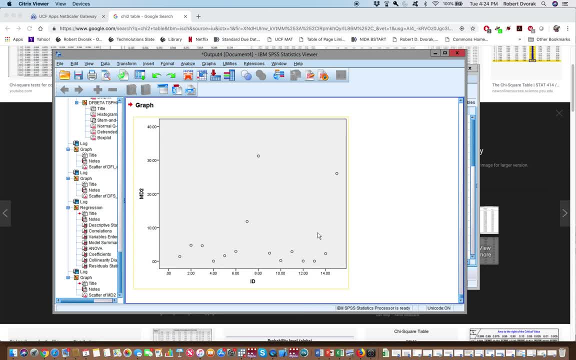 and 15 are almost certainly problematic outcomes, and that's these two guys right outcomes. and that's these two guys right outcomes. and that's these two guys right here, right, number 8 and number 15. and so here, right, number 8 and number 15, and so 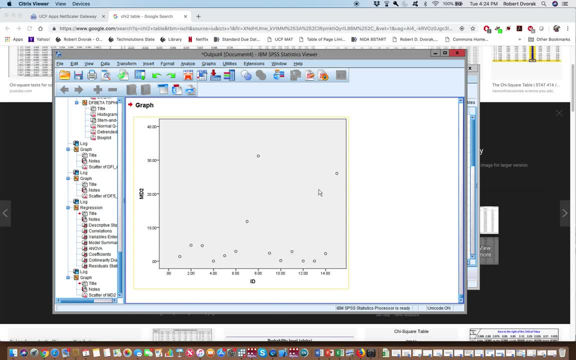 here right, number 8 and number 15, and so we could go and remove these two. we could go and remove these two. we could go and remove these two observations and remember this is on the observations and remember this is on the observations and remember this is on the regular data. I haven't transformed. 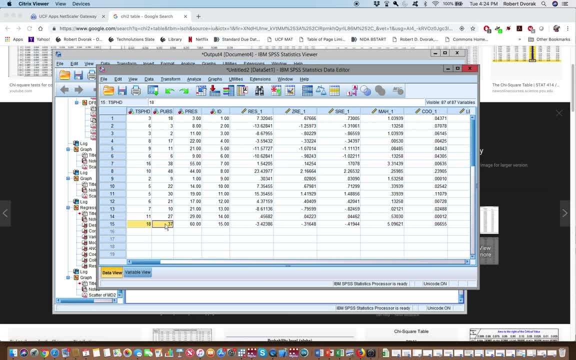 regular data. I haven't transformed regular data. I haven't transformed anything. I haven't changed anything I anything. I haven't changed anything, I anything. I haven't changed anything. I went back to 18 and 37 here, and so we went back to 18 and 37 here, and so we. 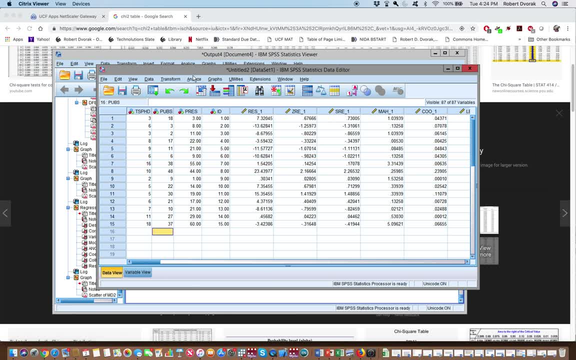 went back to 18 and 37 here, and so we do have these same two things that seemed. do have these same two things that seemed. do have these same two things that seemed like they were problematic. if we like they were problematic, if we like they were problematic. if we actually go and a lot, oh, we don't even. 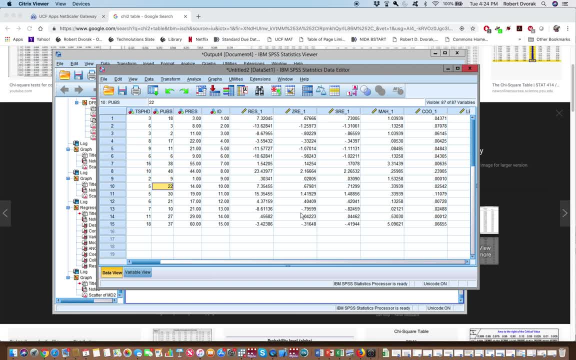 actually go and a lot, oh, we don't even actually go and a lot, oh, we don't even have to do it that way, we can just look. have to do it that way, we can just look, have to do it that way, we can just look at the Mahalan of assistance. if we only 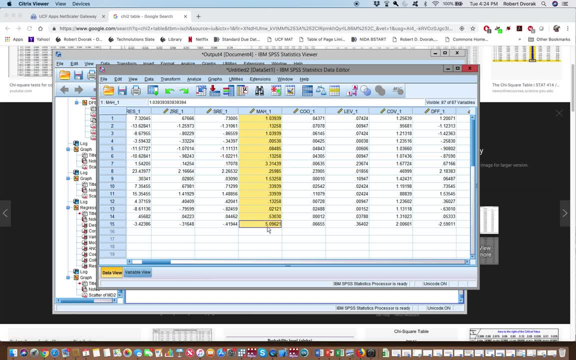 at the Mahalan of assistance, if we only at the Mahalan of assistance, if we only had one in right, if we were to square, had one in right, if we were to square had one in right, if we were to square this, that would be: it's gonna be 25 that. 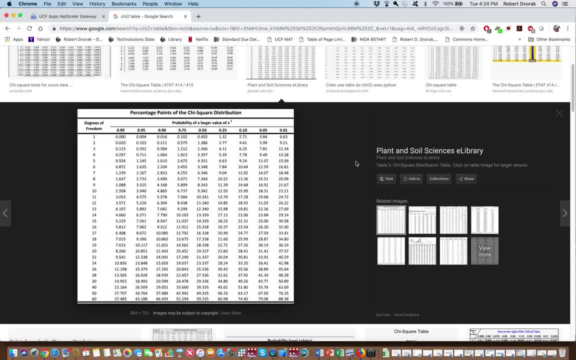 this, that would be, it's gonna be 25. that this, that would be, it's gonna be 25. that one's gonna be 9 and at 2 degrees of one's gonna be 9 and at 2 degrees of one's gonna be 9 and at 2 degrees of freedom. even here, 9 is gonna be close. 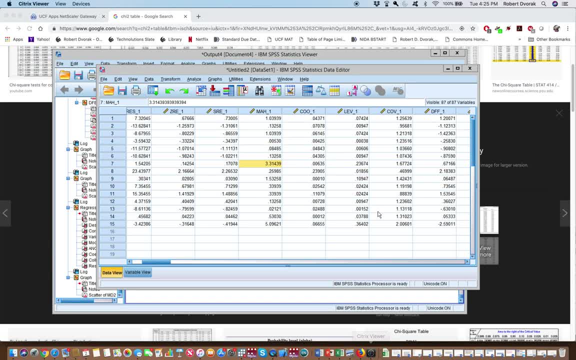 freedom: even here, 9 is gonna be close. freedom: even here, 9 is gonna be close. the other that number 15 observation. the other that number 15 observation. the other that number 15 observation. this one would be close. I'm assuming this one would be close. I'm assuming. 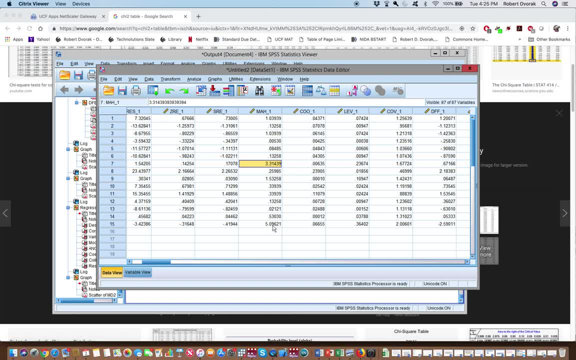 this one would be close. I'm assuming that we square these right. so this would that we square these right. so this would that we square these right. so this would be around 10, I guess, and this would be be around 10, I guess, and this would be. 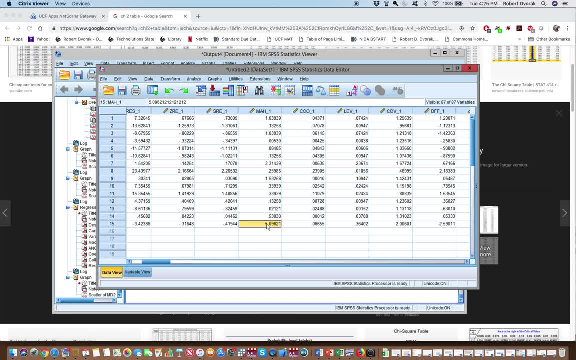 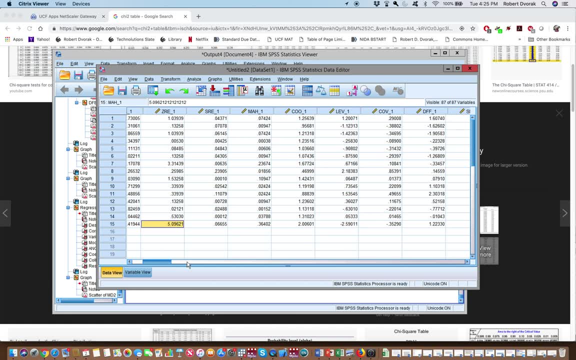 be around 10, I guess, and this would be 25. this is a definite outlier right. no 25. this is a definite outlier right, no 25. this is a definite outlier right, no matter what we do. whether it's a matter what we do, whether it's a. 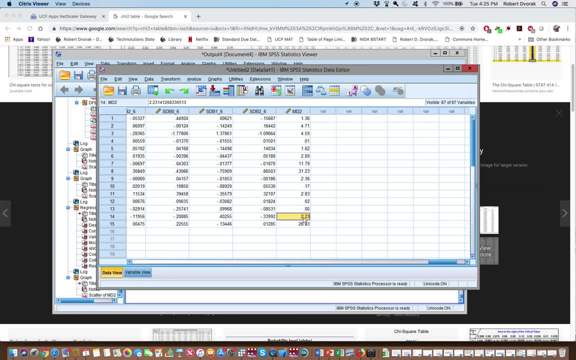 matter what we do, whether it's a another predictor in here, makes this a another predictor in here, makes this a another predictor in here. makes this a much. actually makes this one a much much. actually makes this one a much. much. actually makes this one a much worse outlier. this one doesn't. doesn't. worse outlier: this one doesn't doesn't. worse outlier: this one doesn't. doesn't change all that much at all. let's look, change all that much at all. let's look, change all that much at all. let's look at the difference between these two, at the difference between these two. 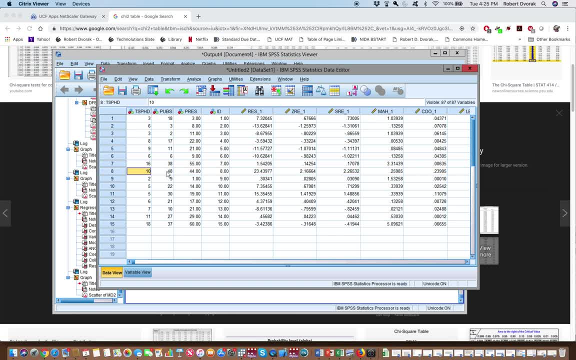 at the difference between these two: between 8 and 15 over here. oh yes, so 10. between 8 and 15 over here. oh yes, so 10. between 8 and 15 over here. oh yes, so 10, 48, 44. those look like outliers you have. 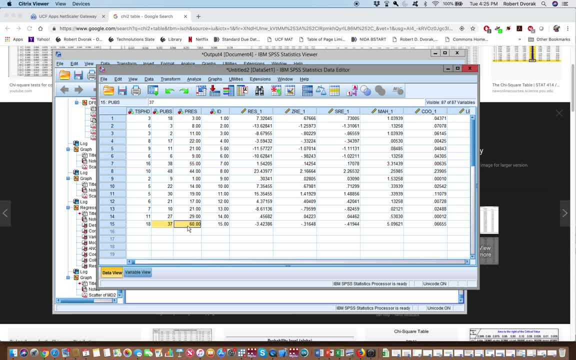 48, 44. those look like outliers. you have 48- 44. those look like outliers. you have 1837 and 60. so you can see that this one 1837 and 60. so you can see that this one 1837 and 60. so you can see that this one winds up being a bit more problematic. 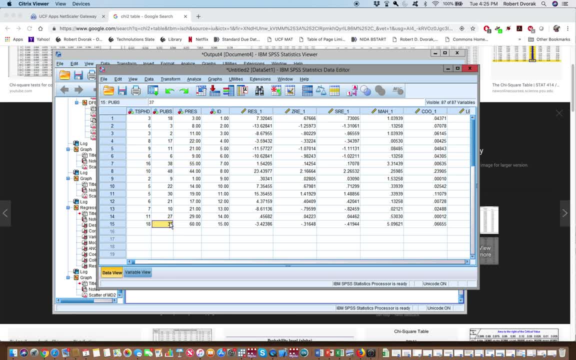 winds up being a bit more problematic. winds up being a bit more problematic, probably because of this item. it's way, probably because of this item, it's way. probably because of this item it's way higher here and that would be my guess. higher here, and that would be my guess. 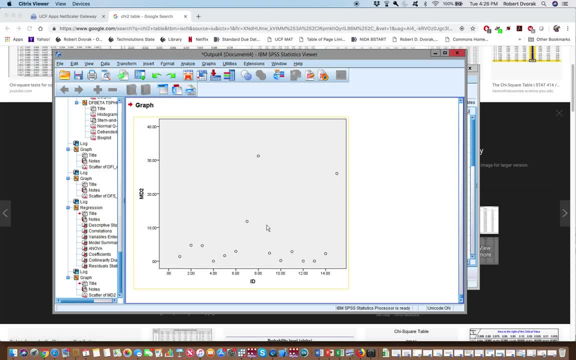 higher here, and that would be my guess. but anyway, in this case I would say we. but anyway, in this case I would say we, but anyway, in this case I would say we have these two oddballs, they are they. have these two oddballs, they are they. 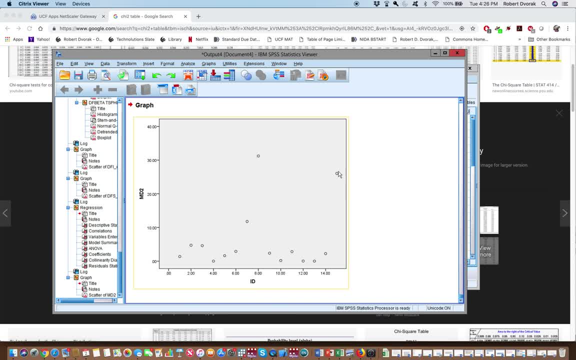 have these two oddballs? they are. they were both univariate outliers. this one were both univariate outliers. this one were both univariate outliers, this one more so than this one when we looked at more so than this one when we looked at more so than this one when we looked at univariate effects. however, this one as 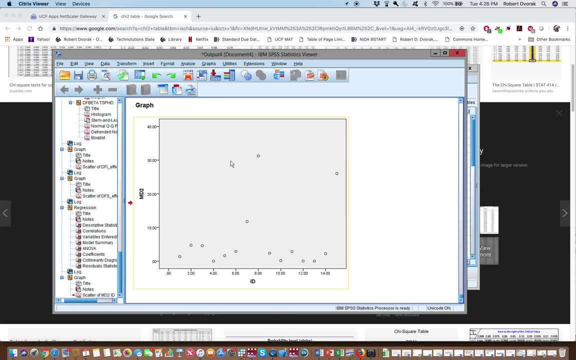 univariate effects. however, this one as univariate effects. however, this one as stronger multivariate outlier effects, stronger multivariate outlier effects, stronger multivariate outlier effects based on the Helen of assistance, and I based on the Helen of assistance and I based on the Helen of assistance and I would say that you have good evidence to 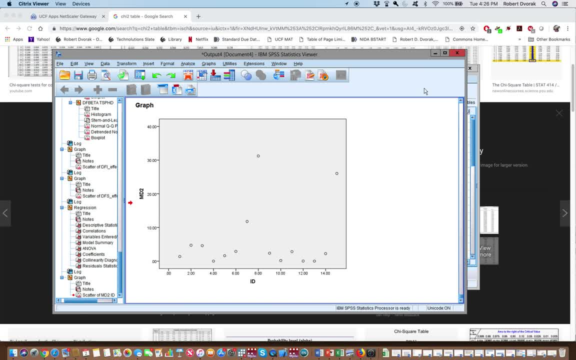 would say that you have good evidence to would say that you have good evidence to drop both of those variables or both of drop both of those variables or both of drop both of those variables or both of those observations and then rerun it- those observations, and then rerun it. 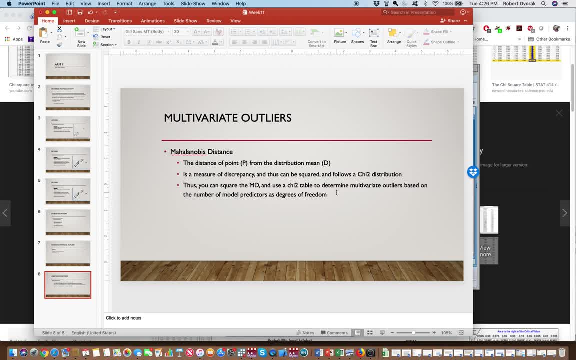 those observations and then rerun it from there, rerun your analysis from from there, rerun your analysis from there. so, all right guys, that is it that there. so all right guys, that is it that there. so all right guys, that is it. that is multivariate and univariate outlier.